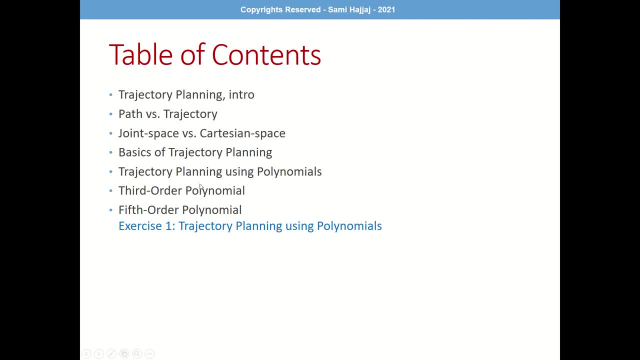 then we're going to talk about trajectory planning using polynomials and how or why they are useful for us. and if this sounds familiar, if you're coming from the mechanical engineering courses, and if this sounds familiar to you, then good, because whatever you're thinking about, it's. 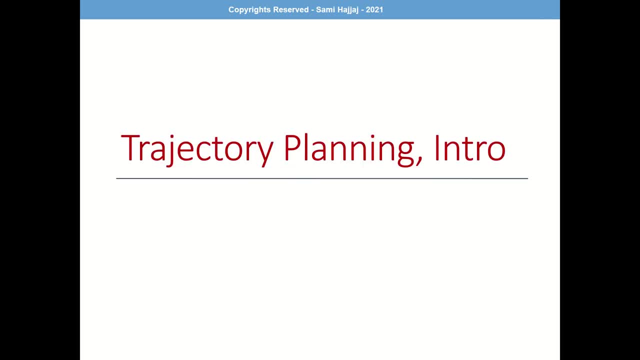 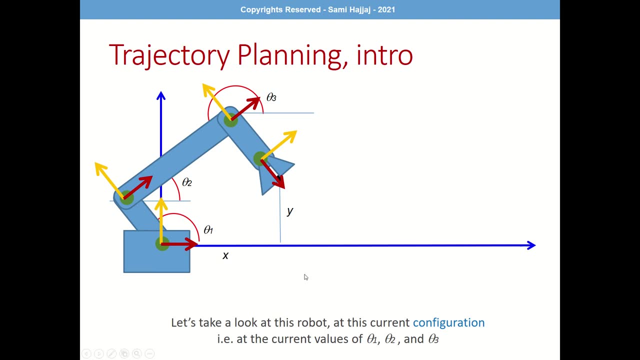 correct, but we'll get to that in a minute. So a little bit of introduction. what is trajectory planning? So okay, so let's take a look at this robot right here, at its current configuration. When we see the current shape of this robot, or the way that it looks like right now, 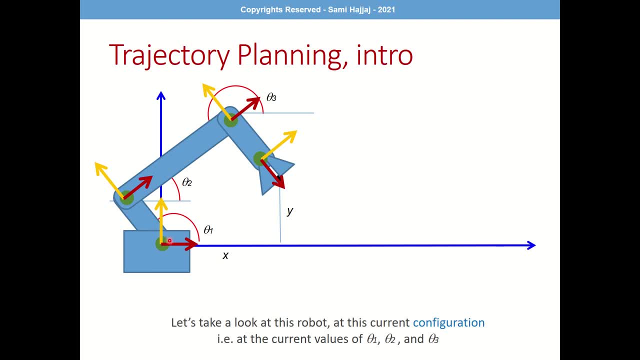 we call it a robot configuration. So at this configuration, aka at this exact values of theta one and theta two and theta three. so we call this this current configuration. Now, here is the same robot but at a different configuration, and this is important. you see that now the the shape of the robot is different. Its reach, the orientation. 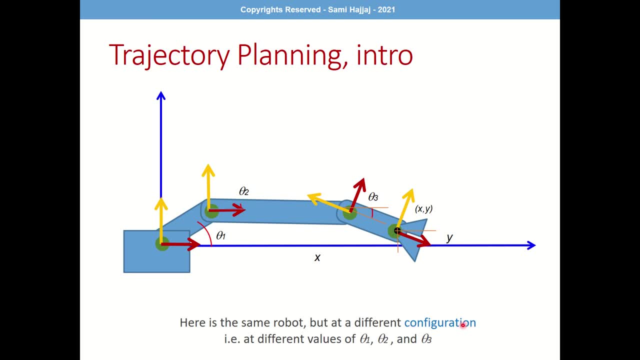 of the end defector is totally different, and that's what we refer by configuration. See, this is one configuration and this is a second configuration. So trajectory planning is about how does the robot travel from one configuration to the other. We can do forward kinematics here. 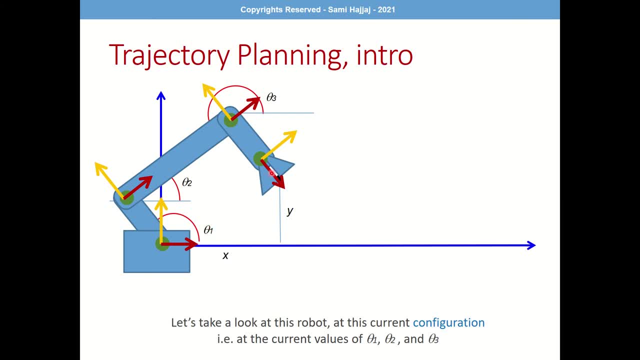 like: okay, if I give you the values of theta one, theta two and theta three, then what will be the corresponding pose of the end defector? or I could, we could do inverse kinematics here. we can. basically, if I give you the pose of the end effector, then you would need to find out the 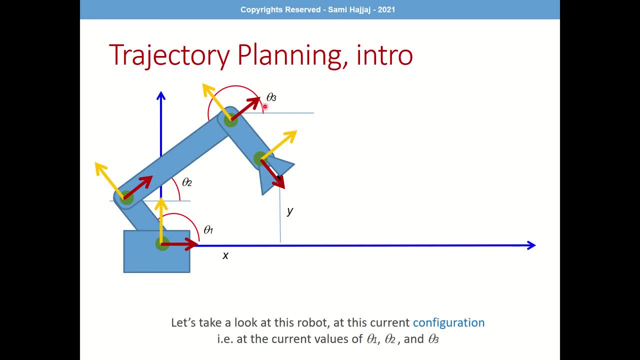 corresponding values of theta one and theta two and theta three. all right, no problem, We can do the same things here. you know we can do forward and inverse kinematics again on this configuration. but the trick is, or the situation now is, what happens in between, when the robot travels between the two configurations? How does the robot actually change? 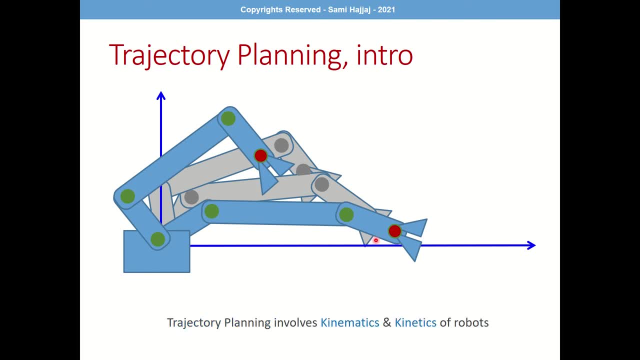 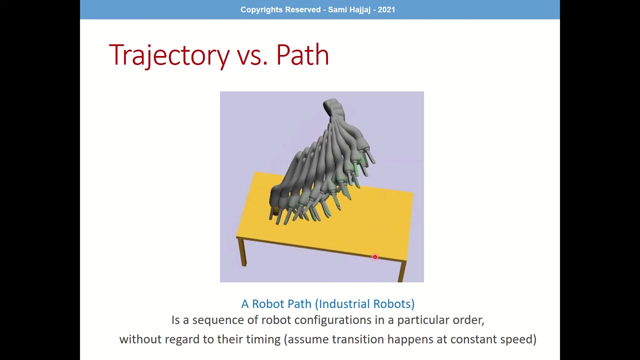 or travel. So this is the study of inverse kinematics. oh, excuse me, this is the study of trajectory planning. It involves kinematics as well as kinetics. Kinematics basically means position and orientation and acceleration- excuse me- position, velocity and acceleration. but kinetics will also involve dynamics or forces and torques. So let's more a little. 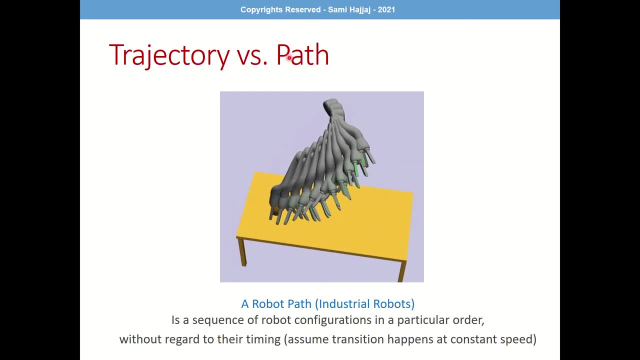 bit of more of definition. So a trajectory versus a path. what is the difference between these two words? They might appear similar to them in a regular layman language, but in, specifically in industrial robots, they actually mean different. they have a different meaning. So let's talk about what is a path? The word, the English word path, might have a different 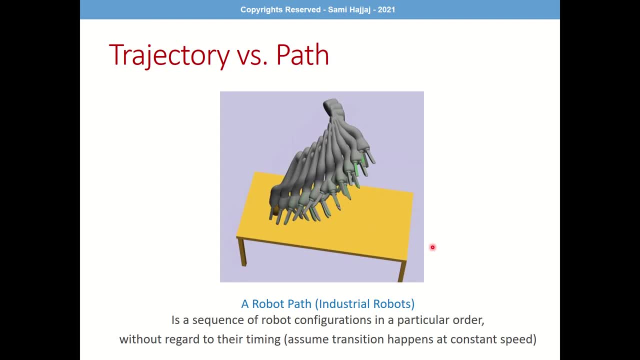 meaning to you right now. so I want you to put that aside and focus on this particular definition of a robot path and for industrial robots. So a robot path, when it comes to industrial robots, is a sequence of robot configurations, as you can see from here. So this is one configuration. 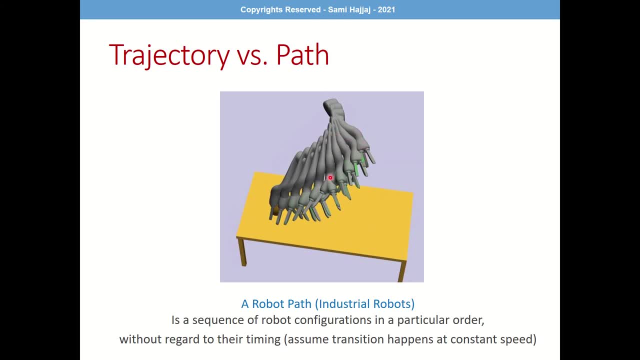 this is another configuration and there's another configuration, So a sequence of all of these configurations are all considered. this is all basically considered a robot path and they are in particular order, so you don't jump from this configuration to this one and this one. they are. 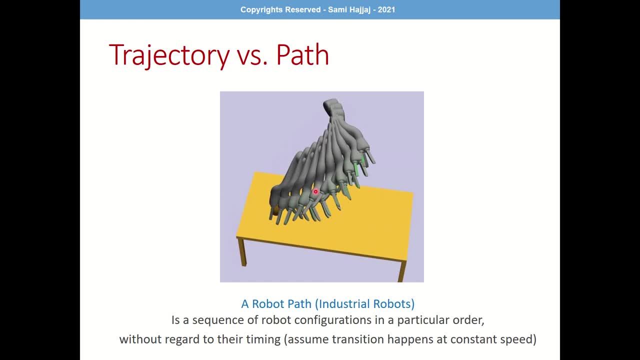 actually given in this correct order, and but we ignore the timing of this configuration. Basically, what does that mean? You can say that of time, to go from this configuration to this configuration could be one second, but to go from the second to the third configuration, this might be three seconds, and so on and so forth, and so we 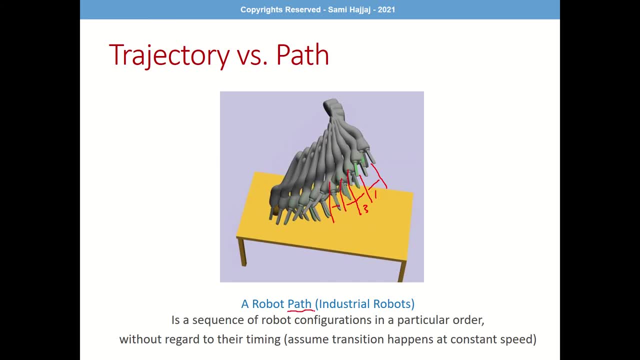 actually don't care when we are, we're talking about robot path. we do not care about timing, we ignore it, you know. so basically, we're going to assume that all the transitions happen at constant speeds, in other words, when you transfer or you transition from one configuration to the other. 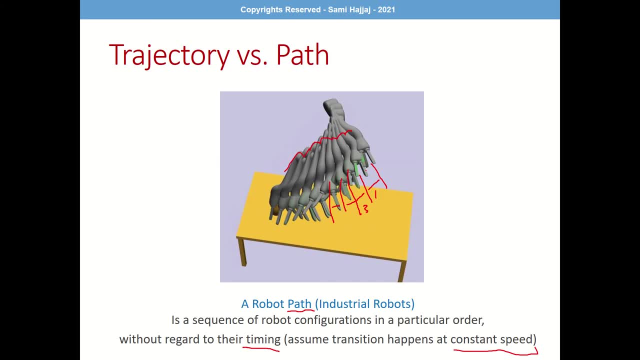 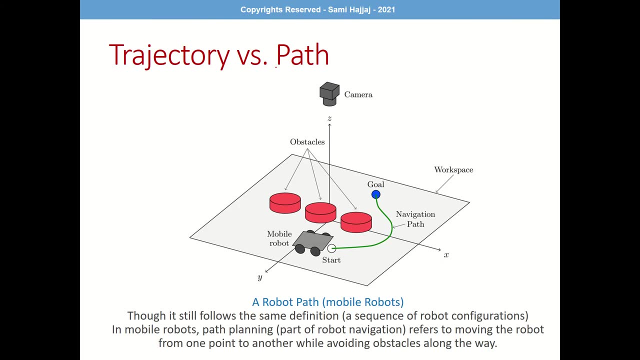 like this. the duration in between is constant, or at least we don't care about it. now the word robot path might seem, or even in the word path in general, right might actually mean something else to you, and this has to do with you know, when you're driving a car, or even in robot, in mobile. 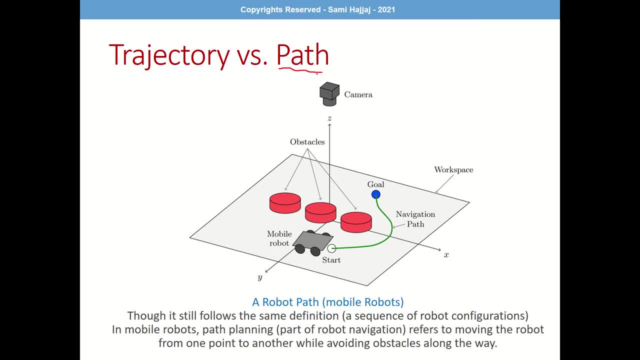 robotics, a robot path obviously is the, you know the, the journey or the line that defines the actual movement steps from one point to another. so you can see that this green part, this green line right here is obviously is the navigation path of this robot. so this is the word path in mobile robotics. but 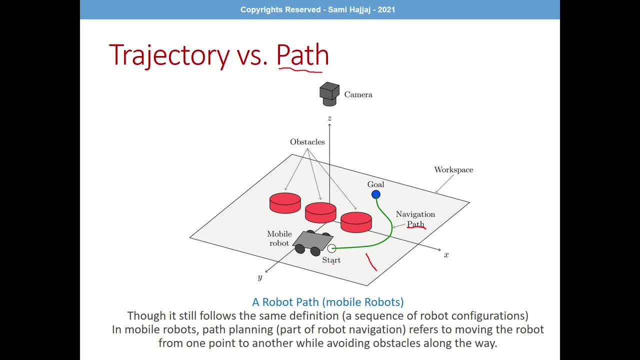 believe it or not, this path is also defined using exactly the same definition that we said earlier. it's a sequence of robot configuration. so this is one configuration. here is another configuration, which is right here, and here's another configuration. so, once again, a sequence of configuration, now in this configuration. 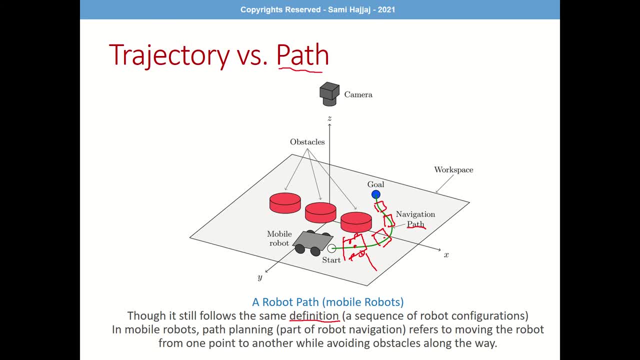 the robot position and orientation changes. see, this is the position and this is the orientation position, orientation, position, orientation and so on. so in all it, although it looks different, but it's actually is exactly the same, meaning a robot path, whether it's mobile robot or industrial robot. 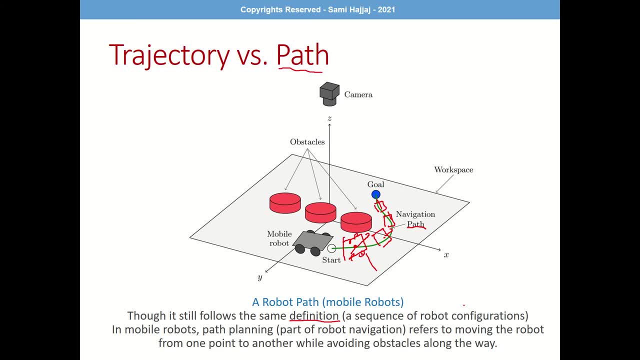 is a sequence of robot configurations, or aka, changes in position, on orientation or, you know, robot parameters along the path. of course, in mobile robotics this means traveling along the path, which is part of the robot navigation package, avoiding obstacles, going from a to b, etc. so we're 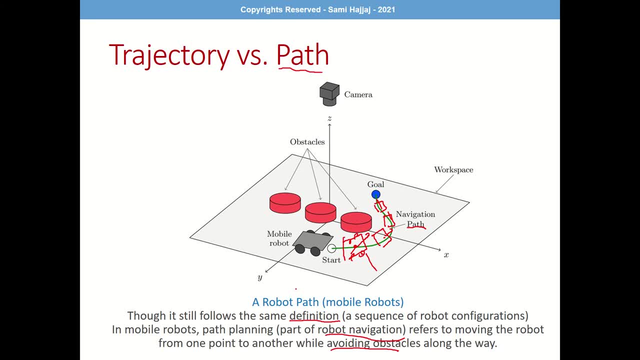 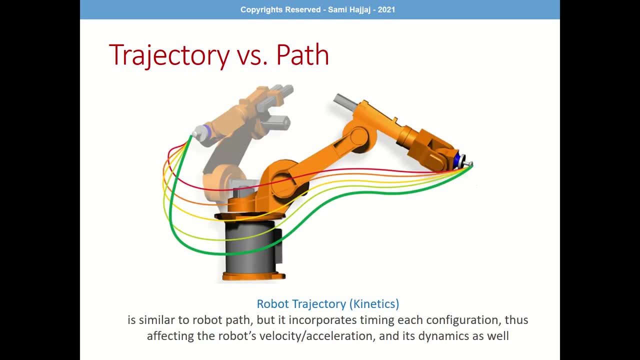 going to focus on. we're going to ignore for a second the mobile robotics definitions. we're going to focus on industrial robots, because this is our course- focuses entirely on industrial robots. so now let's talk about the robot trajectory. just now we discussed the path, but now let's talk about trajectory. a trajectory is a very similar to robot path. 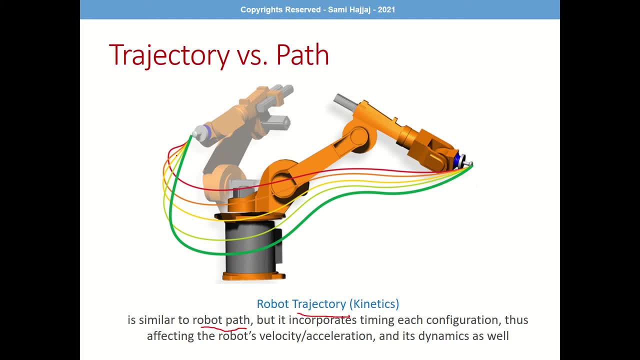 it's exactly the same, meaning it's a sequence of configuration that are actually changing. however, we in. we now incorporate the timing. we must incorporate the timing, otherwise we're going to have problems. so therefore, the robot's velocity and acceleration, as well as dynamics, are all incorporated. meaning: incorporate means that we put into consideration. we will study the effects. 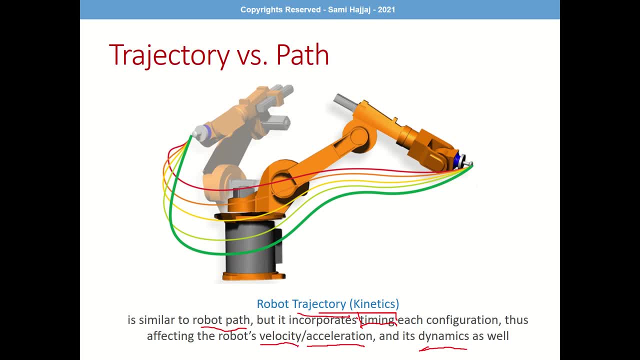 and therefore we will have a note in mind what happened to robot kinematics, what happened to robot dynamics as it moves from one configuration to another. so, essentially, a trajectory is a robot path plus timing. so you can simply say, if you want, you can just down here and say: trajectory is equal. 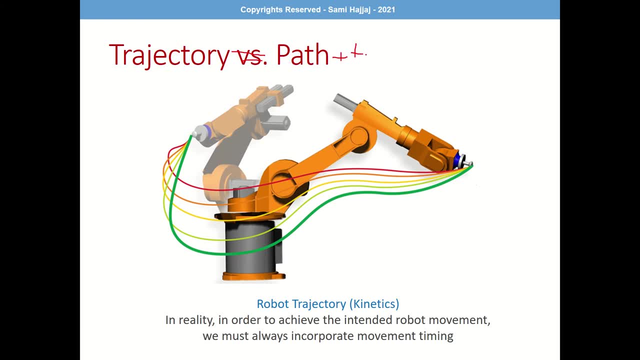 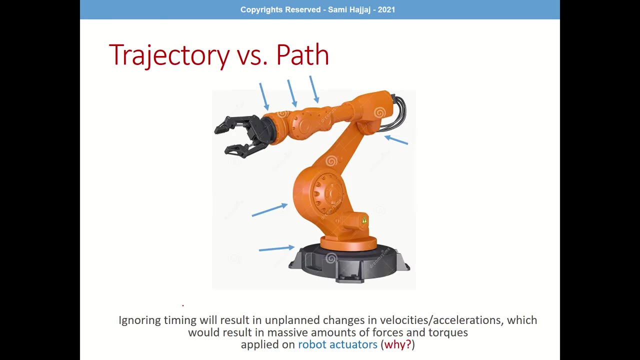 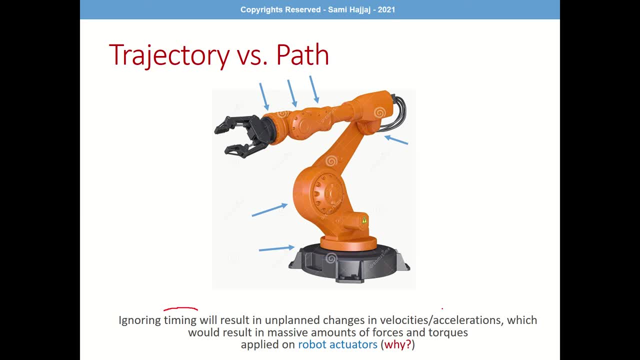 unplanned changes in velocity and acceleration, and this is actually the key one right here. if you remember, in theory of machine we we've seen something like this as well. if you have unplanned changes in velocities and acceleration, then you will have cons on um, you know. 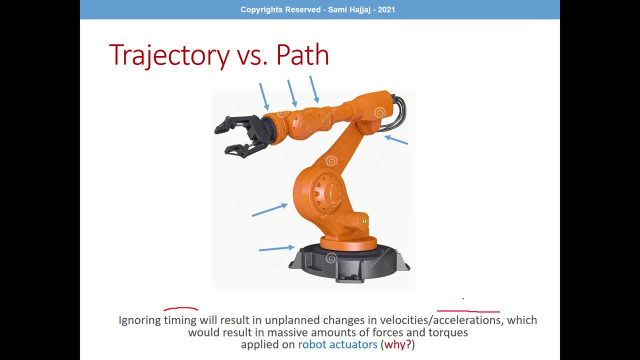 you have terrible consequences if you end up with very high values of acceleration. you know what? i'll give you a moment to think about this. what happens if you get acceleration- uh, you know whether it's a acceleration or alpha for angular- which is very, very high. what's the big deal and what about? 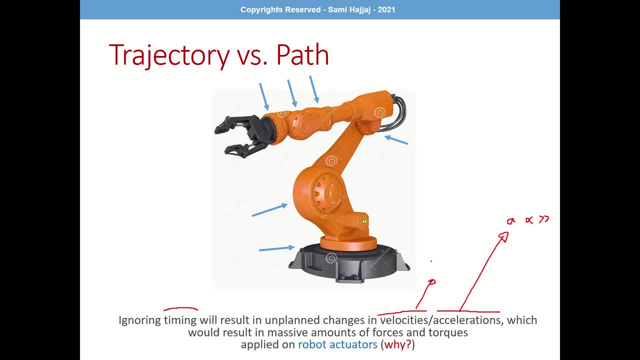 velocities, if velocities itself is also very high. so if v for linear, or omega for angular, if that one is also very high, what's the big deal? think about it for a minute and then, um, you can pause if you want. think about it for a minute and come back to this video. okay, so i hope you have figured it out. 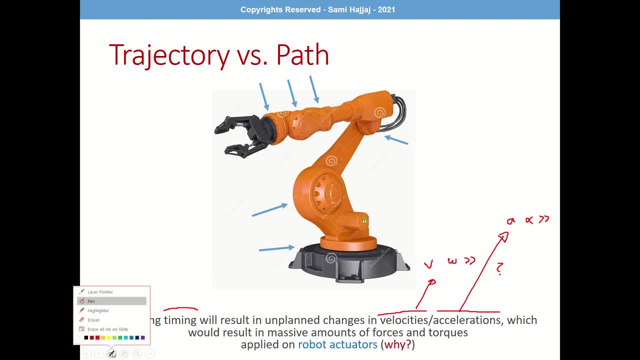 this one might be a little bit easier to to realize- which is the effect of the acceleration. obviously the acceleration have a direct effect, which is force is equal to m, which is the mass multiplied by acceleration. so if you have a high acceleration multiplied by the object's mass, you will end up with very high forces. the same thing applies for angular. if you 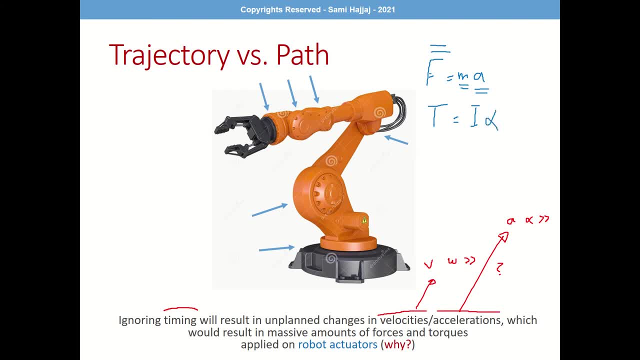 have a torque is simply equal to the inertia multiplied by the angular acceleration. so the angular acceleration, if it's too high you will end up with very high torque. and if you have very high torques then those torques will be applied on the motors, so those motors moving 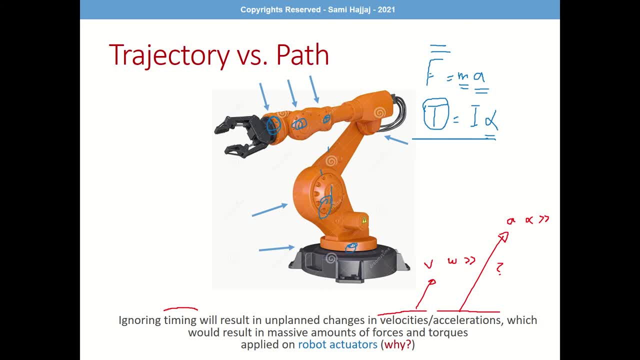 the robot into this or these joints right here, they will have to apply extremely high torques that could result in in damaging the motors or the actuators. So if you are not careful, you would end up applying amounts of torques and forces that are beyond the capacity of the actuators. 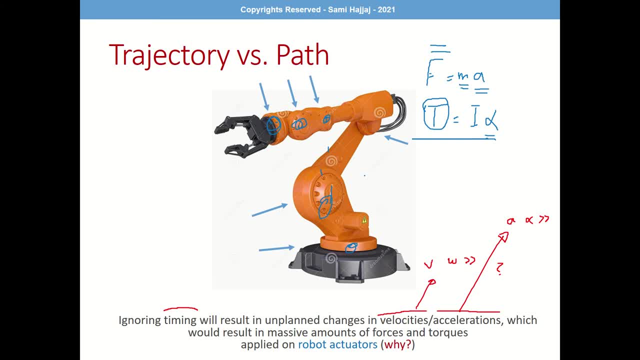 Or you would require then, in this case, very high amount of torques, which would require a huge amount of motors, which will become very difficult to work with. So, whatever it is, you will always want to end up, you will always want to reduce the amount of accelerations. 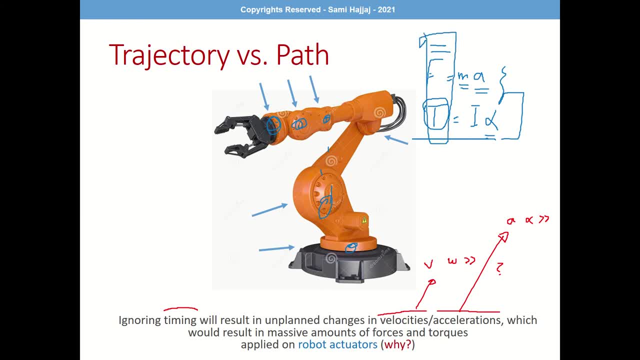 in order, or at least control it within the limits of the actuators capabilities. Okay, that was the acceleration, but what about the velocities? Well, velocities, if you remember, are involved directly in kinetic energy. So, Ke kinetic energy is simply equal to half of MV square. 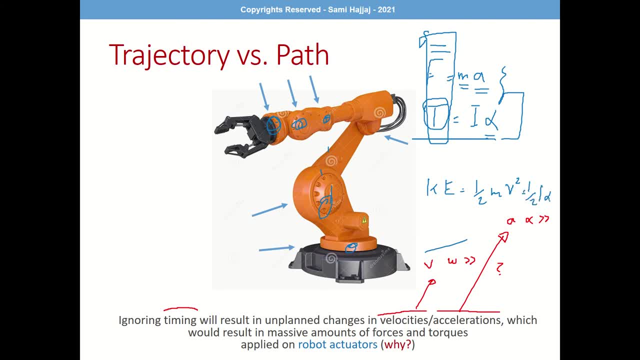 also equal to half of I alpha square, which is the inertia, and alpha, which is: this is the linear and kinetic and this is the angular kinetic. So once again, sorry, not alpha, omega. So let me just clarify. So this is omega square. 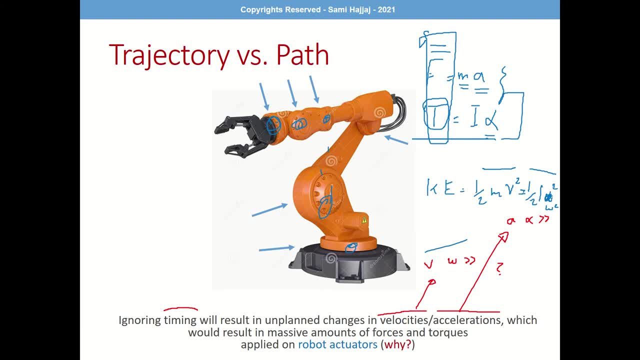 Not a alpha square. So, even though we are not talking about acceleration, we only talk about velocities, you could end up with a very high kinetic energy And again, if the kinetic energy is too high, then we are talking about consumptions of power. 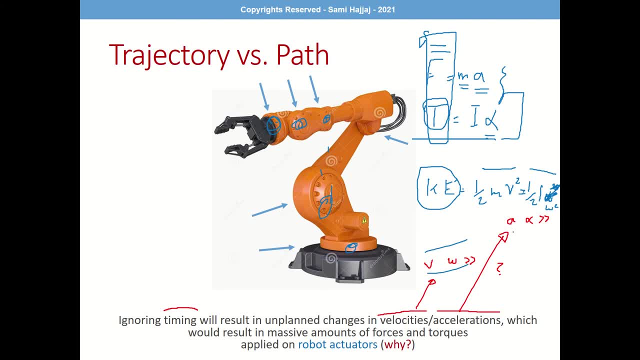 You know, even though let's say that we ended up with a, even though we had an acceleration that is within the capacity of the motor, the actuator, okay, no problem here, but then we still end up with unnecessarily high amounts of velocities. you can end up with kinetic energy, and kinetic energy, or energy in general, are directly. 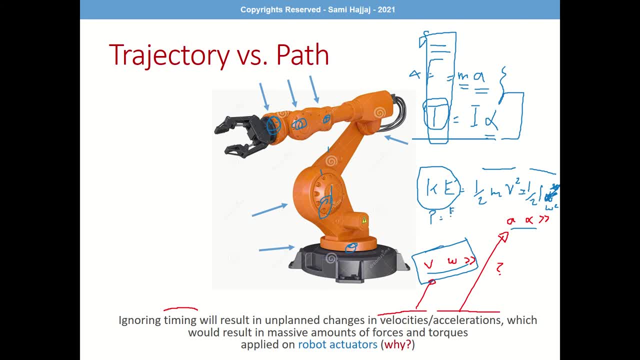 connected to the power, which is energy divided by time, and therefore that could actually result in amount of power required to move the robot, so you could end up with unnecessary amount of power consumptions or amount of power required to move the robot, which again power is translated to costs. 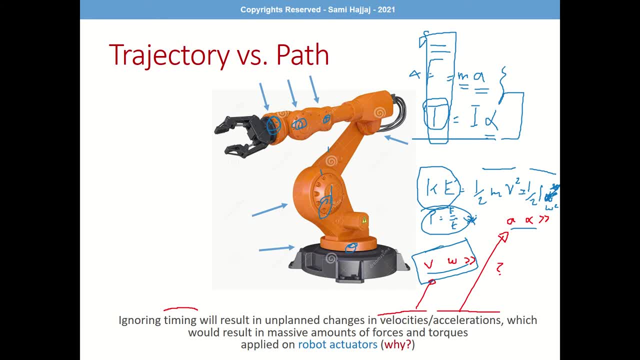 which again cause could result in unnecessarily powers or unnecessary power costs involved in robot operations. so if you're having an industrial robot doing machining or, let's say, welding, but you're overusing the amount of power- electrical power- to run the robot, then a lot of the overhead. 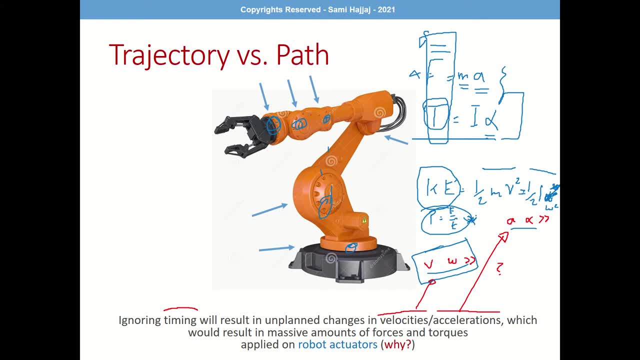 costs will go to just moving the robot. that will actually increase the cost of the product, will minimize your profit margin and cause other problems. so you would always want to minimize these two together as much as possible, lower the velocities as much as possible and, of course, lower the acceleration. so that is why this. 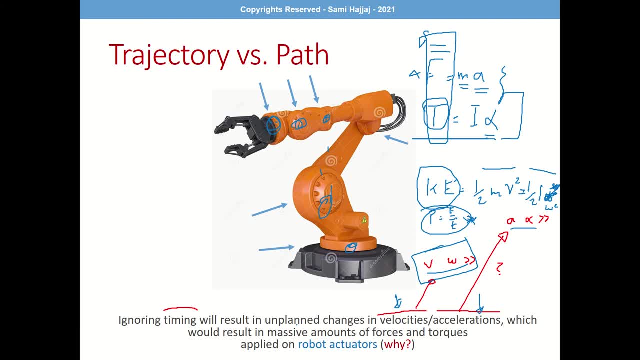 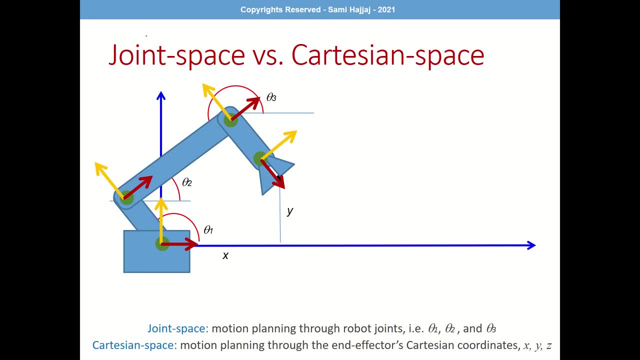 is the importance of trajectory planning, or and so on. okay, all right, we get that. what's next? so now let's just define one more definition, which is joint space and cartesian space, and this terminology is used in many robotics books. i would like you to take a look at this, and 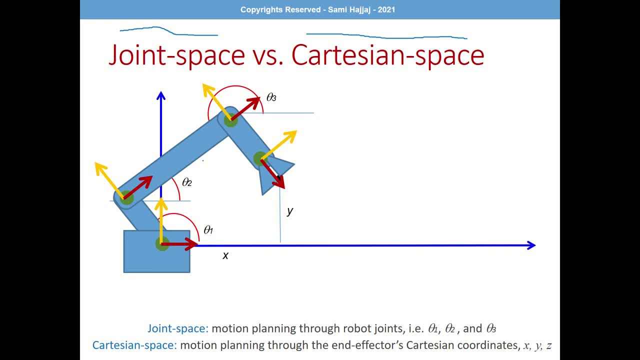 familiarize yourself with it. you are already familiar with this concept. i just want you to be familiarized with the name of it. so what is joint space? joint space, joint space trajectory or cartesian space trajectory trajectory. these are two different types or two different ways of doing. 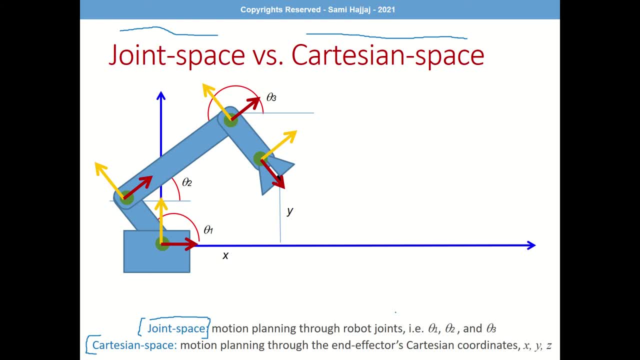 trajectory. one of them by focusing only on the joint values, in other words, by focusing on the robot values and therefore controlling, in this case, in this particular robot, theta one, theta two, theta three- if you want, you can just simply call it theta i. so essentially, uh, in joint space motion planning, we essentially do the motion planning through the. 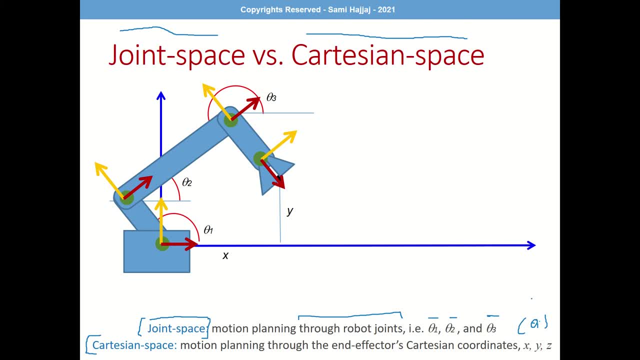 robot joints, and that would be theta i. of course we would have li if we had linear, actuate linear joints as well. so theta i and li. now cartesian space motion planning is that doing the same thing but through the n defectors, cartesian coordinates. so this is basically xyz, if you. 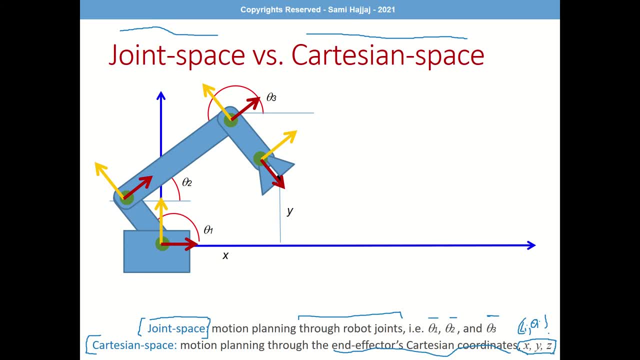 only care about position, but if you want to include the orientation, then you have to put noa as well. now- uh, you might think, wait a minute. this looks very much like forward kinematics, and you were right. so this is very much similar to working with forward kinematics, while this part right here. 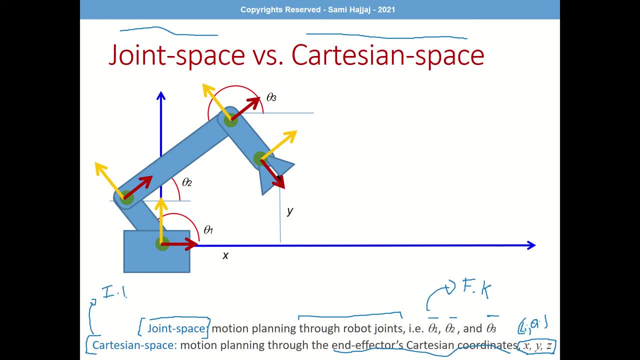 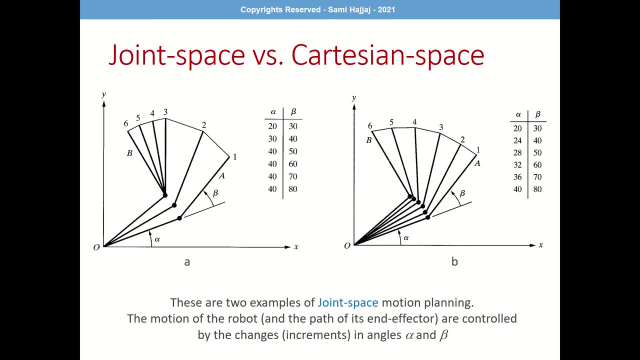 is very much similar to work with inverse kinematics. uh, however you like to call it, it's fine, as long as you understand the meaning of the terminology. okay, let's move on. so here's an example of- oh, actually, two examples of- joint space motion planning. what is that meaning? what does that mean? 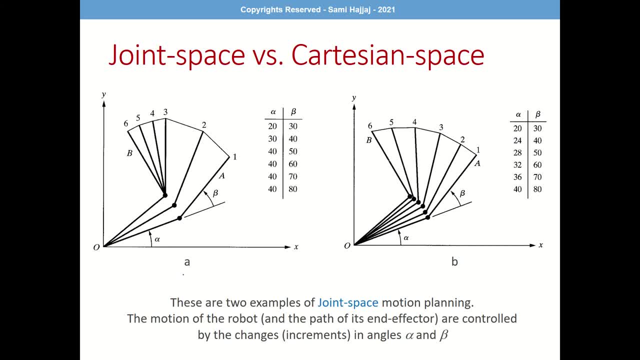 you see, in this particular example, or in this example right here, example a, we have decided to move the robot uh by changing the values of alpha and beta, alpha meaning this the first joint angle and beta is the second joint angle through the values. you see in the table right here. what was? 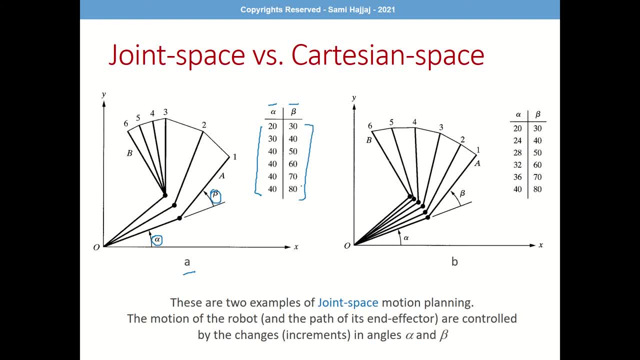 the reason behind it? what was the logic? don't ask. just basically, it was decided that we're going to follow this path, this pattern, and, as you can see, joint alpha changes in the beginning from 20 to 30 and then stays at 40. it doesn't move any forward. you can see that it's moving in the right direction. 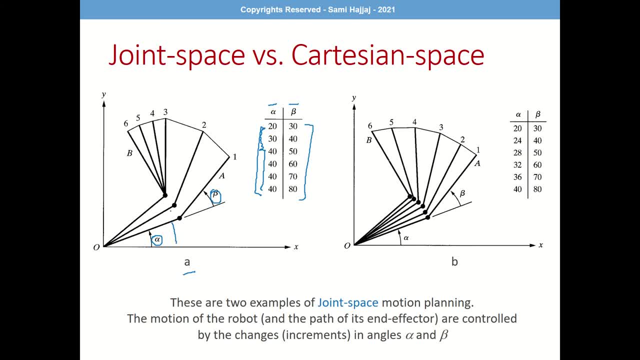 you can actually see that effect here. so this is basically 20, uh sorry, 20 and 10. this is the initial value. so this is 20 degrees, 10 degrees, and then from then on, zero. so nothing happened from there, okay, or maybe you can say that: from here, zero. this is now 20, uh, 10 degrees, and then another. 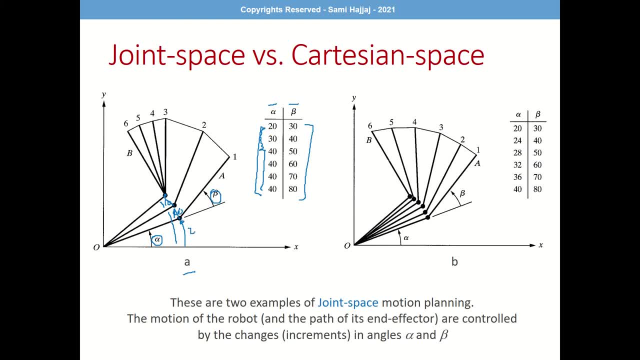 10 degrees. yeah, this is. this is basically what happened. so this is now 20 because it was zero. then goes to 20, so that's what happened here. then from 20 to 30, that means it changes by 10, so that's at 10 degrees. and then from 20 to 40, another change by 10, that's another 10 degrees. 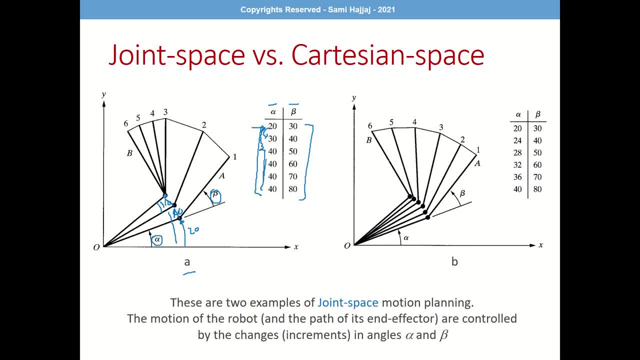 here. then, as you can see from the rest, there is no changes. so that link doesn't move any forward. now, looking at angle beta, as you can see that it starts at 30.. so, right here, this is the beginning. this is 30, and then, from here on now, the change is: now it's 10 degrees. here, another 10 degree. 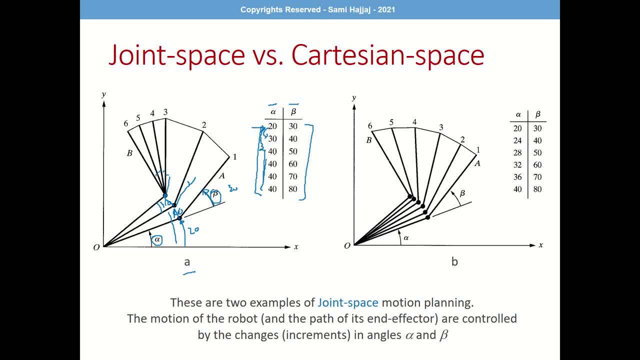 basically, it's always going to be 10 degrees as you go along. you got me, so that's essentially what in the first particular case. in the second particular case, the situation is slightly different and we decided to make the, the changes slightly more uniform, meaning that from here is: 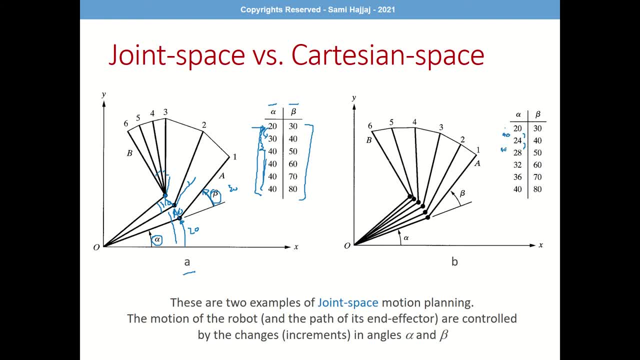 always four degrees different. so this is 40, 40, sorry, four, not four degrees. four, four, four, and so on, until we get to here. yeah, if you notice that the starting angle is 20 and the ending angle is 40 here, but we also get the same thing here. so this is also 20 and this is also 40. right, but then 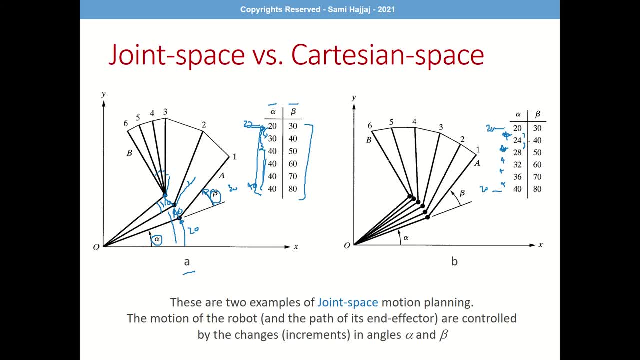 you change from from through the, from the beginning until the end. the same thing here. this is also 30 and we end up with 80, just like the beginning. there the case, and i think this is exactly the same. yeah, this particular beta angle and the transition from, from the starting point to the. 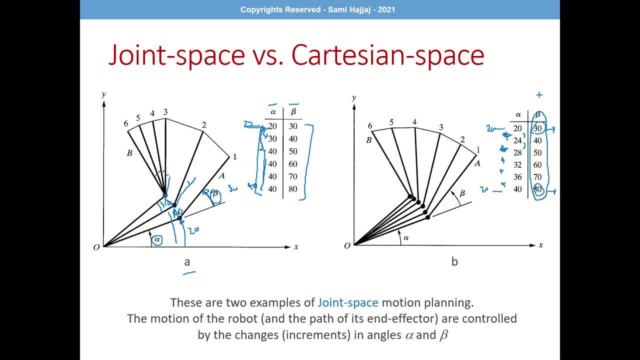 end point does not change. basically, here we decided to increment by 10, and here we decided to increment by four, but over here it's also plus 10, but over here the increment is not fixed. it's not fixed. we go 10, 10 and then we stop. i mean so zero until n. so this is how we actually um. 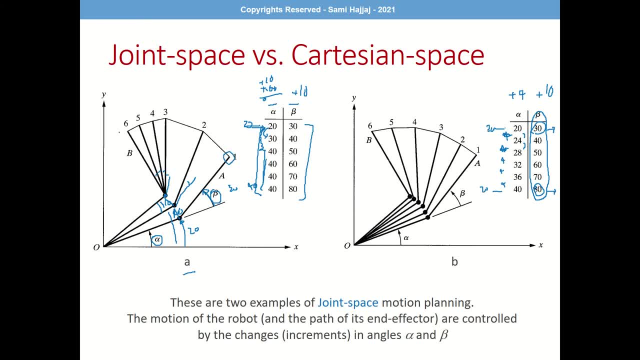 in other words, in both of the cases of these two robots, we have position a and position b, but we can see that the the resulting path of the robot, the resulting the way that the robot traveled, is different, because we have controlled the angles, we have incremented the angles different. 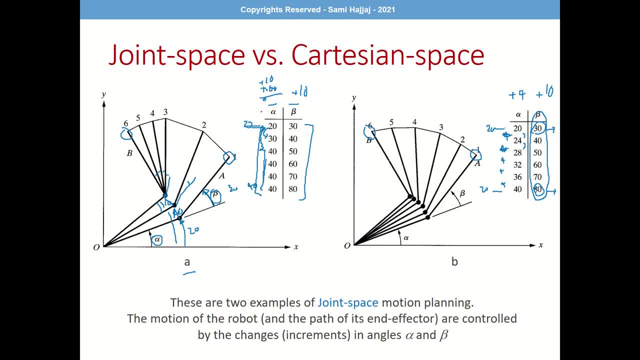 see here, when we incremented the robot, when we incremented the angles in this particular pattern right, you can see that the resulting travel or the resulting robot path is, basically, is this path right here and, as you can see, this, by the way, is not a straight line. it's a little bit of curve, as you can see. that is different. 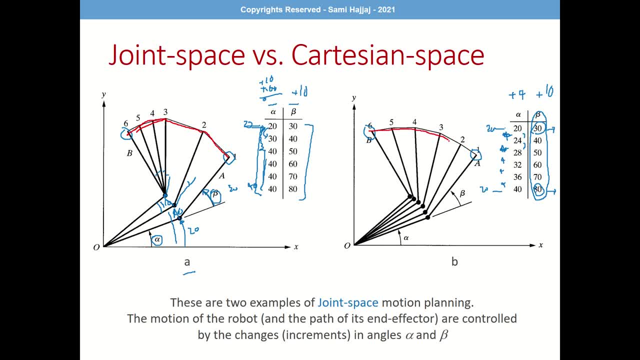 from this path right here, which looks like a little bit more uniform. okay, so once again, that this is how or this is what happens when you work with joint space, when you control or when you change the path of the robot or the the way the robot travels from beginning until end, by simply controlling the joint angles. okay, 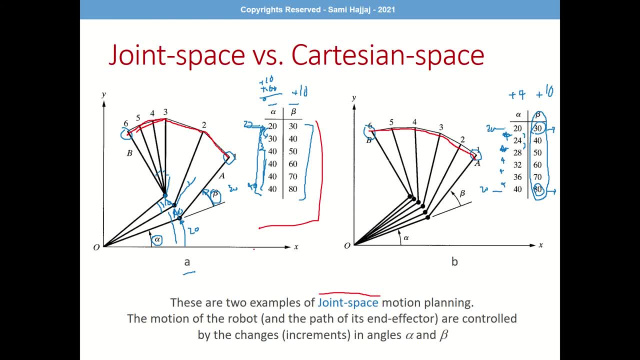 now, as you can see, no matter what you do in case one or case a or case b, the the resulting path will always be a chopped path, being basically a series of straight lines and, uh also, uh, an increments of straight lines between a and b. i think that's mentioned. yeah, the next line. 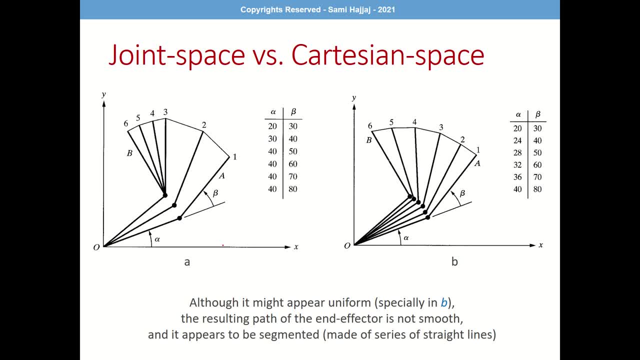 as you can see, right it, although it might appear a bit more uniform, especially in, in this case, case number b, right the, the part of the nd vector is, as you can see, is not straight. it's not straight line. it's basically a series of straight lines, chopped, as you can see from here, although this 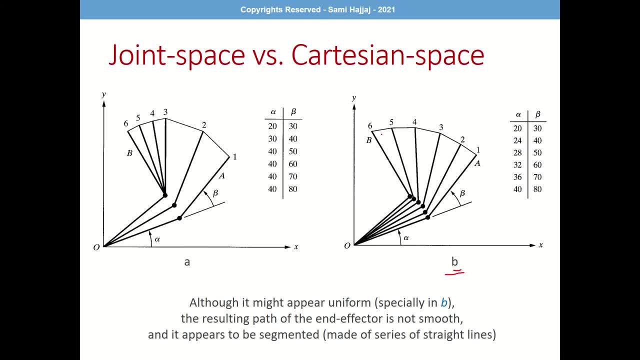 looks a little bit more curvier, but more, maybe more uniform, but this is still a series of straight lines and like it appears to be segmented and the changes of the angle is actually it's also happening. uh, this could be enough for you, this could be sufficient, but at some point you would. 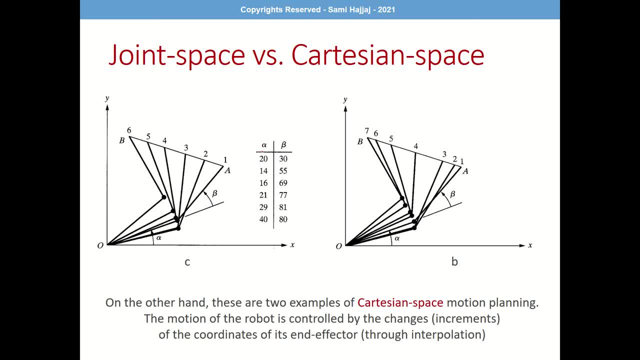 see that this is not enough. now, this is an example of, or two other examples of, cartesian space, meaning we decide the way that the robot moves based on the coordinates of the nd vector. that's how we did it. we did not uh care about the angles, we simply started from the position. 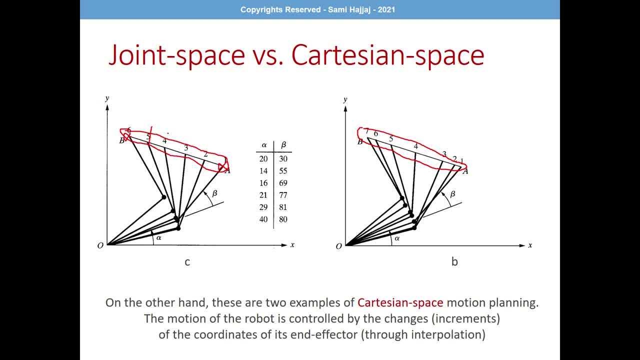 of the beginning until the end. and then we decide we break the path into into simple points like that, and we find the corresponding core values you see from here. and then we did inverse kinematics and similarly here as well. i mean, uh, as you can see, by simply. 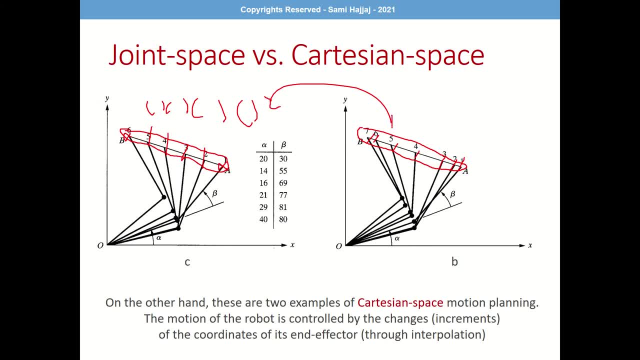 whatever, the difference between here and here is that the increments were different. see, here are more or less uniform increment, but here is not uniform anymore. again, i mean now as i the. the point of showing you this example is you can see now the impact of cartesian space. 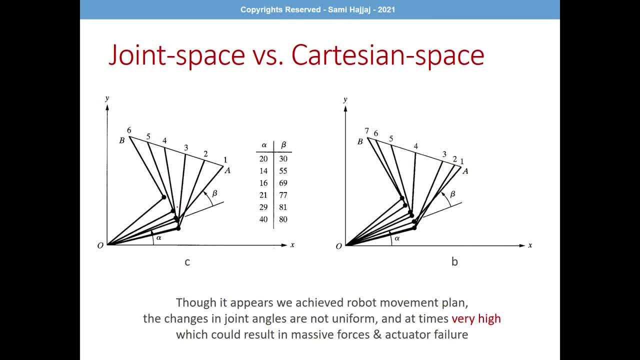 on joint angles. now the difference between these two is that you can see that sometimes the changes could be disruptive. sometimes the values or the differences in position are not constant. maybe here are relatively constant changes, but over here we have not constant. this is a very high change. 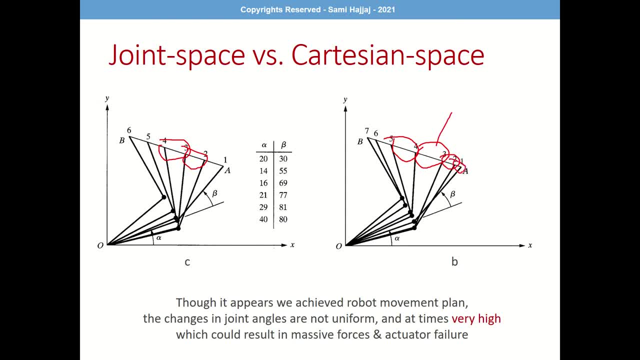 compared to a relatively slower change, and here is also could be very, even slower change. but this higher change in position could also result in even higher changes in velocity and which will also correspond to even higher changes, or you know, differences in acceleration, which again could result in mass cono. 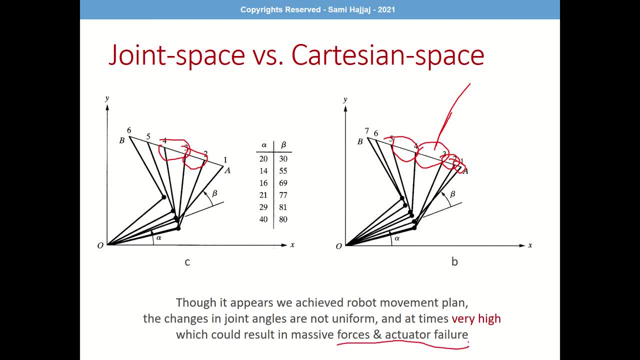 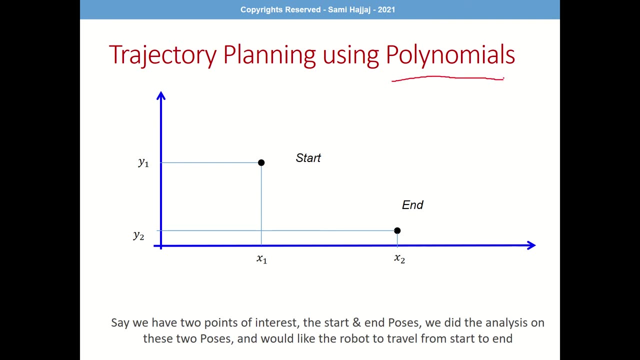 massive forces and actuator failure. So that is why, whether you do it directly from the joint space or the Cartesian space, you may not always find the answer. The answer could end up coming from polynomials, And a polynomial is a mathematical equation. that is we love. 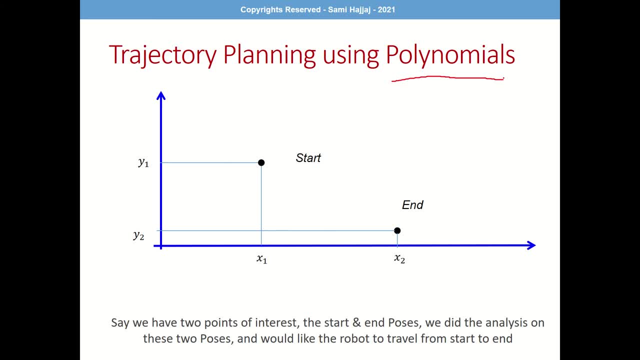 it in mathematics because it can be easily derived and therefore we can easily work with the family of equations along with their derivatives. So this is not a mathematical course. I'm sure you are familiar with the concept of polynomial equation. If not, maybe you can just Google it a little bit more. Maybe I'll share a link to a description on. 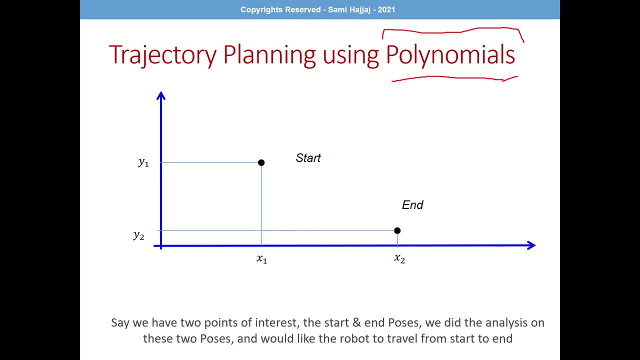 this, but I'm sure you guys can Google this one out. Now let's see about this situation that we have in front of us. We have a starting point and we have an ending point And we have two points of interest. Let's just say this is the start of the motion and this is. 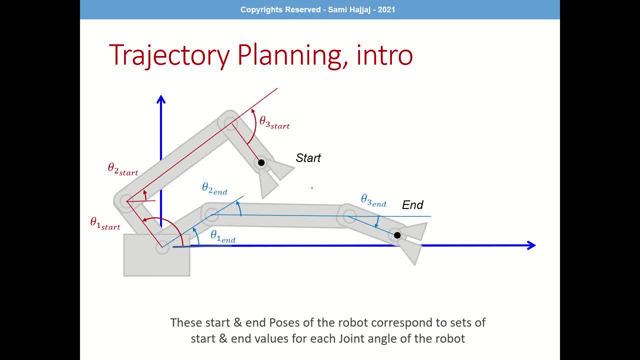 the end of the motion. And these are the two points of interest. And these are the two points of interest. And these are the two points of interest And these two points actually correspond to the robot positions or the robot configurations we've seen earlier. You see, the start point actually corresponds to this robot configuration. 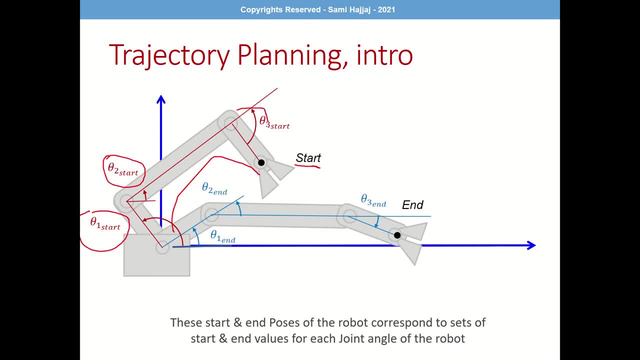 which itself is defined by the values you see here. So the starting point actually is a set of values that correspond robot configuration, And the end point is also correspond to another set of values that correspond to the end robot configuration. Okay, So now you have two. 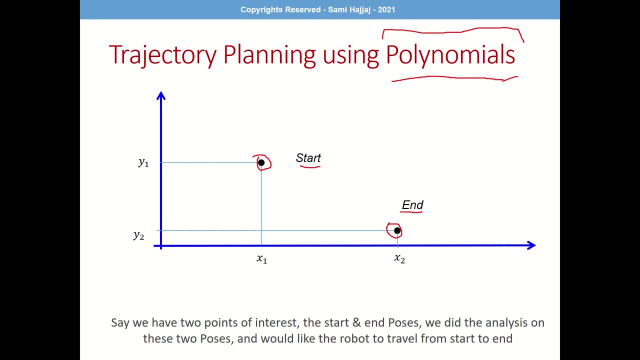 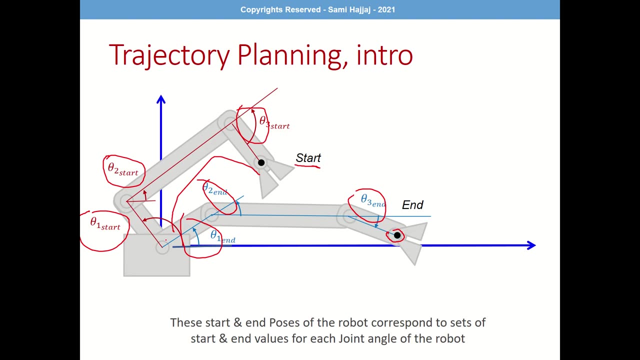 the end, and this points right here represent at the start and a point now. we want to know right now is what happens. I think I missed one slide. yeah, yeah, the point is right now is what happens in between. I would like to travel from here to here, but then what happens at this? 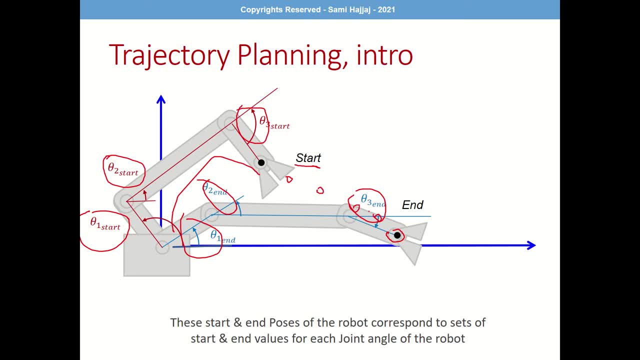 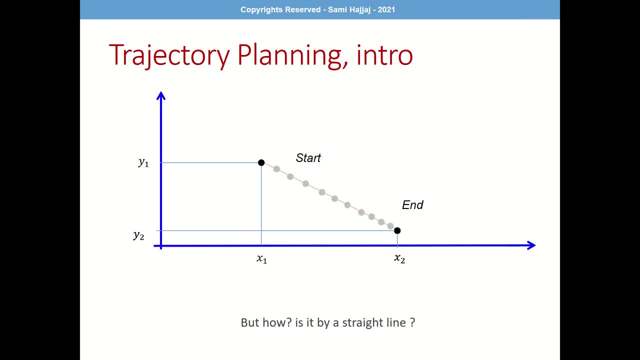 point, for example, or here or here, what is actually the corresponding values for you know the angles versus in between. you might be thinking, okay, a straight line is the answer. right, we could just move the point along the straight, lovely line and we have the coordinates of every point. we just do inverse kinematics. 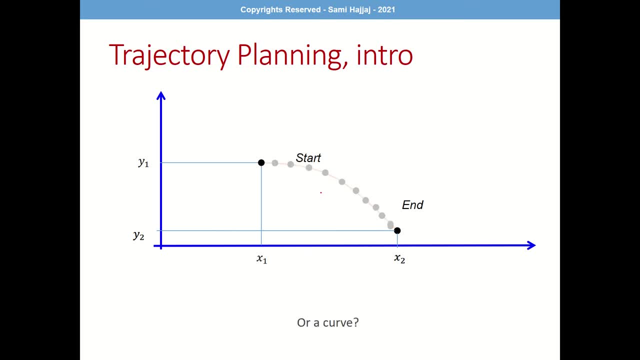 and we have the answer. okay, this would work. but this would also work. I could- you know, somebody else could decide to move the robot along the curve like this, and we could do the same thing- find the corresponding coordinates here, then by the, but then using the coordinates, you can then define. 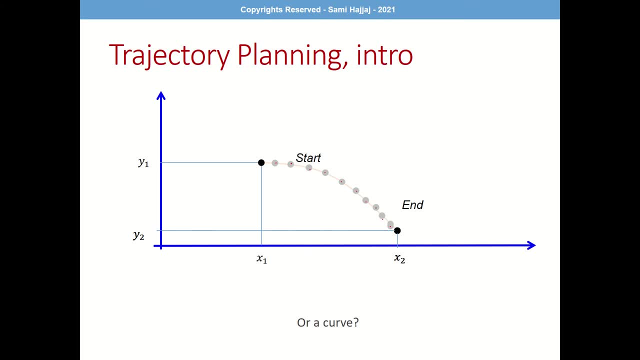 do inverse kinematics and find the corresponding robot configuration. how about this one? this would also work. assuming for a minute that you have an obstacle, you know, maybe you don't want the robot hand to to, you know, to cut, to come to a certain area within the workspace, maybe because you, you know. 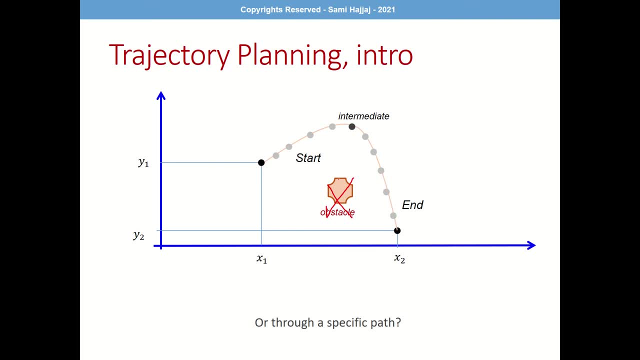 that this is where the robot, the human hand, will be, or the, you know, the operator, will be. so you don't want the robot to hit the person. so you would basically make the robot travel from here to here, and then the robot would travel this path. maybe you would define an intermediate point and then you would. 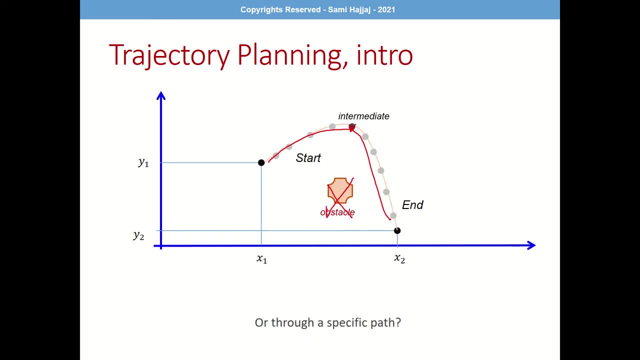 basically make the robot travel along this path. so, in in all of these cases, there's no right or wrong answer. they are correct and they are all not correct. in other words, that this could be valid, this could be valid, it could be valid, it depends on the situation. so this one brings us to the same equation. 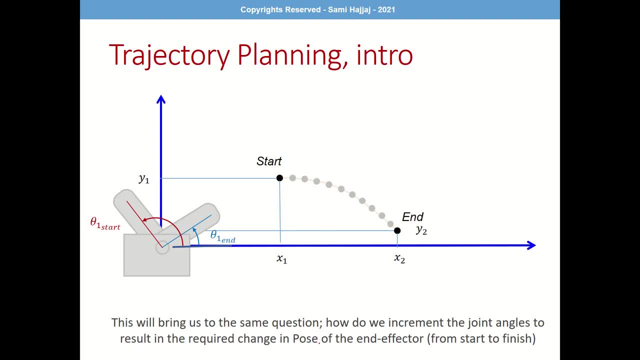 how do we increment the joint angles? that would respond or will correspond to the required changes in the pose. I mean so from the start to the finish. let's say we find the point from here and we find this here, but then that again would prey us to the same problem. what happens in between right say the same. 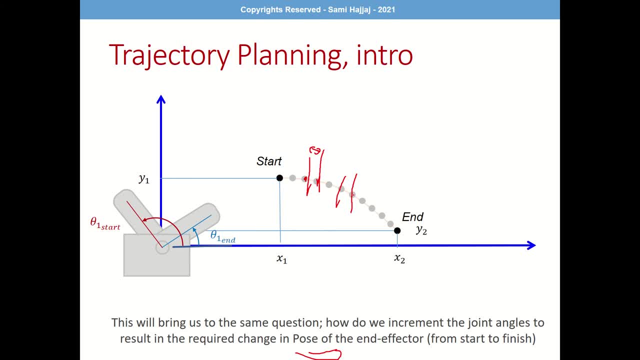 thing here, even if, let's say, we define the values and we do in school here, would bring us here and in between. ok, again, we're going to end up with the same process. you cannot just put the infinite number of points here, because and will result in huge amount of calculation. 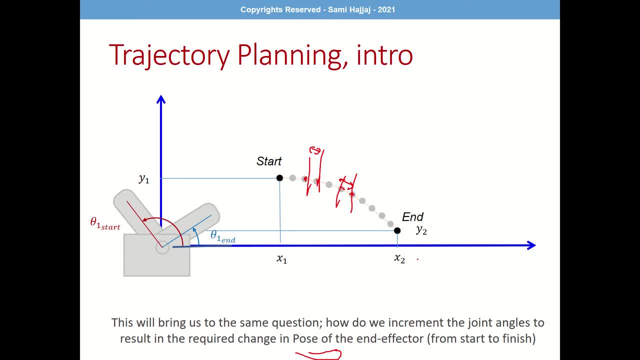 loading open 일본 Ч鐘 on the processor. So again that could cause a problem. You would want a way, or we need a way, to sort of to model the relationship without having to do inverse kinematics every micro millimeter. 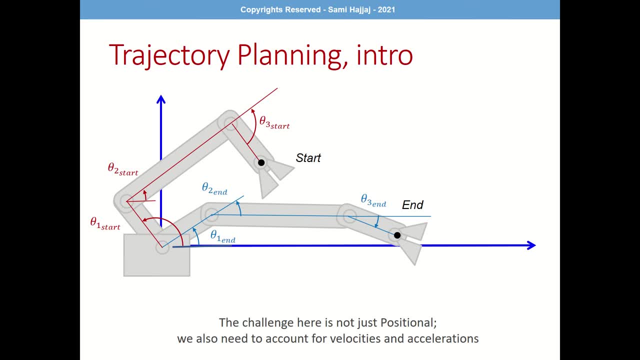 So again, the challenge again is not just positional, It's also involved acceleration and velocities. We just talked about this, that this is not about path planning but it's about trajectory. And trajectory also include timing, because it also gonna affect the velocities and acceleration. 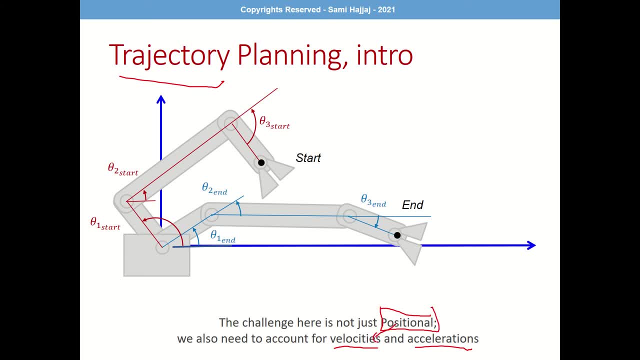 The changes in position through time essentially is velocity And the changes in velocity through time is essentially is acceleration, And we just talked about the effect of acceleration and velocities on the dynamics. They will change forces as well as energies. So that's why we want these two. 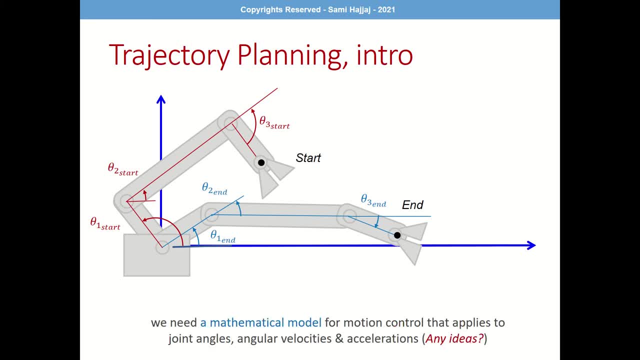 velocities and accelerations to be minimal as well. So we need a mathematical model that will actually help us to develop some sort of formulas or motion formulas or equations that will also put into consideration angles, positions, velocities and acceleration. And if you're thinking about it, 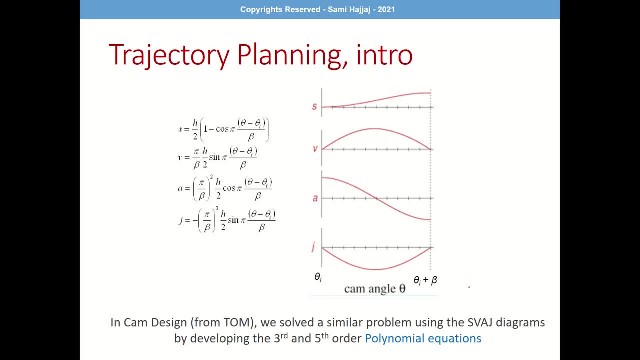 yes, we have done something like this in the past. If those who are doing mechanical engineering taking this course right now, then you would recognize this from theory of machine. I do actually teach, Tom. I mean I did in the past, but not anymore. 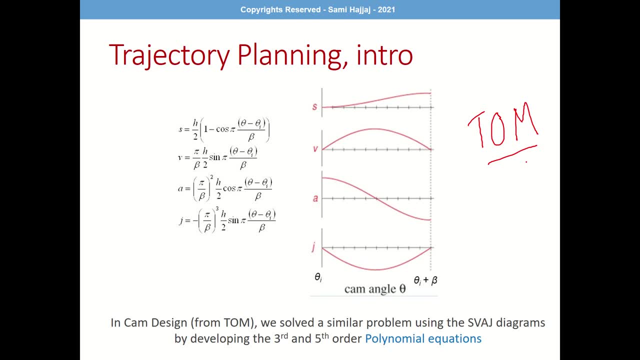 I think I taught Tom for five years And in chapter eight I think, when we did calm desire, we came up with the same or we arrived at the same problem. We want to design the calm, or the transition from the calm from one position or one displacement to another. 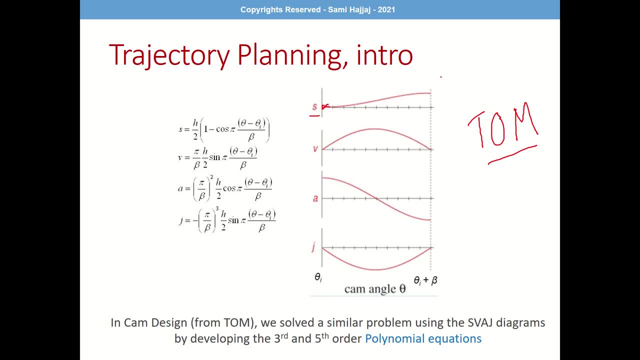 That's the meaning of the letter S here: displacement. This is the displacement from one space to another, while managing the velocity change. velocity changes, acceleration changes, as well as the jerk, which is the derivative of the acceleration over time, or how the acceleration itself is changing through time. 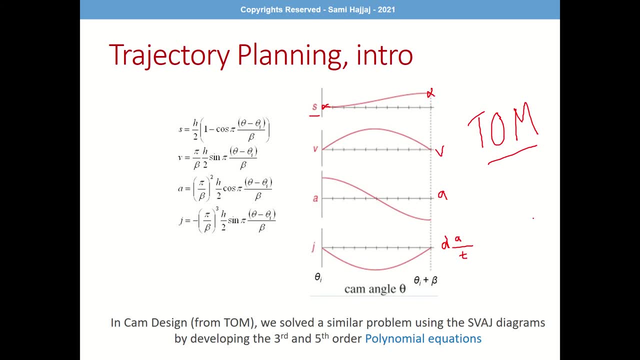 So we want to, we want to find the model that helped us to find, and these are not polynomial, These are actually sinusoidal equations, if you remember, But then these are also similar method. They're also trying to solve the same problem. 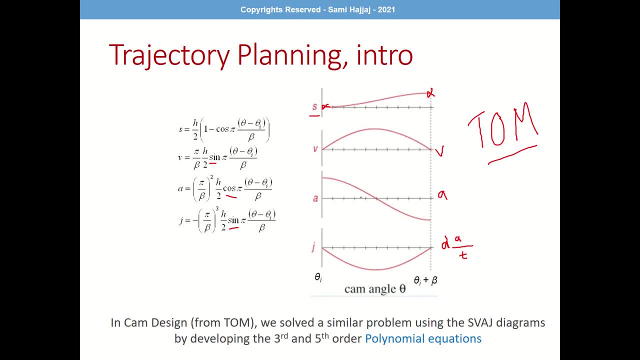 It's trying to find a model that can actually help us to model this motion or to control this motion by putting into mind all of these elements together, the SVAJ, which is the displacement velocity, acceleration and jerk into the motion. 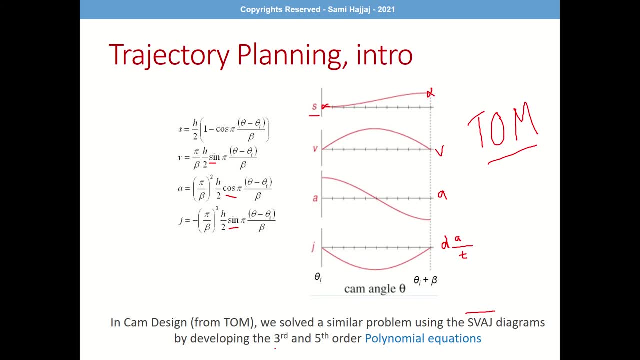 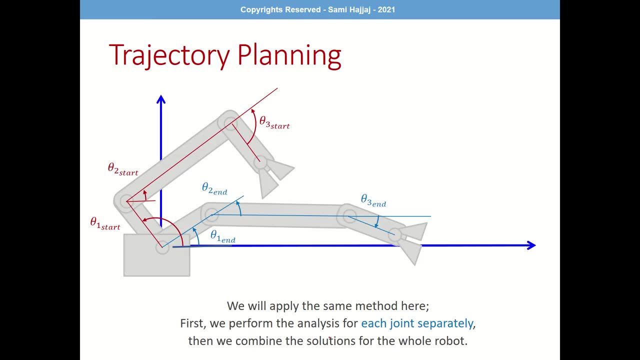 And that's why we used, at that time, the third order as well as the fifth order, polynomial, And at the time, if you remember so, that's how we apply the third order. I hope you remember why we had two versions of the polynomial. 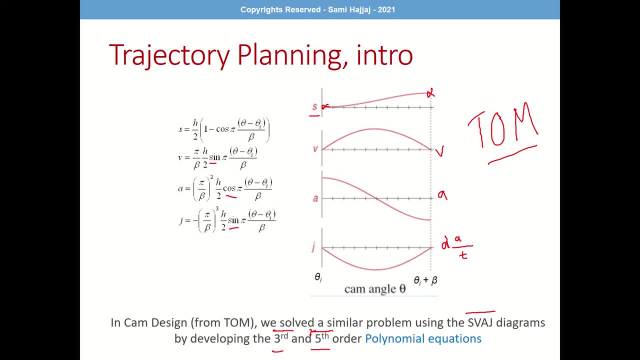 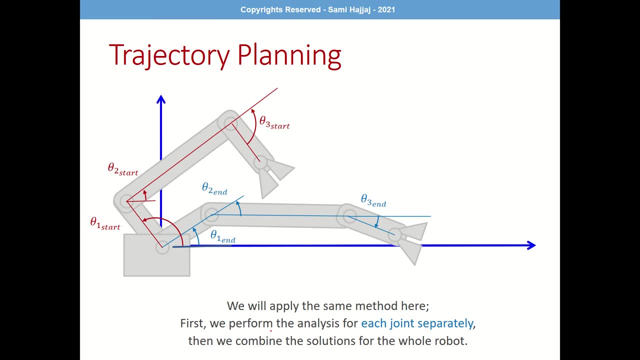 I hope, if you don't, the reminder is coming soon, but that, basically, we would see in a few slides from now. So, coming back to our robot example, basically it's the same. It's the same idea. We have two positions: starting and ending. 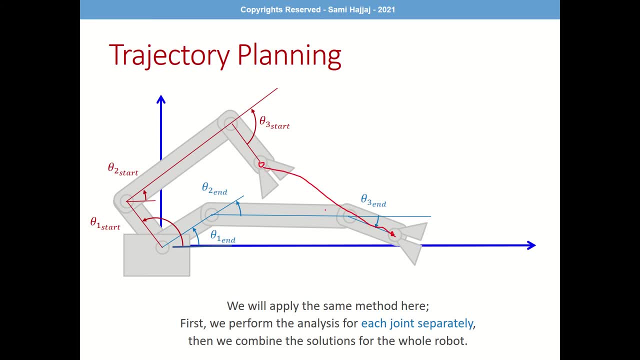 and we need to sort of create a model of motion that put into consideration the changes in position, in this case, theta as well as angular position, theta dot as well as angular acceleration, theta double dot or, if you'd like, this is alpha omega and this is alpha. 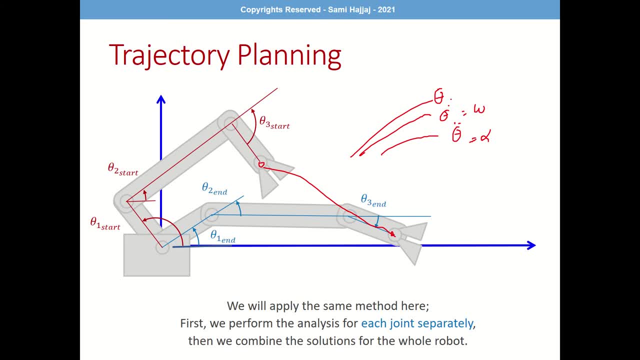 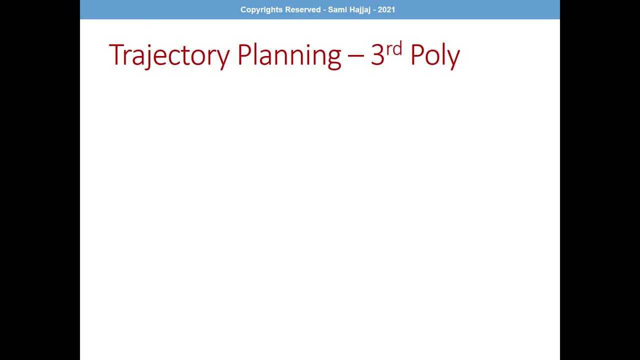 And so, therefore, you would want to put a model that puts into consideration all of these motions or all of the kinematics At the same time, And that brings us to trajectory planning. third polynomial, And I think this is already the procedure, So the third order polynomial is going to be used. 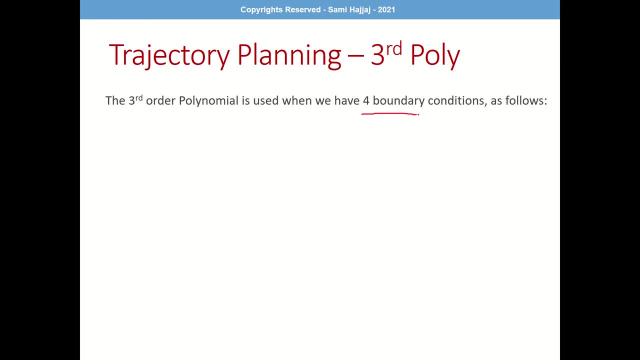 when we have four boundary conditions. There's a formula for that is that the number of order is equal to the number of boundary conditions minus one. So four boundary condition minus one gives us the order that you need. I think yeah, So order. 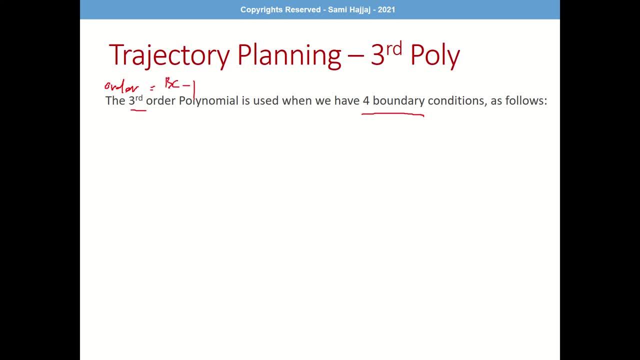 equal to boundary condition minus one. That's the formula. So four boundary condition minus one gives us third order, polynomial. So these are the four boundary conditions that we have: The position at the start, which is, at t, equal to zero, and the position at the end. 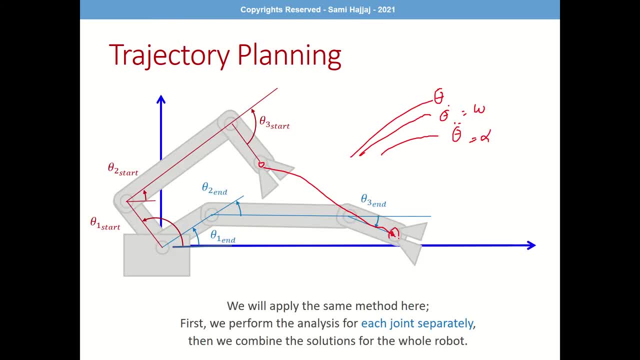 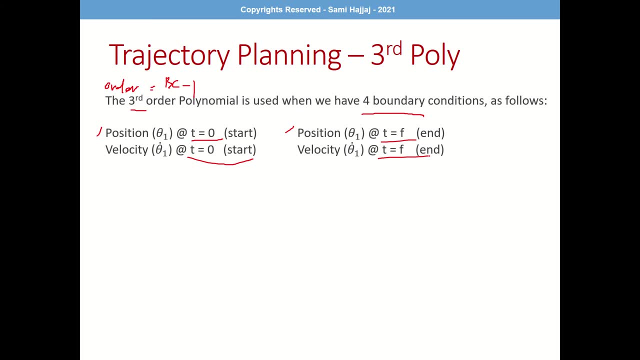 And this one is readily available to us, because we already have the position at the start and the position at the end. Okay, what's next? What's next is that we need the velocity at the start and the velocity at the end as well. 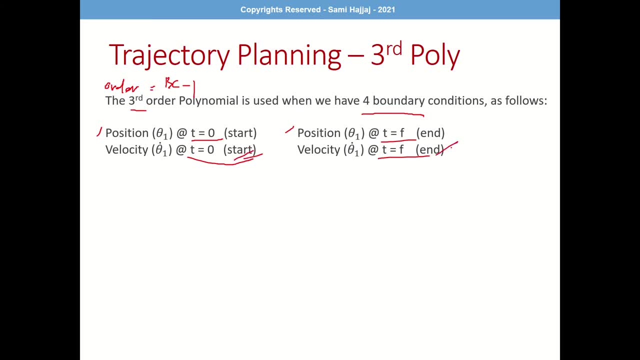 We could have. we could define a specific value right here and a specific value right here, And that will be our. actually, we're really gonna do that. We're gonna define a certain velocity at the beginning and the velocity at the end. 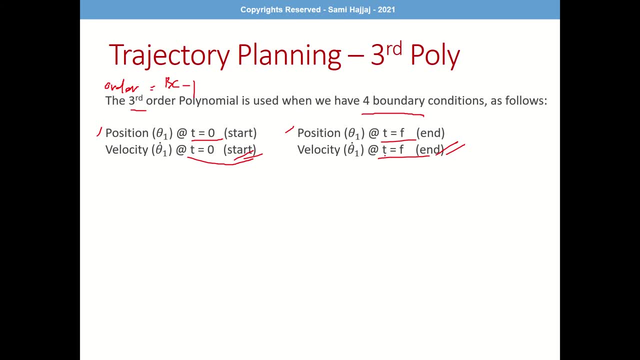 And that will be our third and fourth boundary conditions. Then, once we have these four boundary conditions, then the motion, or the motion of joint number one, or theta one- essentially not just theta one could be any theta, by the way- will then will be defined using this equation: 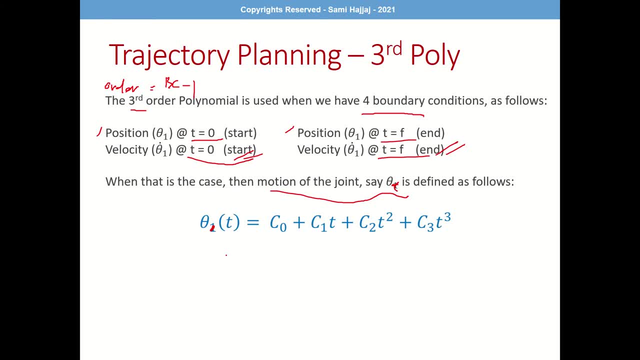 which is the value of the position, will equal to c zero. until the end, as you can see, until the t to the power three or t cube. And this structure you see right here essentially is the polynomial equation, with time as the variable and with four coefficients. 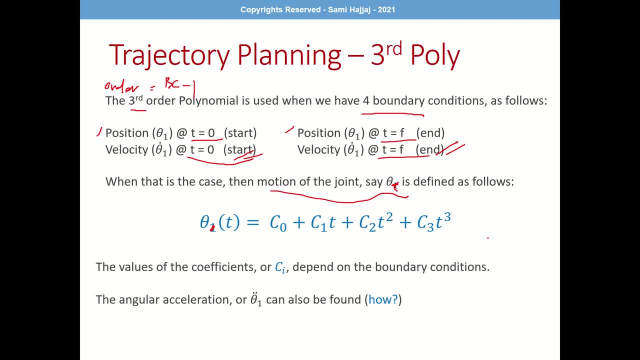 C values. you see in front of you are the coefficients. And, by the way, I'm not teaching polynomials here, I'm just revising. So once again, if you have, if you do not remember or do not understand what is polynomials, I suggest you stop. 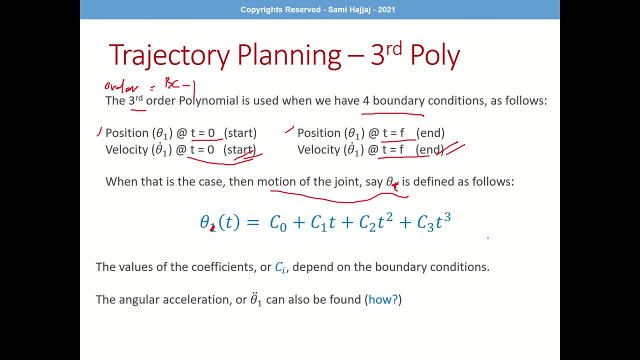 this video now and Google the concept on polynomial, or you can take a look at the link in the description and watch that video, or read that article first and then come back at this point. Okay, but again, since you are, this course is an elective course. 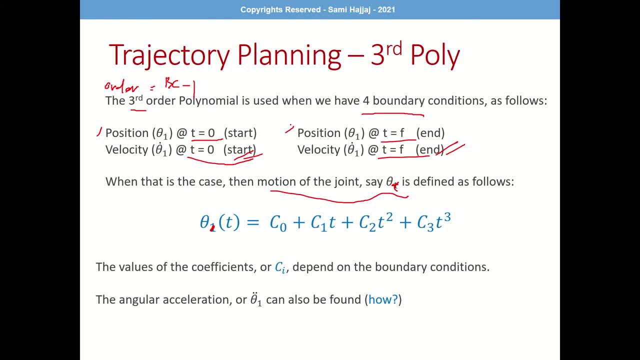 and you already passed on a couple of years ago, So you should remember the polynomial. if you paid attention back then. Okay, so now we are here. So the values of the coefficient CI, or basically coefficients zero, one, two, three. 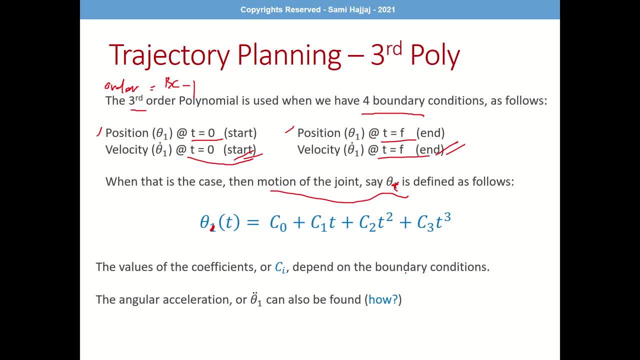 until the end right are depend on the boundary conditions. So the way you're gonna find them actually is dependent on the boundary conditions. Now, even though that we considered only position and only velocities, we can still solve and find for the acceleration. 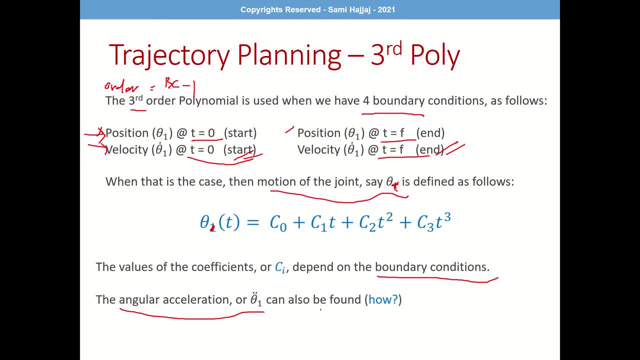 even though that it was not part of the boundary conditions. I will leave this for you to think about is: how do we do that? Once again, this should not be difficult to work out for you, because you have already seen how polynomials work. 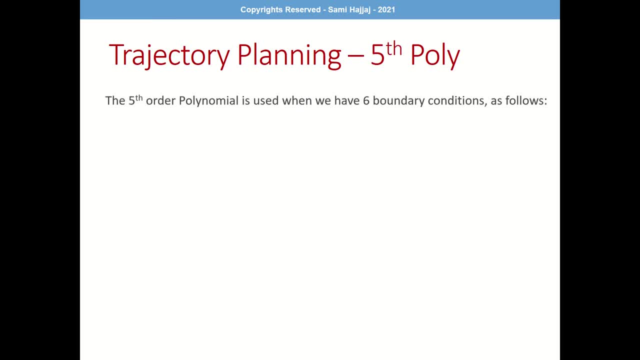 in the theory of machine. Okay, fifth order. Now, if you are already familiar with third order, or if you have already solved examples on third order, then transitioning to fifth order will be pretty much straightforward. It just is gonna be more work, more calculations. 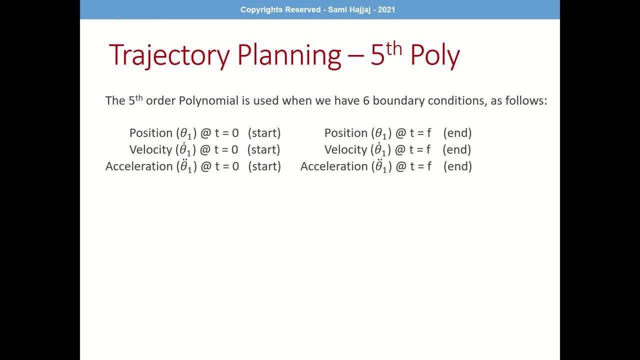 but the procedure is more or less the same. So for now, because we have six boundary conditions, we will need five. We will need the fifth order. Again, the formula that we seen earlier here applies, which is the order of the polynomial equal to BC minus one. 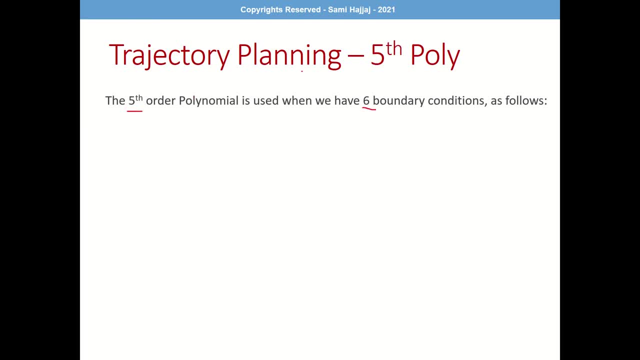 or the boundary conditions minus one. So here we have six boundary conditions minus one. that gives us fifth-order polynomial. So now, these are now the antioxidant, the boundary condition spent. Now we're gonna involve the position, as well as the accelerations, into our analysis and you need six values. 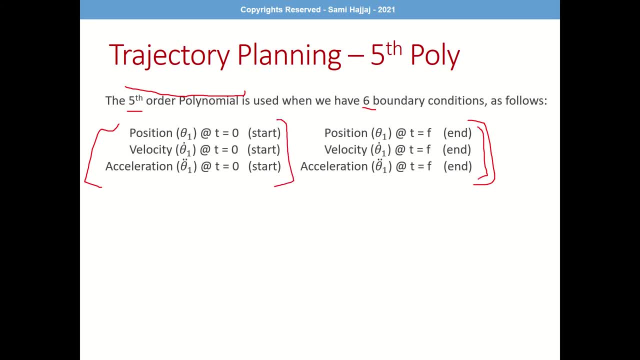 three for the starters and even two for the first. if you get the fundamental, the relation between the position, You will need six values: Three for the start and and 3 for the ending. that will give us the 6 boundary conditions that we will need, and 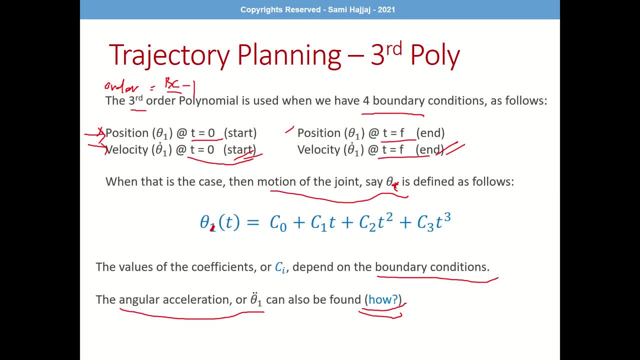 then we will use it to find the balance. And by the way, this was a typo, I think this too. it's not necessarily or limited to just theta 1, this could be any theta or any joint. I think when I was making this slide I forgot. 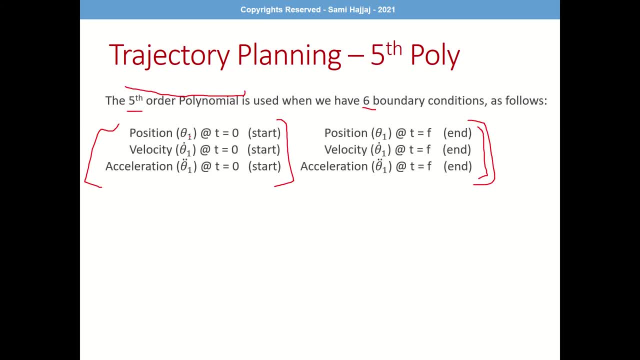 to remove this number 1 here, but it's actually any joint or any angle for any joint, so it's not necessarily limited to just theta number 1.. Alright, so let's just put that note somewhere, okay. And similarly the equation of the position of this joint essentially again is defined: 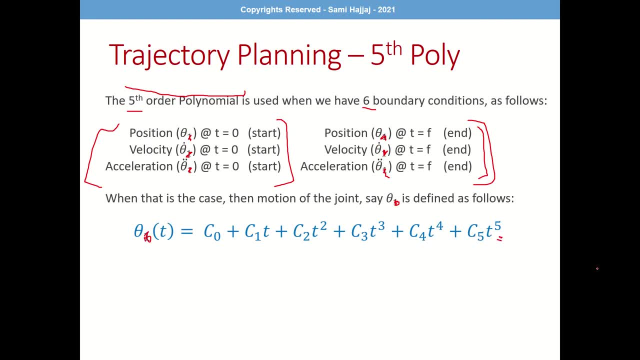 or using the 5th order polynomial, which it ends at the power of 5, and again we have 6 boundary conditions. So 1,, 2,, 3,, 4, essentially they start coming from 0, so there are 6 C's. 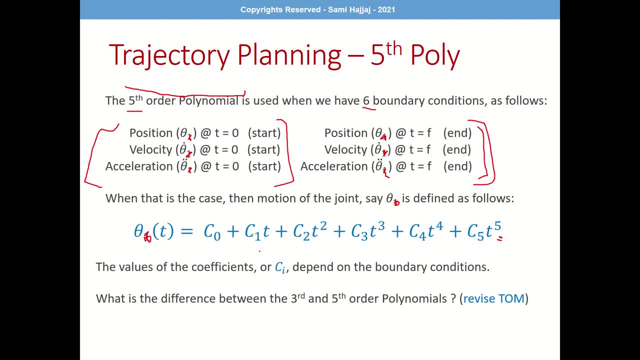 But the procedure is exactly the same as 3rd order polynomial: A little bit more work, but it's exactly the same process. Using the boundary conditions, solve and find the coefficients, find the constant values. then you then not the coefficient? yeah. so the values of the coefficients? yes, which? 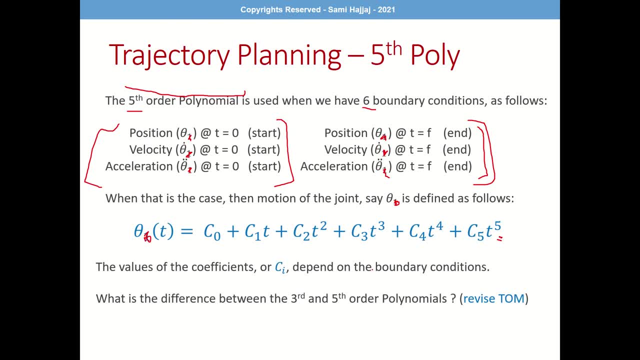 is, the C's values depend on the boundary conditions. So once you have now there is a difference between them, anyone can? I'll give you a moment to think about it and try to remember what is the difference between them. Okay. 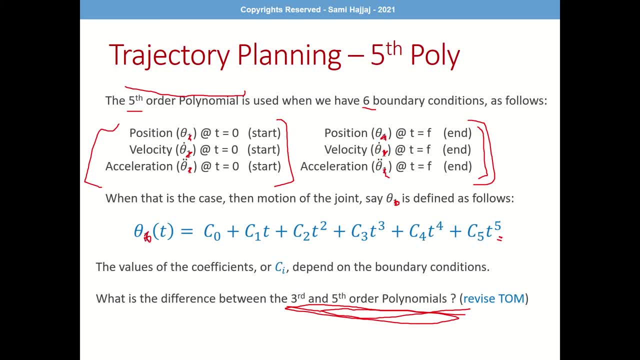 Apart from difficulty, what is the reason why we come to 3rd order polynomial? You see, let me explain what's the purpose of this question. You see, both of these two powers, whether it's 3rd order or 5th order, they're both. 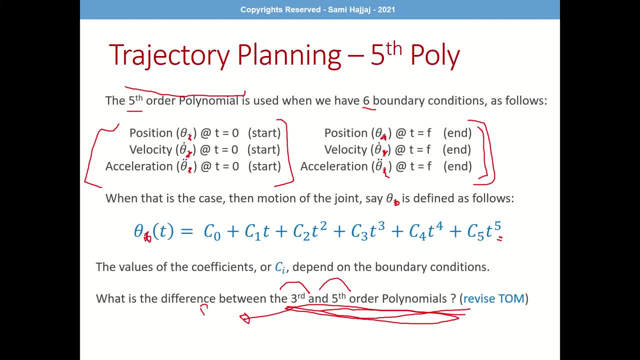 going to give you the kinematics meaning they're both going to provide you with position velocity and acceleration. And this one too: position velocity and acceleration. where is mine? yeah, position velocity and acceleration. So what is the difference between them? 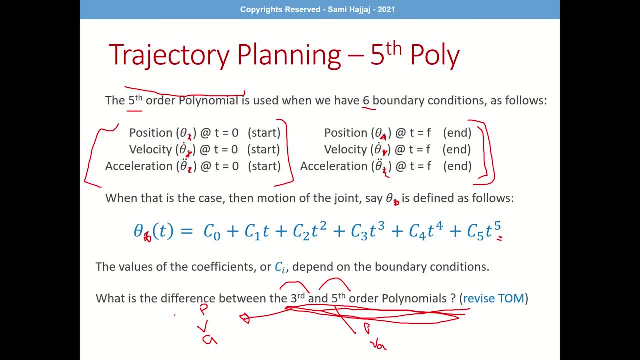 Okay, I'll give you a moment to think about it. you can pause and think about it, Okay, so the difference between them is that here, although the 3rd order polynomial gives us acceleration, we did not include acceleration in the analysis itself. 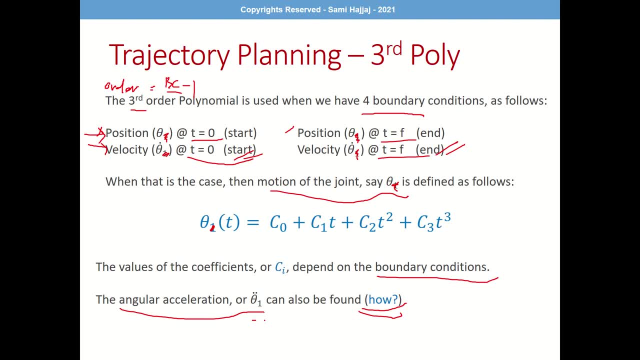 If you go back to this previous slide, you will see that, although we can find the acceleration from here- and, by the way, the answer to this question is simple- is that once you develop the formula or the equation for velocity, right, you just differentiate this one with. 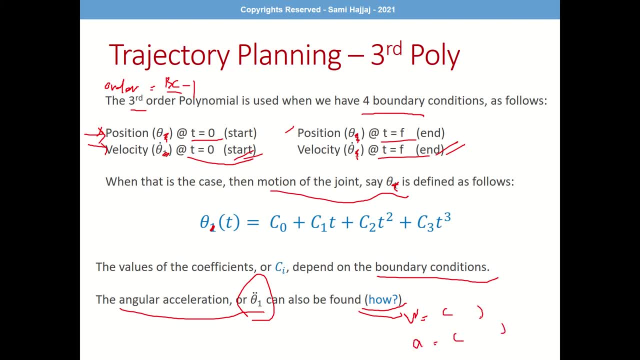 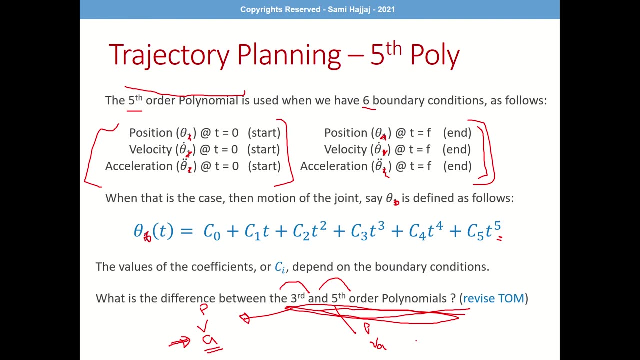 respect to time, You will get the formula for acceleration. it's that simple. So once you develop the expression for velocity in terms of time, then just differentiate that with respect to time, you will get the acceleration formula. okay, So the difference now is that either now here we start with values, now the difference. 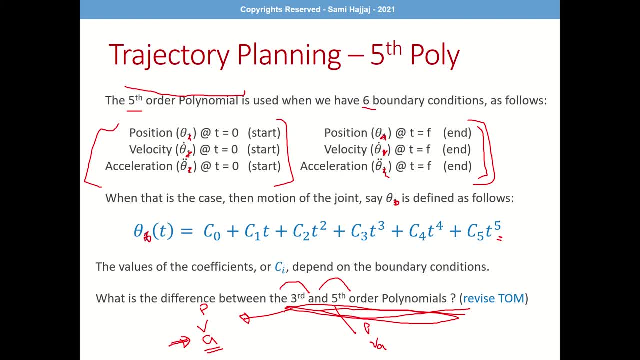 between the 3rd order and the 5th order. you see, although both of them they give you kinematics, we did not include acceleration in the analysis. So, as a result, you might think, okay, I'm going to do this. 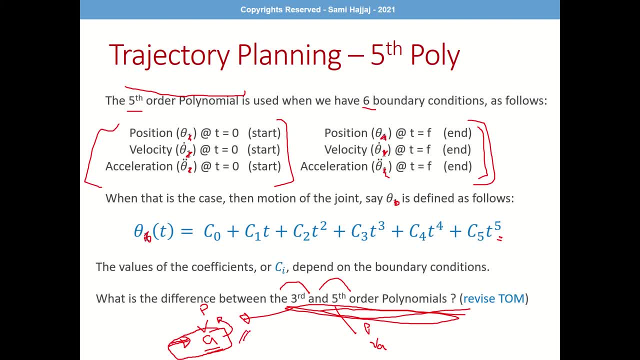 Okay, You might end up with problems here, meaning you might end up with a situation that, although the values of the acceleration could be found, but it could be still causing you problem, You could end up with sudden shifts of acceleration. You might end up if you're not careful. let me try to draw it over here. yeah, 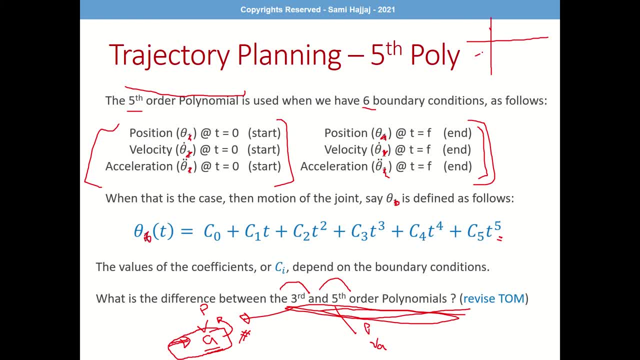 So over here your acceleration diagram might look like this: if you're not careful, like this and then suddenly like this: within the time, within the range of the angle, So although the values of acceleration here and here is fine, but then suddenly you have 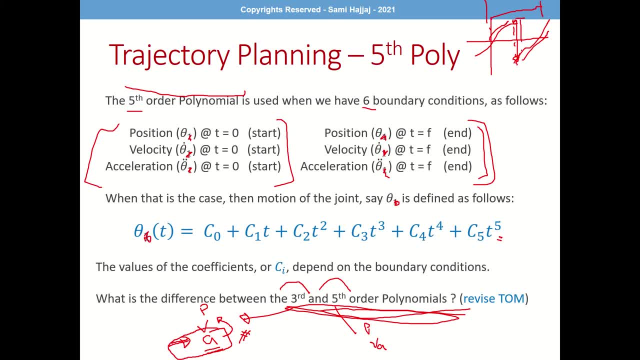 a change in acceleration, a huge magnitude of change, but then with zero amount of time. You see, remember, or excuse me, velocity, yeah, this could happen in velocity. yeah, So, if you have, if you remember, dv over d time or you know, time essentially is the. 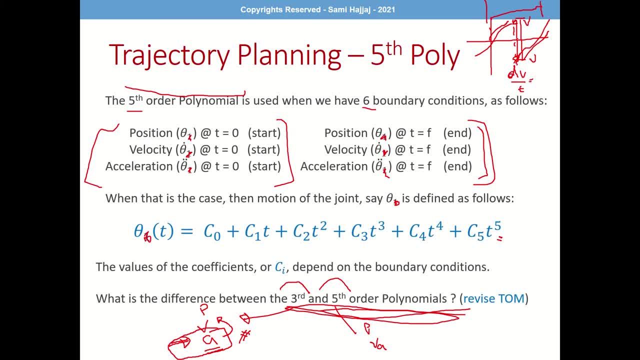 changes in velocity over time. So if we have a big change in velocity, as you can see here, but the time is almost zero, this could end up almost equal to acceleration- Okay, Equal to infinity, or very, very, very high amount of acceleration. 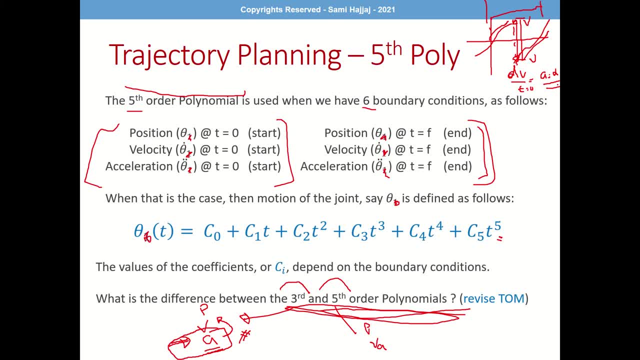 And that could translate in real life into very, very high amount of forces and torques. So that is why using third order polynomial, yes, easier, but then not safe, we should say. That is why the fifth order polynomial is safer, because you would incorporate the values. 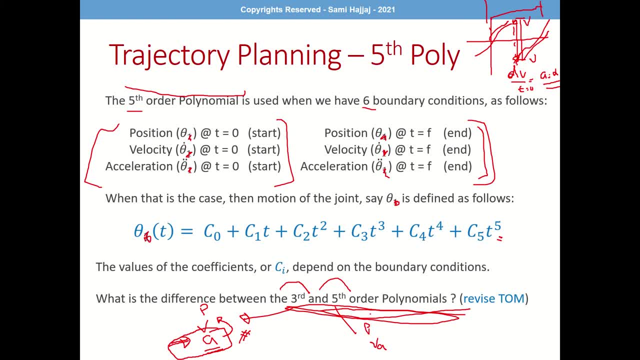 of the accelerations a lot more safer compared to the fifth order, polynomial. You would not end up with this situation because you've already accounted for acceleration changes beforehand. So that's why- pros and cons, yeah, Third order is easier, but then could still result in problems. 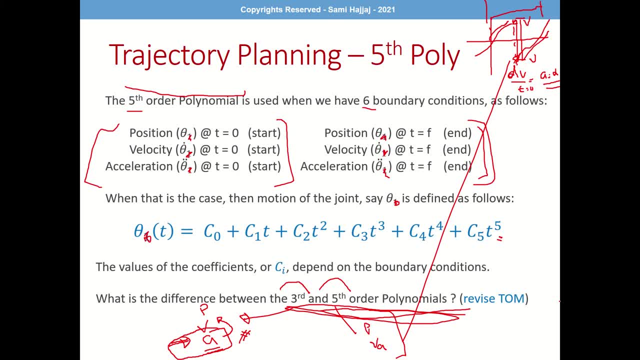 Fifth order is a little bit more difficult, but then more accurate. Now, of course, when I say difficult or more difficult, I'm talking about if you want to do it by hand, But of course, if you right, if you use MATLAB or any software, then of course you should. 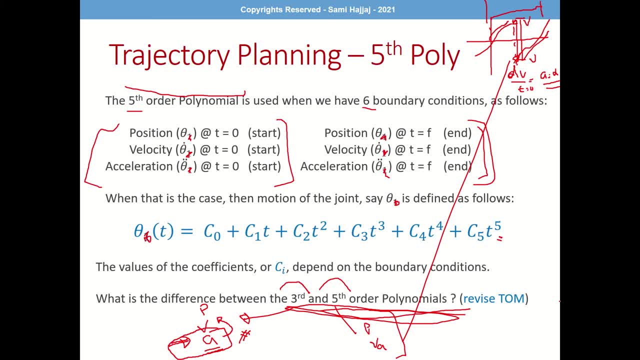 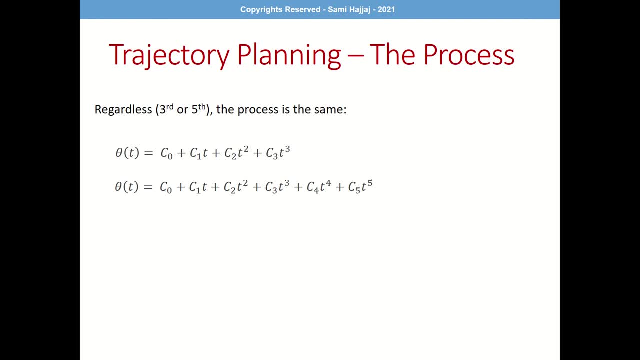 go for fifth order because you will not be doing the labor work yourself. MATLAB or any software you develop will do the hard work for you, Okay, Okay, Last part before we begin the exercise. Okay, So, regardless whether it's third order or fifth order, the procedure is usually the. 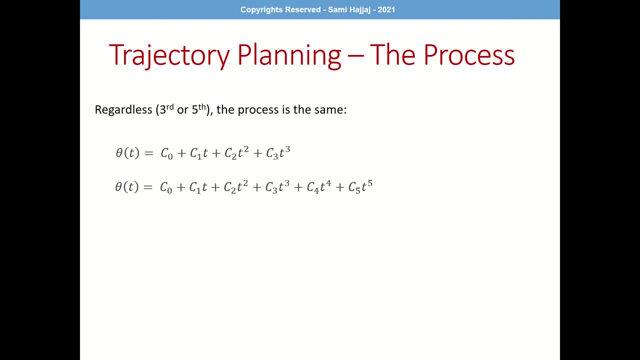 same. This is the third order example and this is the fifth order, And I think this time I properly removed the 1-1 from here. So, whether it's third order or fifth order, the very first step is important, Based on the given information, AKA the boundary conditions. 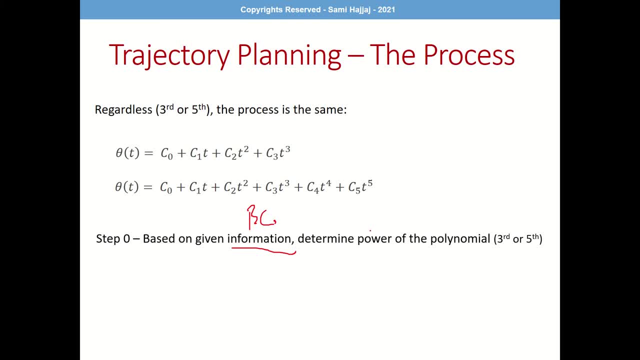 Okay, So you will then determine the power that you need, whether it's third order or fifth order. Basically, if you were given four information or four boundary conditions, then we are here, But if you were given six information or six boundary conditions, then you are here. 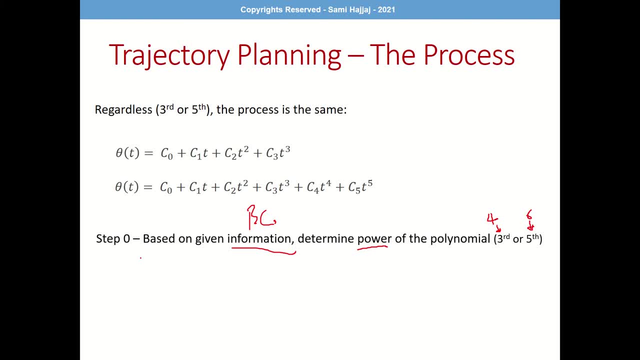 So, based on that, you will know which equation are you working with. Is it third order, which is this example right here, or third order, or fifth order? Okay, So you know, You know which one are you working with. Second step: 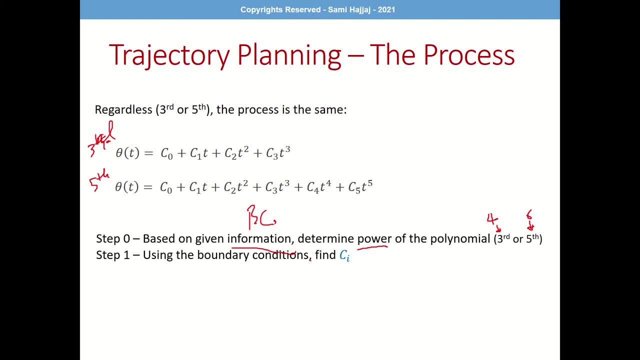 Okay, After you determine the power and the version of the polynomial you're going to be working with, then you're going to use those boundary conditions to find the coefficients, And this is essentially a matter of using algebra. really, You will have equal amount of equation, equal amount of unknowns, just solve and end up. 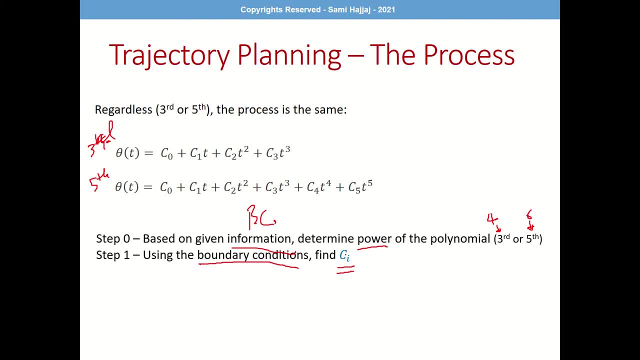 Now the difference between this, between third and fourth, is right here, You see, in the third order. when you actually come here, you will end up with a two by two system. Third order: Yeah, You will end up with a two by two system. 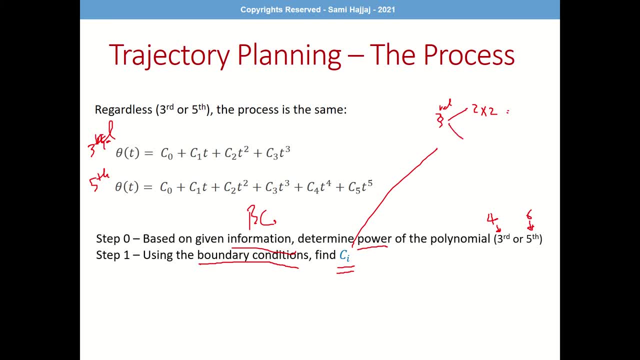 What does that mean? Basically, two equations and two unknowns. So obviously this is relatively easier to solve. But in a fifth order- polynomial right in a fifth order- you will end up with a three by three system of equation. So you will have, essentially, this is terrible, okay. 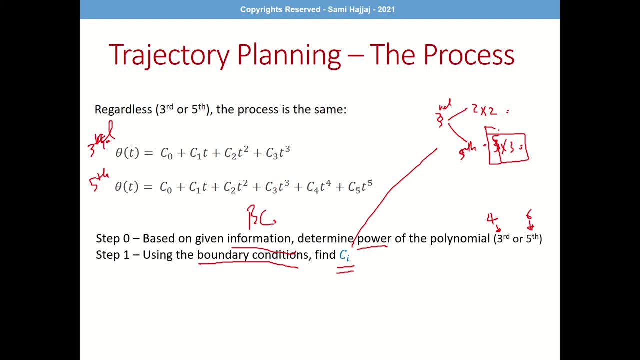 You will have three equations and three unknowns, which is still doable, but again you will need more time if you're doing it by hand or using your computer, But of course both of these situations are easy if you're doing this using software. 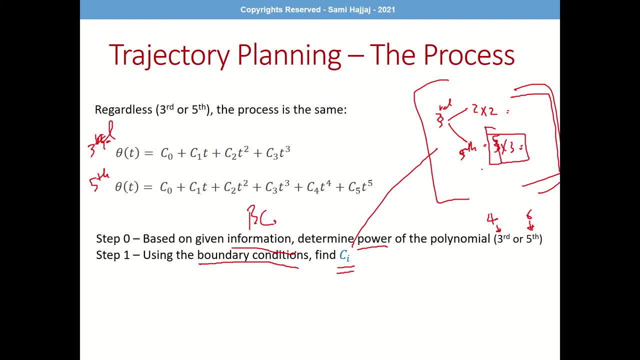 Now, if you're doing a test on paper, then obviously you will do it by hand or using calculator, So you need to put this into consideration. I mean, when it comes to time consuming, when the time management and stuff, of course, calculators. 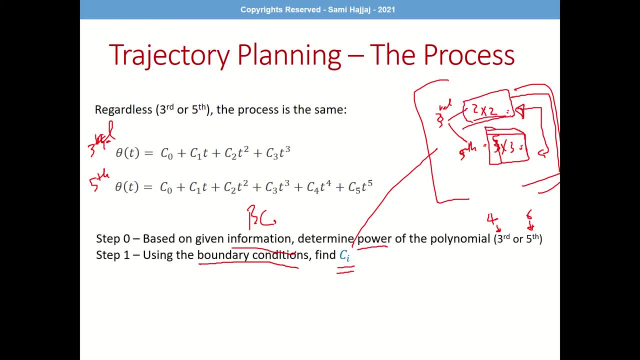 can sometimes help you. Some calculators can help you to just plug in the values and then it will find the solutions for you. You might want to learn more about your calculator. Okay So, once you develop the coefficient. Okay So, once you develop the coefficients, and then what? 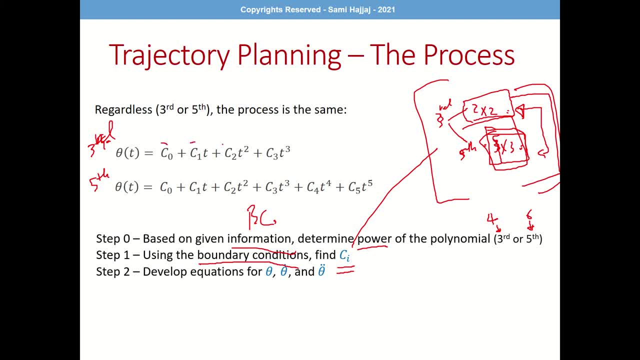 But then, once you develop the coefficients, you can just plug them in here and then you can develop the equations where the only variable will be the time variable, and that will be the equations that we are talking about here. Let me clean up a little bit here. so let's just move this extra line, yeah. 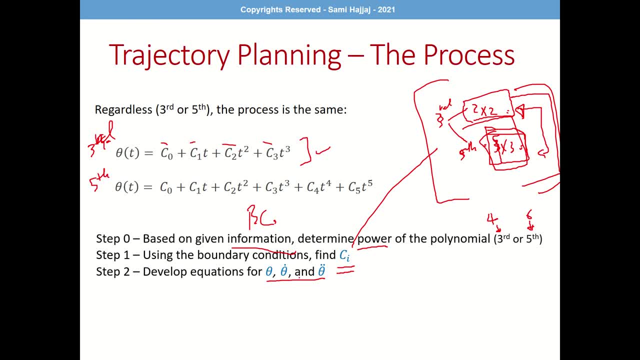 So essentially, once you find the values for coefficients, then you can then develop the equations for the kinematics. We can call these, we can sometimes call these equations the kinematics equation. Kinematics obviously because they involve position, velocity and acceleration. so kinematics. 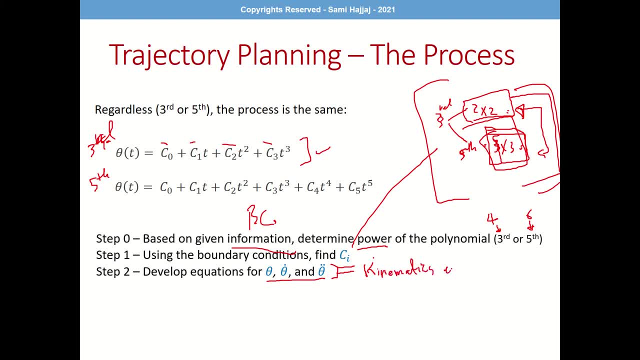 equations Right, Then of course that means only function of time. There's no other variables here, so simply function of time only. Okay, So once you have the formulas in terms of time, only then we know that we are done. 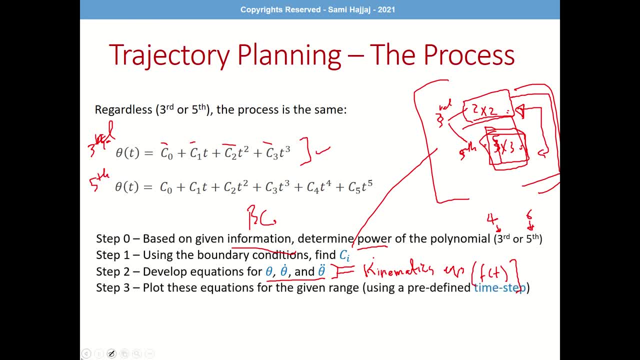 Then next, once you're done, then you can simply plot using a predetermined time step, A time step, Okay. So a time step essentially is, you see, when you actually start the procedure, you must have a starting and ending point. 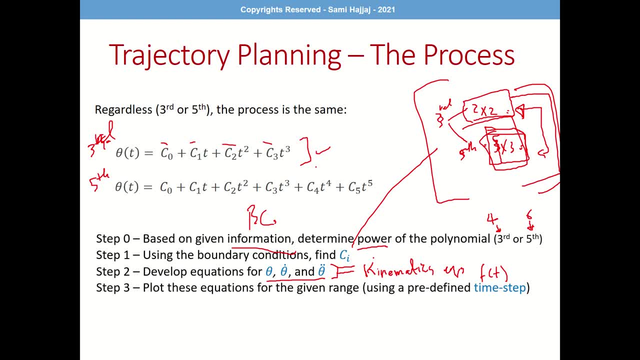 So what does that mean? You will have to say that I mean the analysis will be limited to, let's say, you know, from t is equal to zero, to t is equal to say three. So all the analysis that we're going to be doing here, all of these steps right here, 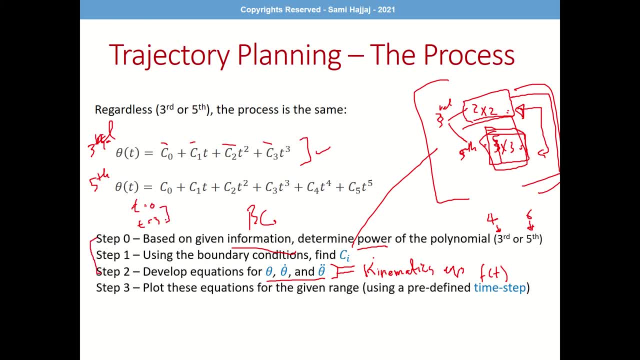 right, it will be based on the situation from time equal to zero to time equal to three. So when you want to find some values or you want to do some plotting, you want to jump from zero to three, but you want to do some sort of an interval, like sort of an increment. 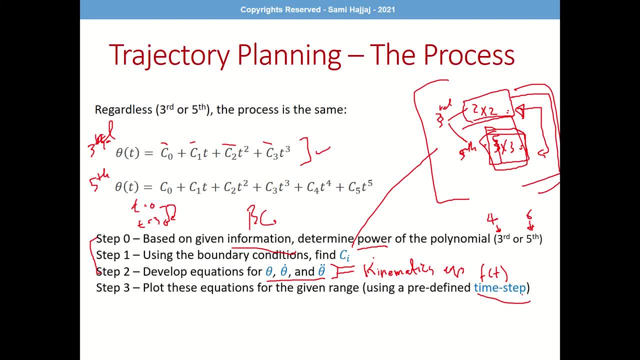 So that is usually defined using a time step. A time step essentially could be, let's say, 0.5 seconds, So that means you're going to start from zero, then 0.5,, then 1.0,, then 1.5,, and so on until. 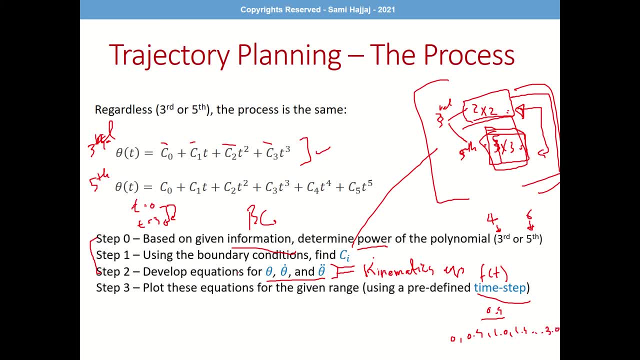 you get to 3.0.. Okay And then? so, therefore, that's what I mean by you can then use it. Okay, So you can use the equation and the plot, find the values based on the time step. So the time step in this case will be the value of 0.5. 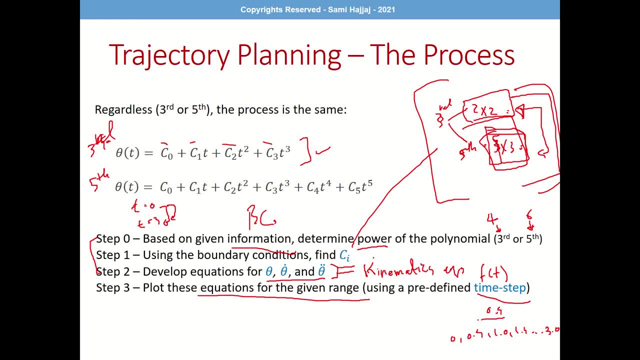 So in this particular example, the time step we find was the value of 0.5. Maybe somebody? we don't want to go for 0.5, they want to use one as the time step. So in this case we'll go from zero, one and then two, and then throw it away to three. 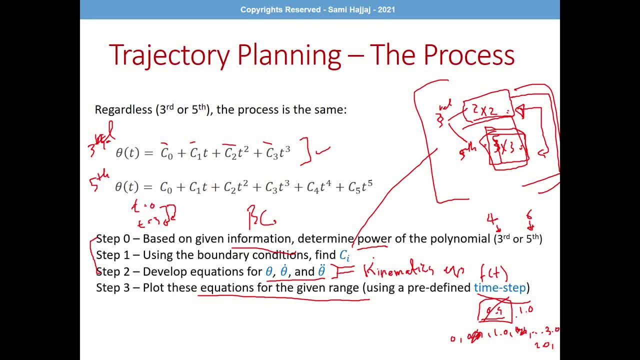 So this is the difference. Of course, the smaller the time step, The smaller the time step, the more accurate the diagram would be. But again, the more work you'll have to do in calculation and in plotting. But again, it's as long as you have the equations ready, then it's just a matter of routine. 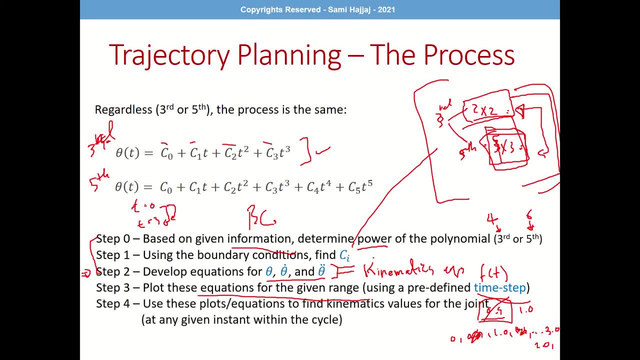 really, You have the equations, just plug them in and you're good to go. Then you can use the plots and equations to find the kinematics values for the joint at any given instant. Once you have the plot, the diagram, and once you have the formula, then you can then find: 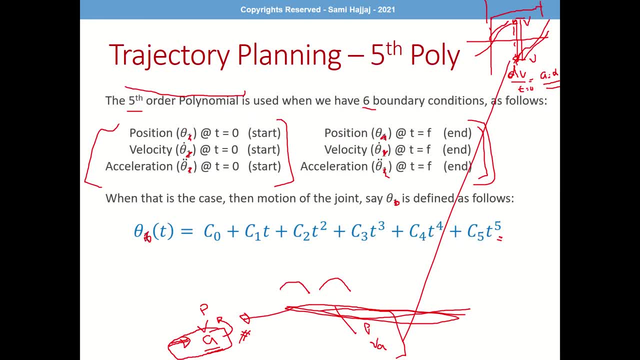 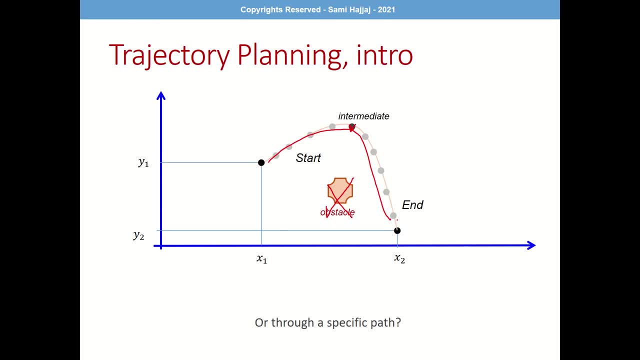 it to find any instant in between, And that actually is the solution to our problem. Okay, You see, if I actually already have the starting here and here, so I don't really need points in between, I will straight away develop a formula or a, you know, a final formula that will give. 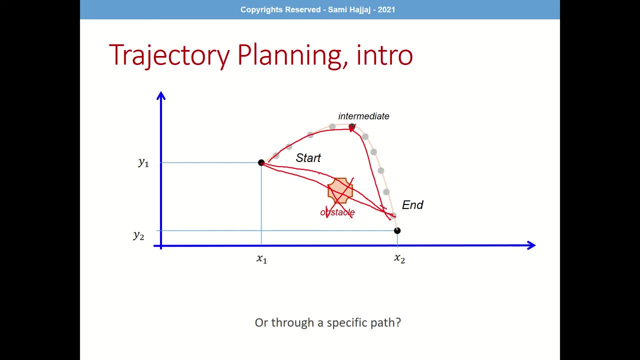 me a curve. So this curve right here is not defined by individual points, and then I'll have to do inverse kinematics. No, the formula itself for this curve will be given to me. So, essentially, the analysis that we're going to do, the trajectory analysis, let's go to 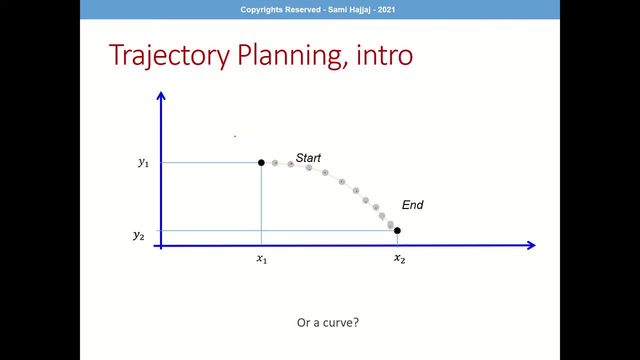 yeah here, So I don't have to actually do the step. I don't have to define it. Okay, Define these individual points, find their original coordinates and then do inverse kinematics. No, I really don't need to do any of that. 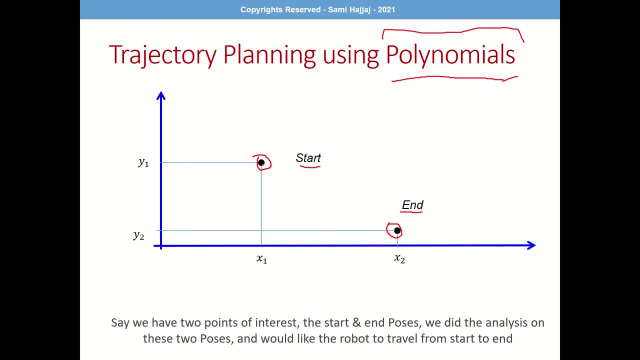 All I really have to do is do this trajectory analysis and boom, I will have a formula function that will define this curve right here. So, therefore, the formula is available Now, at this point, at any instant along the curve, of course, my current curve, you see. 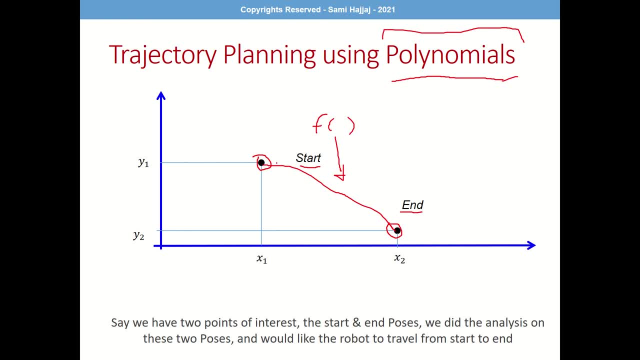 in front of you is very ugly, but you get the idea that it will be a very smooth line. And then then, at any point or at any instant in between, you can then find the value or the corresponding value of the joint. And similarly, we can then take this formula and then plug it into the controller, which 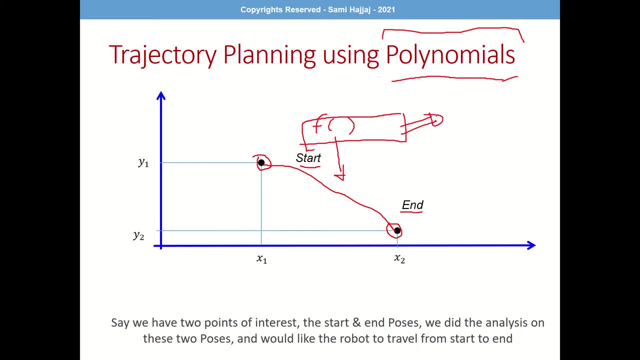 will then be used to basically control the motion. So rather than going point by point, we will simply give the formula into the controller as a controlling algorithm, And then that then will control the motion from the start until the end point And also through the proper time. 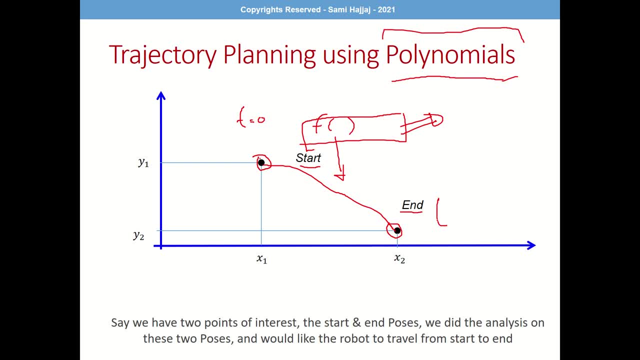 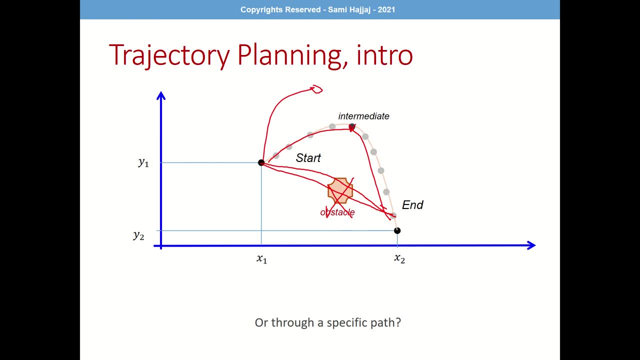 So, from t to n, From t equal to zero, which is at the start, until t equal to final, which is at the end. So this is what I mean by trajectory analysis using polynomials. okay, Where are we? We are here, okay. 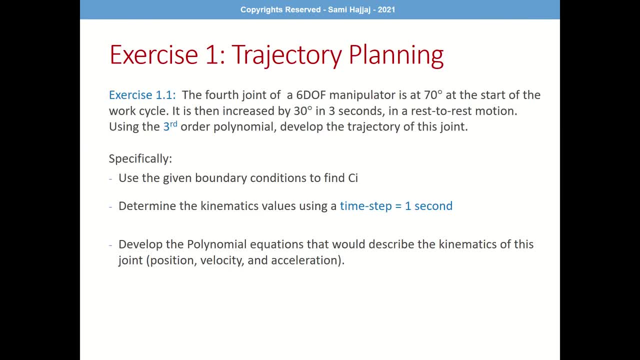 So, and we talked about this And now finally we do exercise, So we're going to go with this last exercise or this exercise and then basically we will be done with this session for today. It's about: yeah, it's under an hour so far. 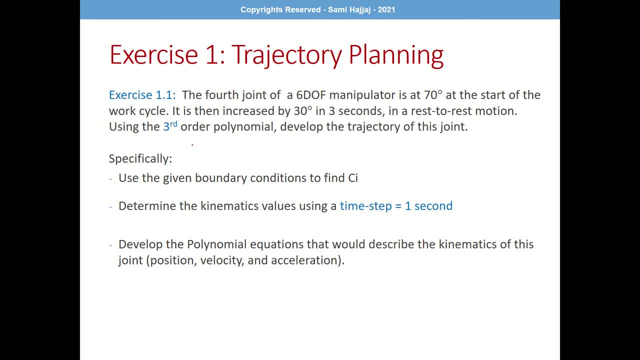 By the time we're finished with this exercise, we'll be finished already, So let's take a look. So again, when you read this question, if you have done Theory of Machines, then this question will look and sound very familiar to you. 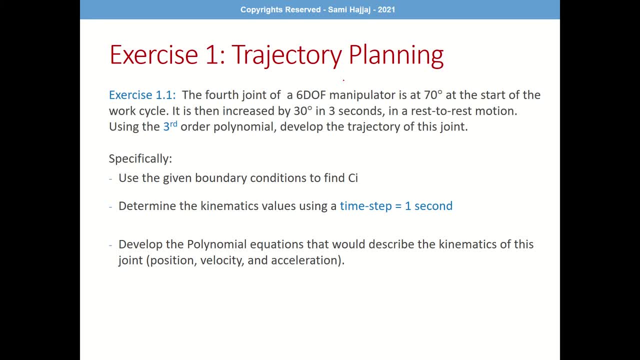 The third. just some of the words will be different, but the values and the numbers will be very, very familiar to you. So this is the fourth joint of the six degrees of either manipulator. Oh sorry, The fourth joint of the six degrees of either manipulator is at 70 degrees at the start. 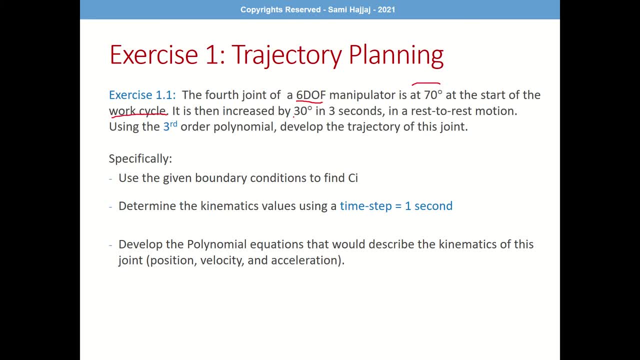 of the work cycle, Okay, Okay. So it's at 30 degrees in 30 seconds. okay, in a rest to rest motion. I hope now you remember what this means, Using the third order polynomial, although this is redundant, but the question is clearly. 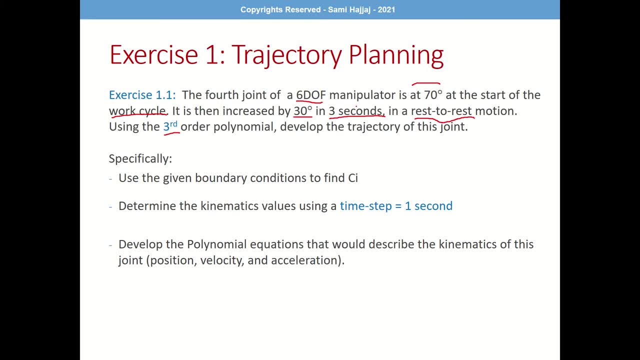 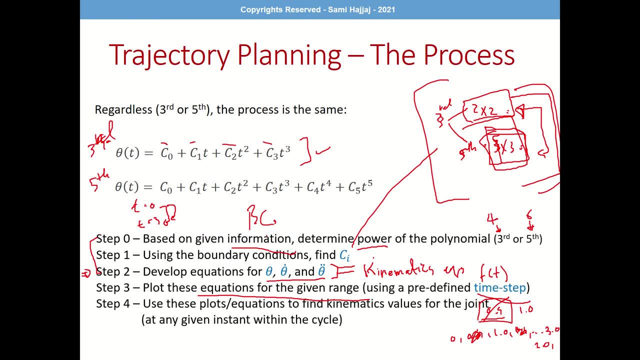 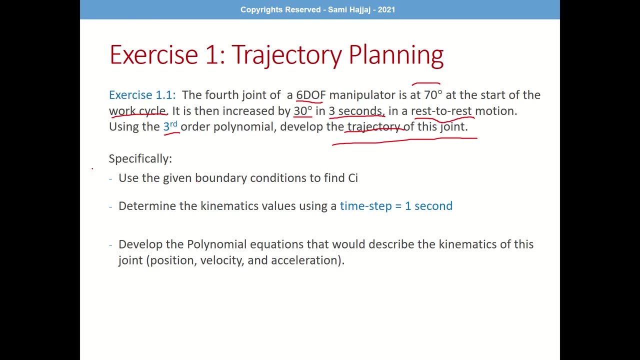 telling you what polynomial to use. develop the trajectory for this joint, straight away, right there. And when we say develop the trajectory means all of this, means find the equations, develop the formulas, plot and so on and so forth. So, But again, one again, because this is an exercise, so the question is: giving you even 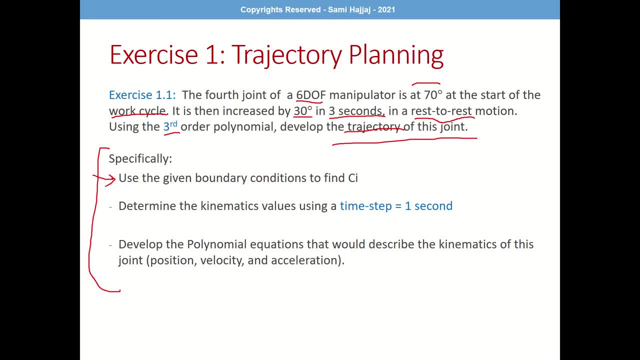 more specifics. Specifically develop, using the given boundary condition, find the coefficients or the constant values and then determine the kinematics values at a time using a time step of one second. So let's see. So it's from zero until for three seconds. 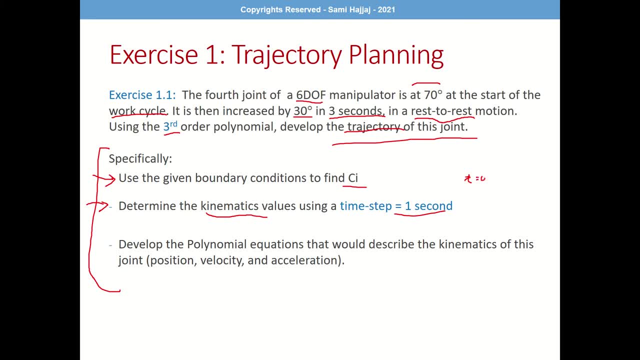 So you have, T is equal to zero. So T is equal to one because it's after one time step, And then the second time step would be zero. Okay, Sorry, Two here, Yep, And then finally T will be equal to three. 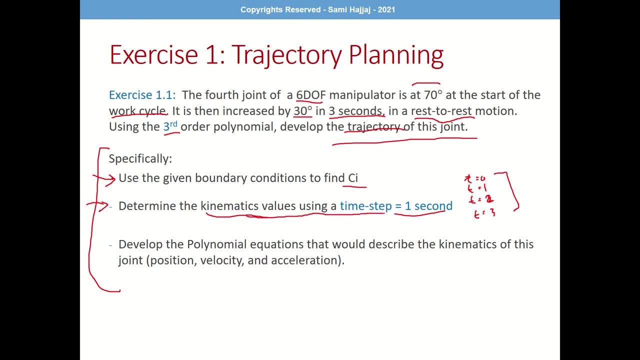 So these are the values. So when they say find the kinematics values using this time step basically means find the values of theta, theta dot and theta double dot at this time And repeat the process for all of these three values at all of these times. 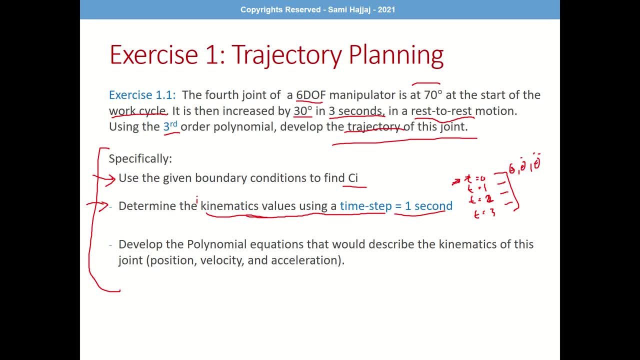 Okay. So that's essentially what the meaning of find the kinematic values using this time step. Then, once you have those nice values, then you can. the point of plus one is zero, Okay, So the point of plotting becomes straightforward. So once you have the values, then essentially you can simply just plot them as usual. 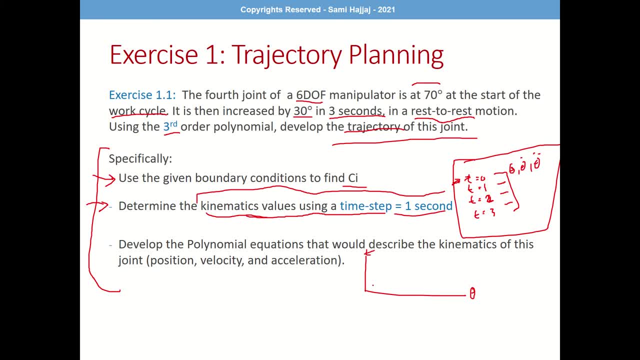 So let's say this was theta and this was time, So you have Sorry. Let's just say this is time and this is theta, very ugly, very big theta, right? So this will be zero one and this is two, and this is three, which is the starting, and 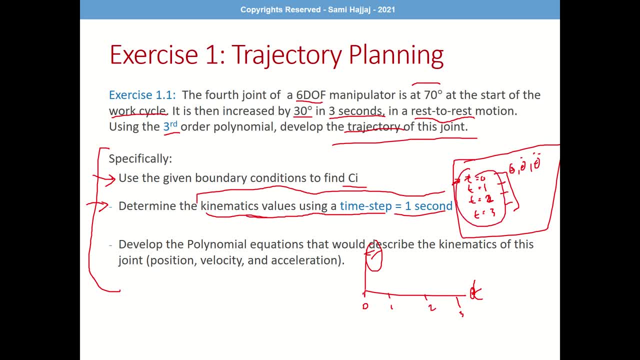 ending, And then you already have the values Remember from here. So it's just a matter of now plotting. So you have one value here, one value here, one value here, and then you can just use by hand. So that would be the plot for position. 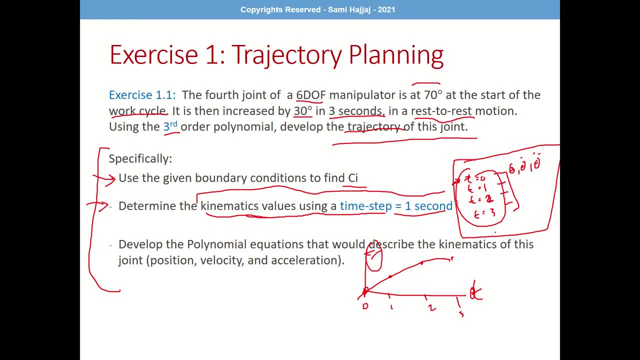 Similarly, the process is repeated for acceleration and velocity, and then you will have the drawings on you or the plottings for velocity and acceleration. So what about jerk, which is the derivative of acceleration? No, we don't need it. 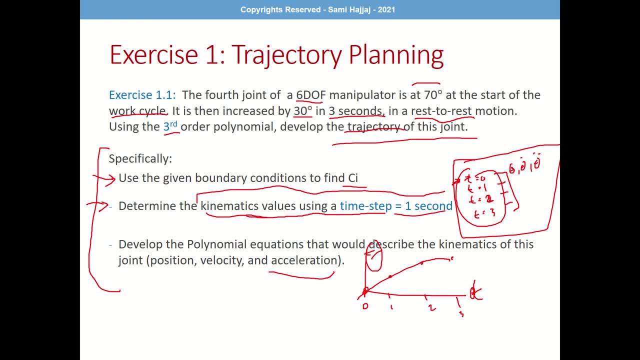 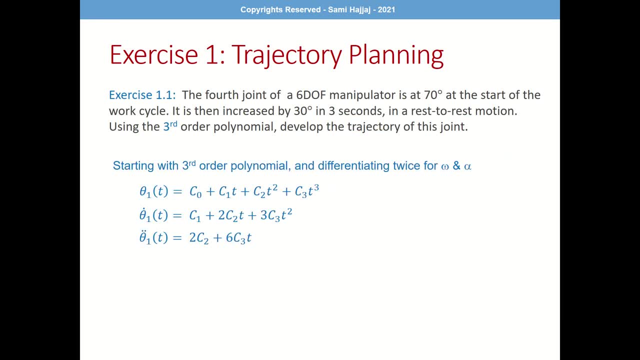 For robotics, or at least for now we don't need it. But if we did need it, we just have to differentiate the acceleration equation and repeat the process. But for now we don't need it. So now, here we are. 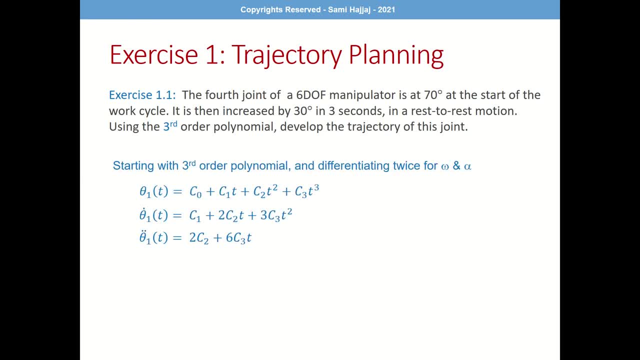 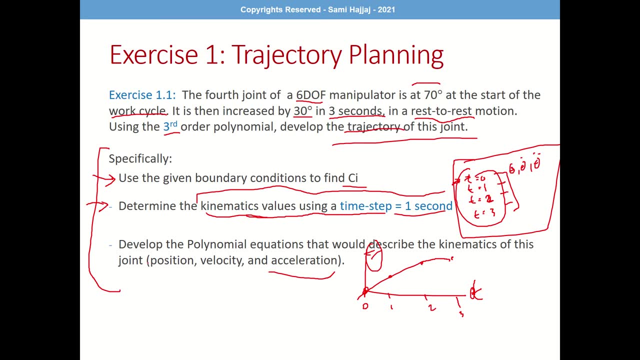 So essentially, oh wait, sorry, moving forward too fast. So this is the question. okay, So now, how do you do it? So, once again, I will give you a moment, I'll give you a chance to pause this video and 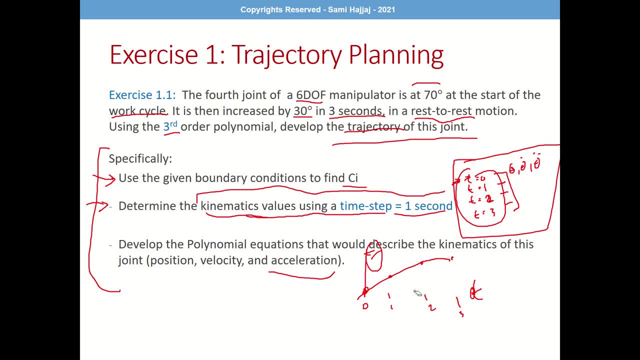 try and solve this question on your own using the memories that you have from Theory of Machine, or at least if you are a mechanical engineering student, because this video is meant for mechanical engineering students and you know what I'm talking about- you might want to refresh from your tom notes. 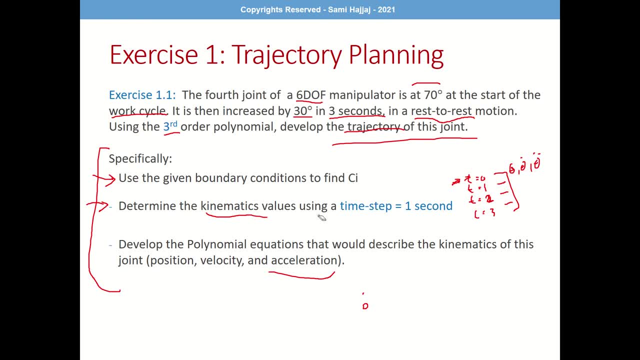 So, essentially, go ahead and pause this video and then solve and find the values and the trajectory for—based on the questions or based on the information given to you in the problem statement. By the time I finish cleaning this slide, I'm going to move on to the next one. 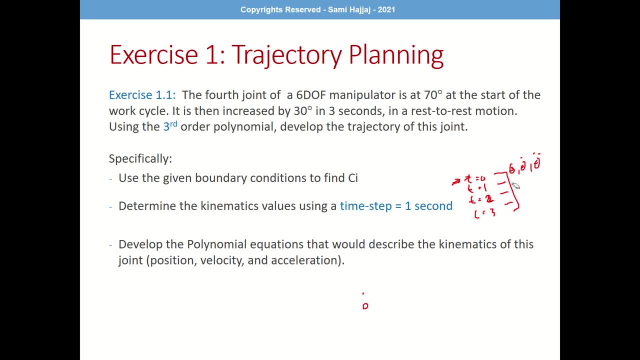 So if you want, you can pause right now and I'll give you a moment to fix it, to try to do with yourself. Jamilской generel. 안녕, It was Alif, it was Emile. It will be nice to talk a little bit. 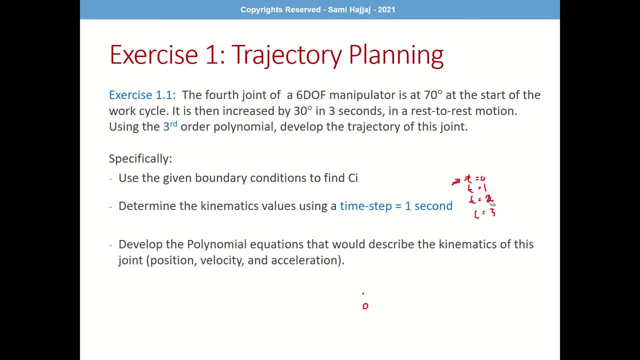 Bye, Jan Runyon. the next slide, which shows the solution. okay, this is too much, so i'm gonna move on now. okay, so now this is the solution. the very first step is that, since the question clearly told you to use, or simply, uh, made it easier for you to, to instructed you to use the third order polynomial, so straight. 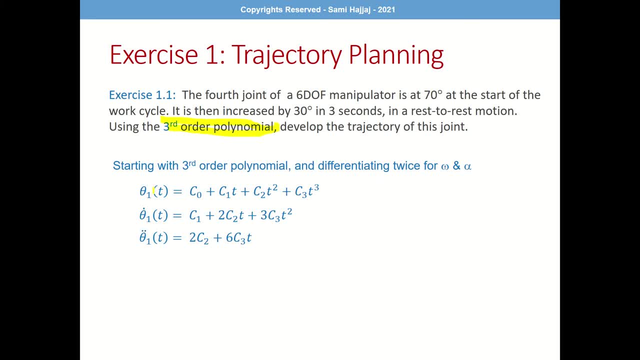 away. go ahead and use it. so the third order polynomial- actually this is supposed to be the question- said fourth joint. so you cannot use theta one because- but unfortunately because i copy pasted this from somewhere, so that's why, uh, i'm getting one here, but by right, this should be. 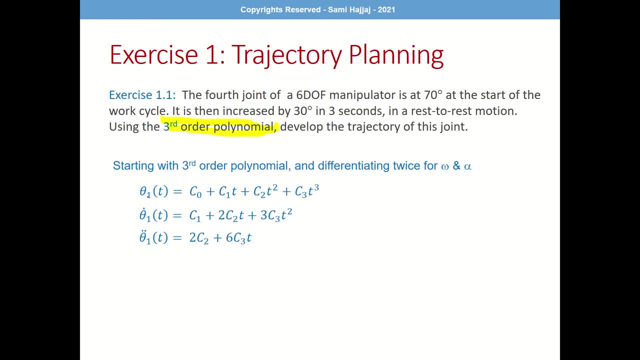 uh four, and this time we have to use four is because, uh, the question clearly says the fourth, the fourth joint. this should be four, uh, four and four. okay, so this is the value c one, and this is basically now the third order polynomial right here. this is now uh, third. 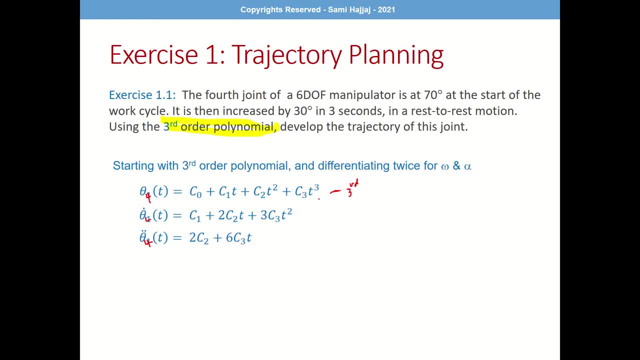 order, and if you take this equation and differentiate it with respect to time, you will get here. why? because, uh, that's the beauty of the, the polynomial equation, and that's why we are using it now, which is the simplicity of differentiation and integration as well. do this one more time and you get the equation for acceleration now, sir, did we need this bar? 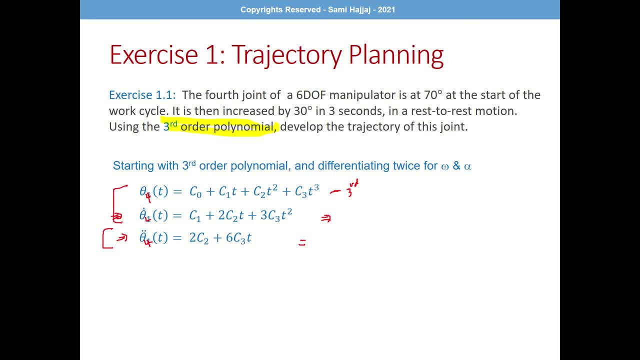 right here? no, we didn't, because the boundary condition is only for position and velocity. but if you want, you can just use this. you can just do it now. you might, might as well. i mean, okay, now that we've done the very first step, which is developing the equations for 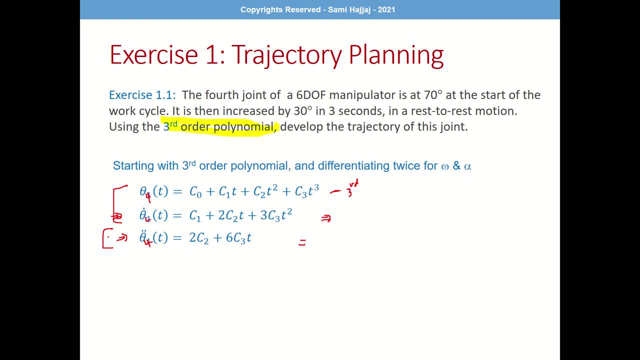 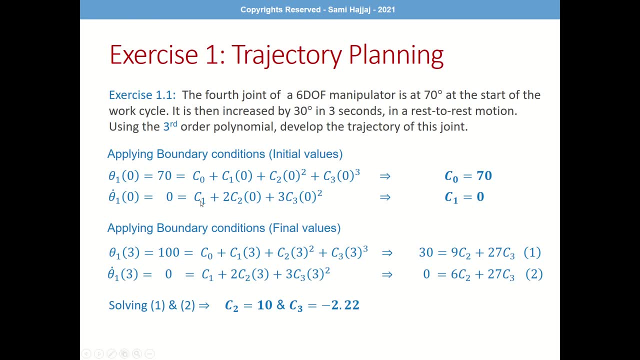 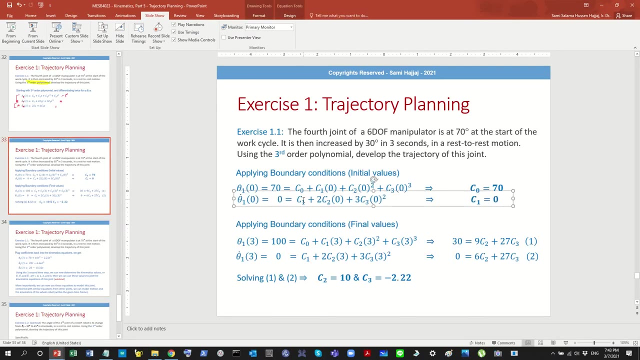 um, alpha, uh, i mean theta, alpha and omega. okay, what's next? next, we need to now apply the boundary condition and this right here, um, you know what? i'm gonna no keep, so i'm gonna go back here and i'm gonna eliminate, animate this part a little bit. so, yeah, so this one, this one, this one, and 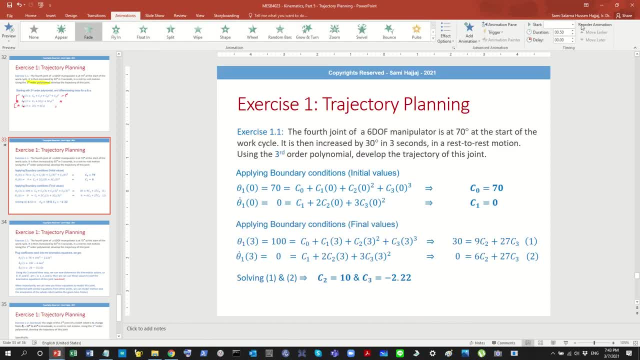 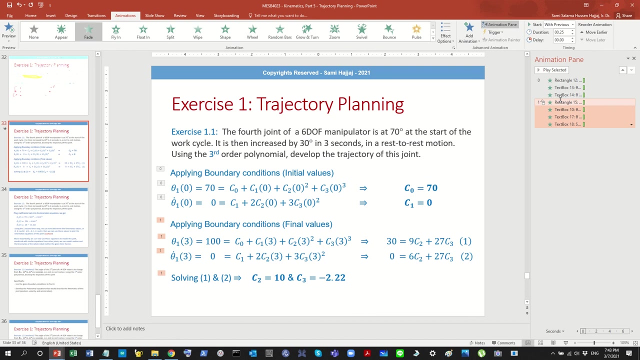 go to animation fade and make it fast, and also, uh, with previous and make it faster. yeah, and same thing for those guys. yeah, now you're watching how i animate my slides. uh, hopefully you learned something from this one as well. okay, so a bit of housekeeping here. so this one right here, i'm gonna. 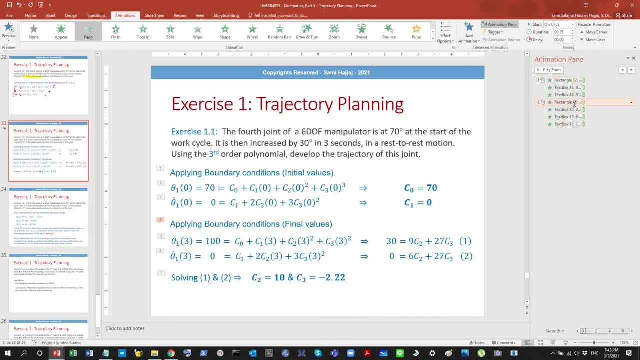 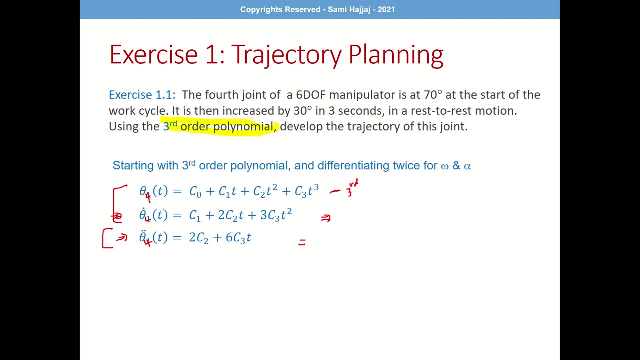 change it to one click right on, and this one right here's gonna be on click and the last one will be on click as well, and i think that's efficient. so let's go now to slideshow continue. so now, uh, now that we have developed the equations, what are we going to do with them? so now we need to solve the equations. 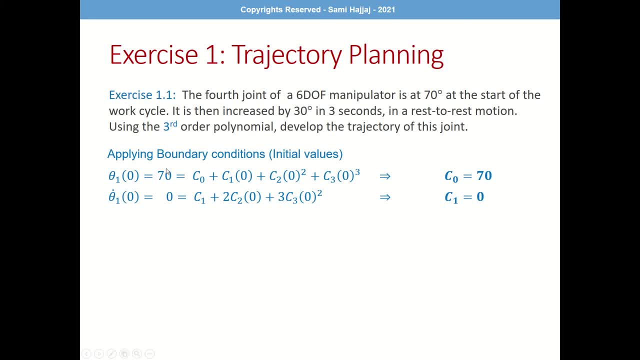 using the boundary conditions. so now we're going to begin with the very first parameter condition, which is we're going to apply it. we have four body conditions, which is um, position and acceleration, the starting value of theta, which is right here at 70, and then let me just switch on the thing. yeah, 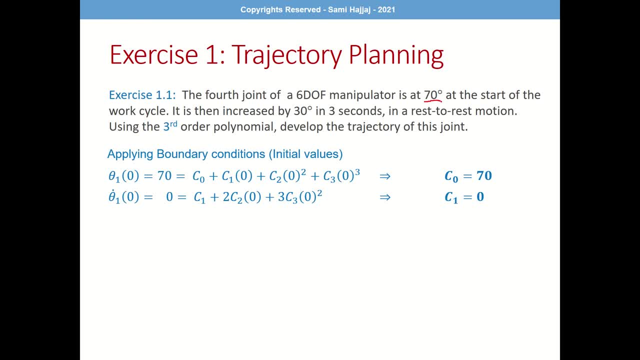 so we have the value for theta, the position value, which is 70, which is right here. this is what's going on at this point. but this statement right here says: is that the value of theta 4 at the start of the time or at or at the initial time, and that's exactly as stated in the 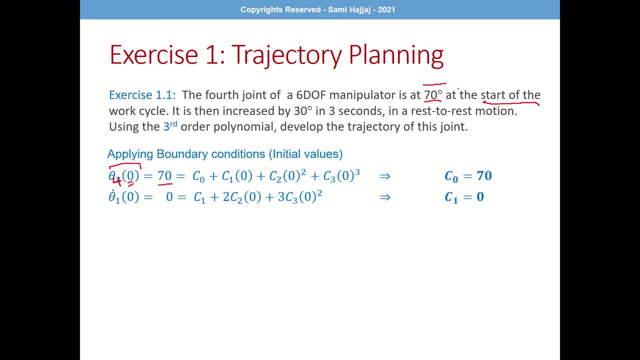 question at the start of the working cycle. the value of that angle is 70, so that's what we got here, but then we already know that the that also equal to this whole thing right here, this whole equation. so that's how we then we have this situation now. you have to remember that in order. 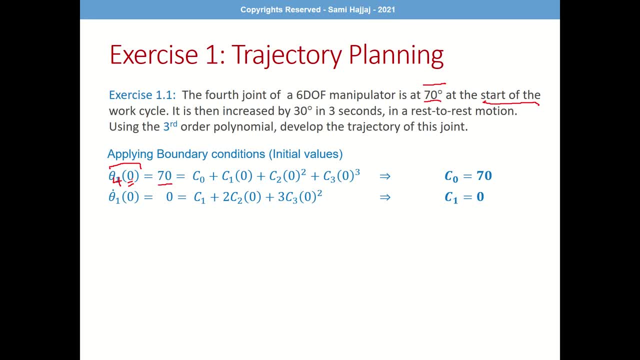 of you to get 70, the value of t is must equal to zero. so you can then use this equation: t, t, t. we just plug in the value of time at the start, which is time equal to zero. so we just simply plug in zero, zero, zero, and similarly here. so now we have the value for acceleration, and again, this is four. 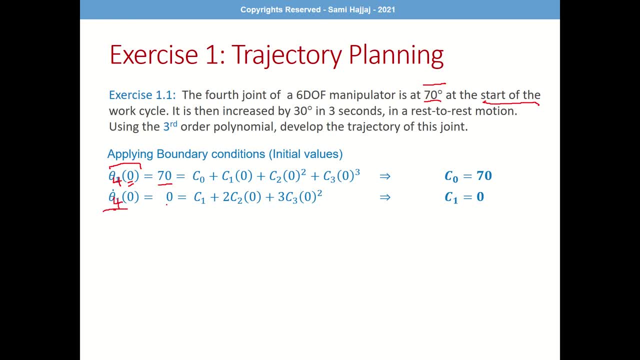 so in the beginning. we know that at the beginning of the velocity is zero. it's already given to us in the question. how did we do that? you should know it by now. but it's right here. it's from rest to rest, meaning at the start of the point the value of the velocity or the object was not moving, was? 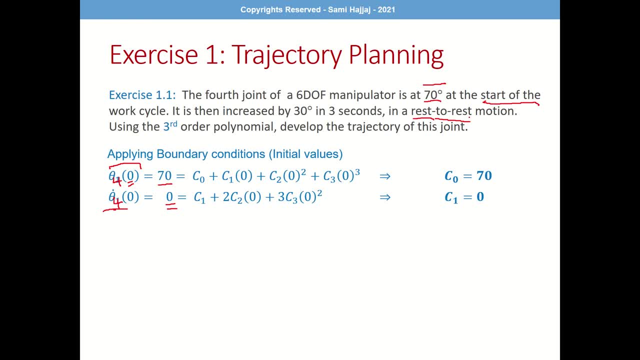 basically a constant, as it was resting. resting means it's not moving, in other words, velocity is the same as its constant right. so we let's continue to put in some indicated cosine function, as we do. we place the twodog on it and here we have the first two values, which is the initial 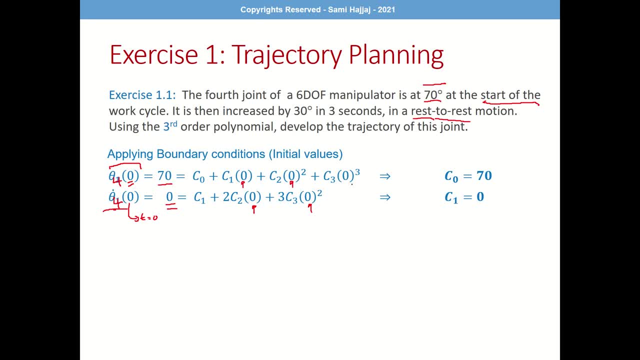 value, and then again we street and the derivative, we then put down the joint velocity and all the second-emetery part, fluid, chronic loss. that, that's three, is that is our final term here, regimented. so right here, that will be the final term, Cristo, here, since this will be the 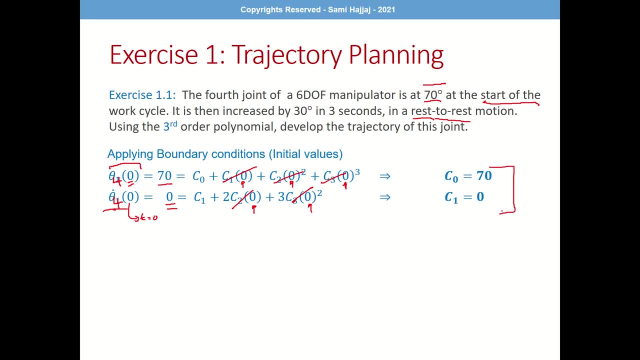 final term record for that will be the Iímность criterion, because it gives us this value which will have to leads to a profit straight away. the first two coefficients: c0 and c1. so henceforth, c1 is 0 and c0 is 70.. now you can. 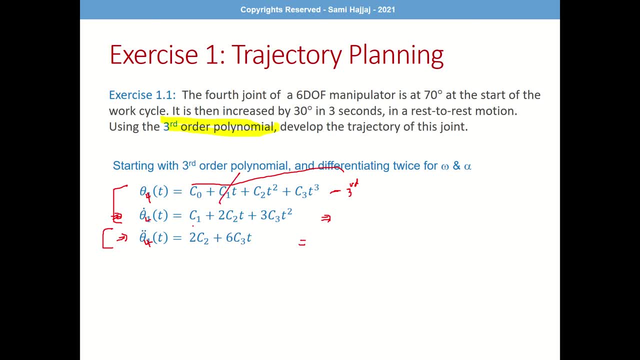 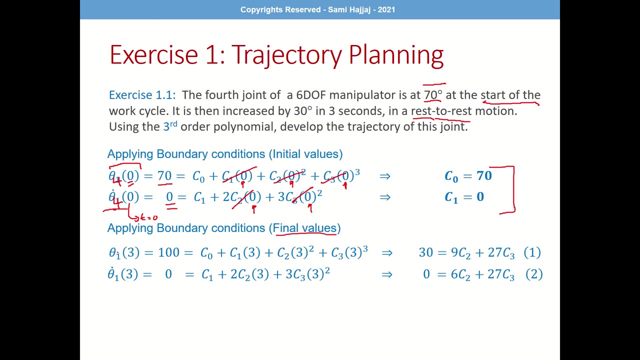 straight away go back here and straight away drop or throw away these two values, because c1 is zero. that actually simplifies the procedure later on. so, um, moving forward. so now apply the boundary conditions of on the final values right here. so again we do the same thing. um, again the position. 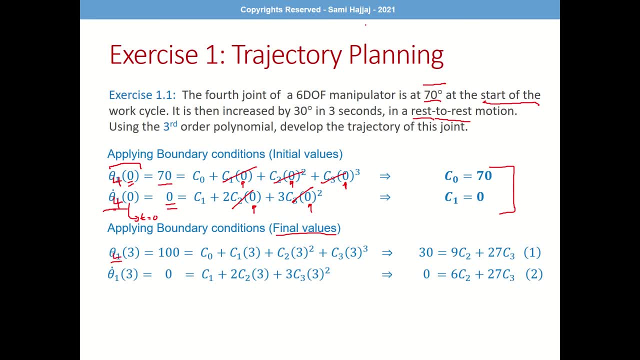 of theta 4, which is again given to us in the question, says: increased by 30 degrees, so it did not become 30, it's increased by 30, so the final value is 70, which is the starting value plus the increase, which is 30. so that's why we get 100 here. and then when does that happen, which is at: 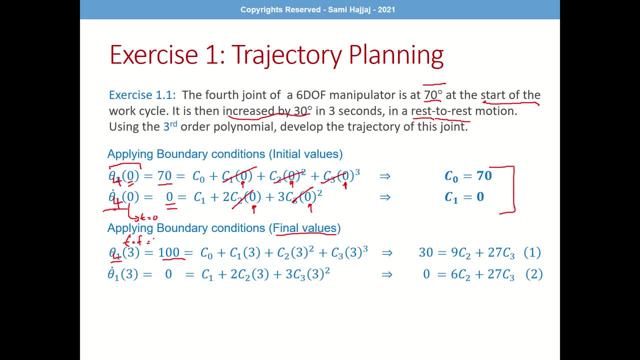 t is equal to final, okay, which is equal to three. sorry, so we take the value for three and we just plug it in here, so that will give us uh, three and three and three. it's all right. and the same thing here. so again. rest to rest means again at the end is also resting, so it means the velocity at the end is. 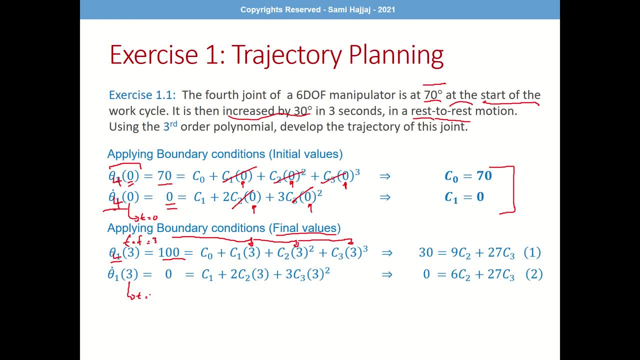 also zero, which also means that when the time is equal, final is also equal to zero. that means the position or, excuse me, the velocity was also equal to zero. so again, this is now: t is equal to three and this t is equal to three. so then, we need to now simplify this equation. at first glance, 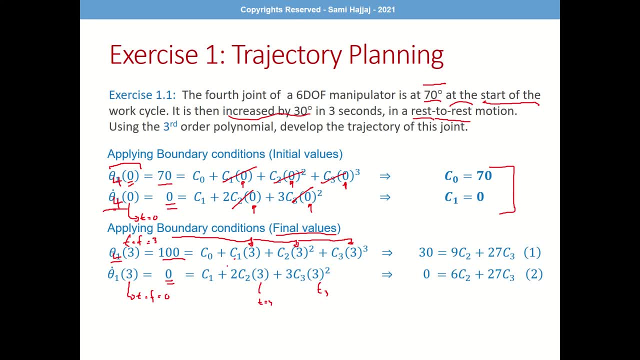 this looks complicated and scary, but you have to remember that c1 is actually zero from right here. you have to remember that. so then we can simplify this equation greatly by doing so. oh no, i think i made a typo. oh no, no, it's not a typo. so then, basically, now you have to remember also that 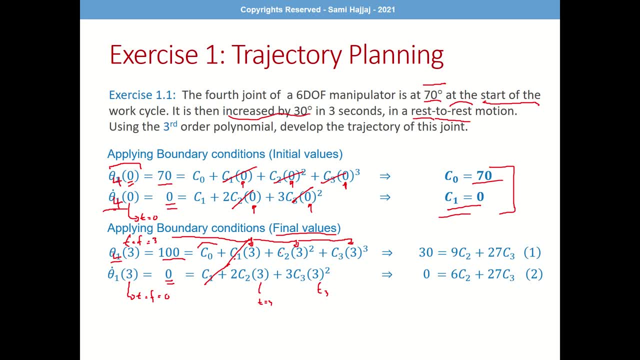 c0 is actually equal to 70, so you have to plug it into the equation. what i did here is that i simply did two steps in one. i put 70 here, so this is 70 and three to the power of two, that will be nine, and then three to the power. three will be 27, and then 70 goes to the other. 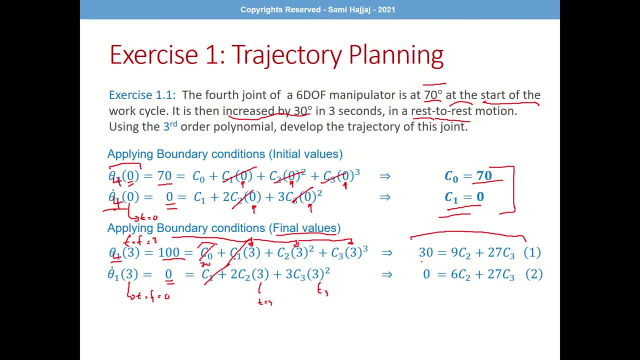 side. so 100 minus 70 gives us 30.. see here. so now this is what happened in equation. so now, after we clean up this equation a little bit, so this becomes equation number one, do the same thing for equation number two. you'd end up with this equation and now, this is now our same. 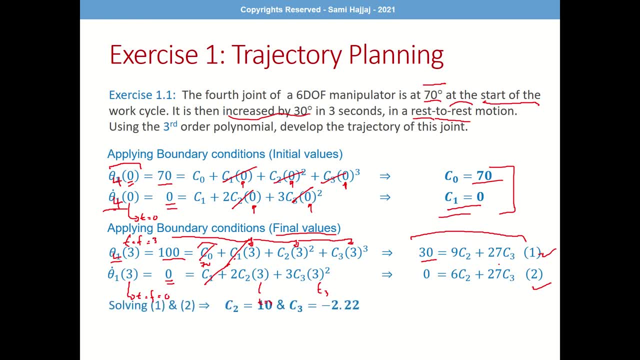 and this is our first and second. this is our first and second, and these are our first and second equation. this is what, then? this is what i meant by a two by two equation, two equations multiplied by two variables, in this case c2 and c3. we can then solve and find these two equations. 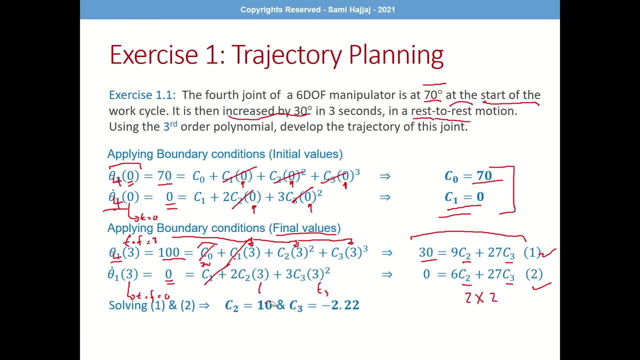 that will give us the values of c2 and c3. let me just clean up a little bit, so then. so then we can get: the values: of c2 is equal to 10, Yeah, C3 is equal to negative 2.2, and that gives us the coefficient. 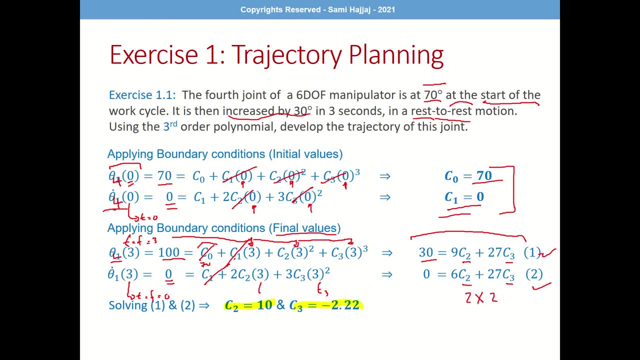 So this is basically what I meant by using the boundary condition to solve for coefficients. By the way, this is also a refresher, in case you forgot how to work with differential equations. So now moving on. now taking the coefficients that you have found. 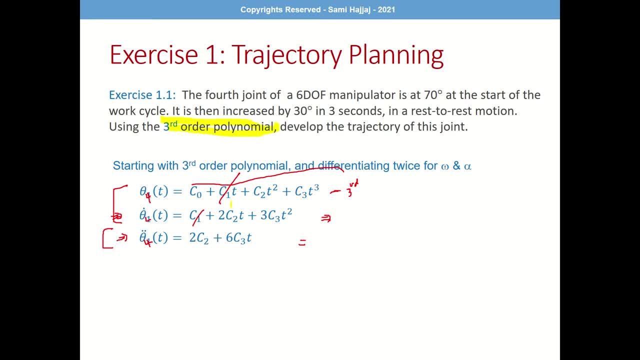 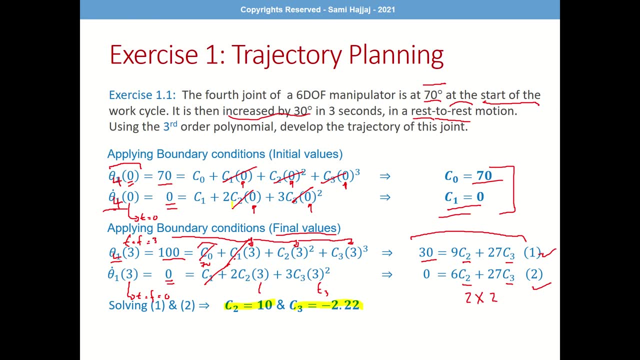 Now remember: the equations originally look like this, with all of C1,, C2, and all of the C values. Now that you have developed the values for coefficients or the value of the C's right, we just then plug them into the equations and then the equations will look like this: 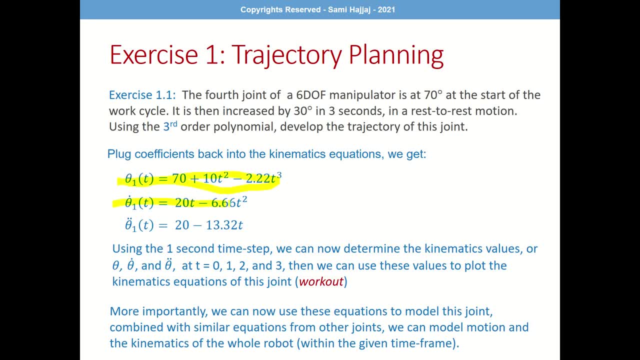 So, right here, these three sets of equations are now called the kinematics equations, Because right here, these are now the three equations that define the position, orientation- excuse me- the position- and velocity and acceleration of the joint number 4.. And again, let me make this quick correction here. 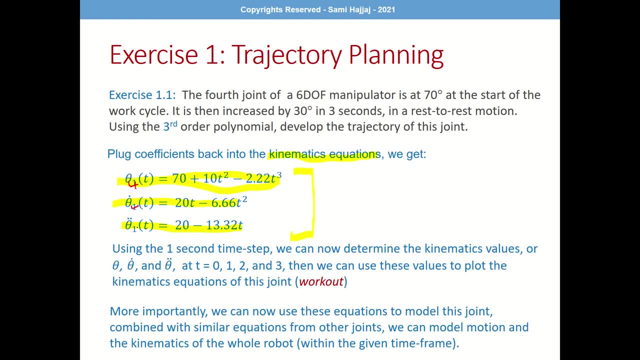 This is supposed to be 4, not 1.. This is a small typo. So then, essentially, these are the equations, or, if you want, you can call it theta, which is the position, and omega and alpha, but for joint number 4.. 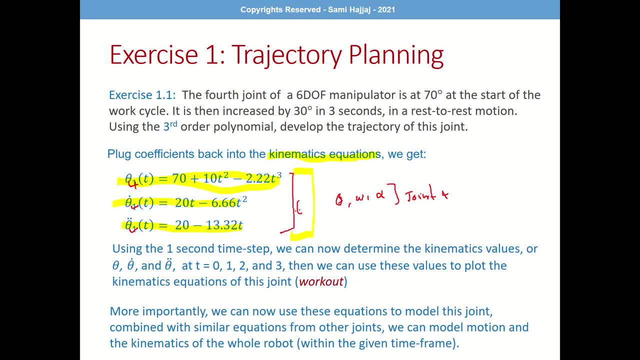 And, as you can see, it's defined as a function of time only, meaning the only variable we have now left is just the time. There's no other variable, no other coefficient, nothing. And then, from here on in, it's just a matter of substitution and plotting. 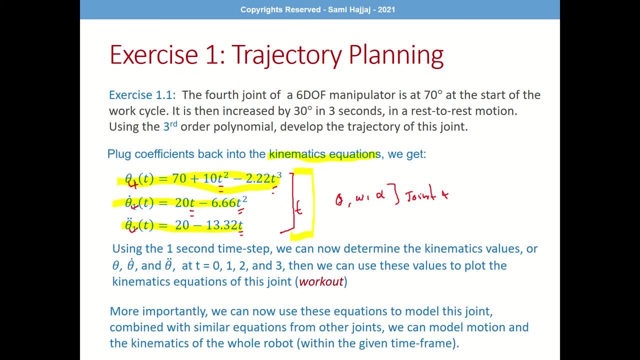 Really Basically based on the values, because the time step given to us was equal to 1, so here's the values of the time that correspond to us. We just plug them into this equation. So when t is equal to 0,, this is going to be a 0,. this is going to be a 0,, 0, 0,. 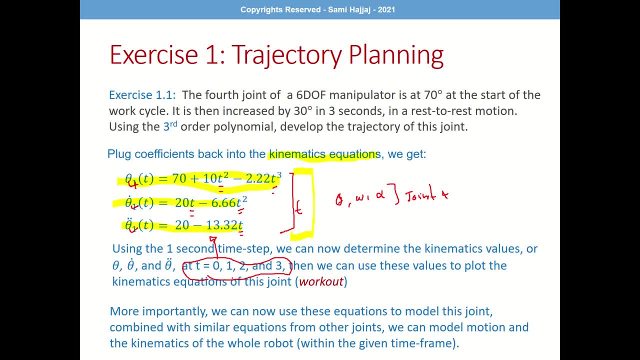 so we're going to end up with the initial values- You should verify them- And similarly for velocity and similarly for acceleration. By the way, if you actually plug, t is equal to 0 here. you're going to end up with the initial acceleration of 20, right from the beginning. 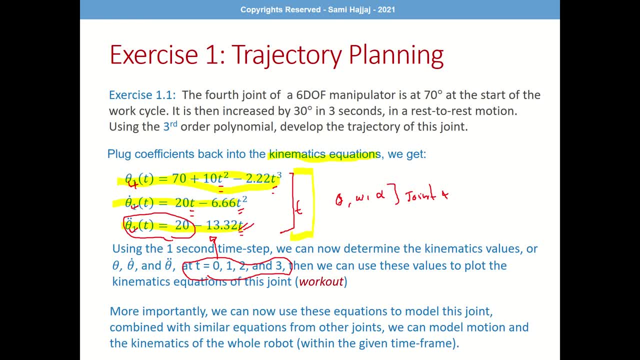 Acceleration straightaway is equal to 20.. So this could be good, this could not be. this could be good and this could be bad, And I will show you. you see, if you plot these diagrams right, I don't have diagrams in my slides, but I'm going to show you how the 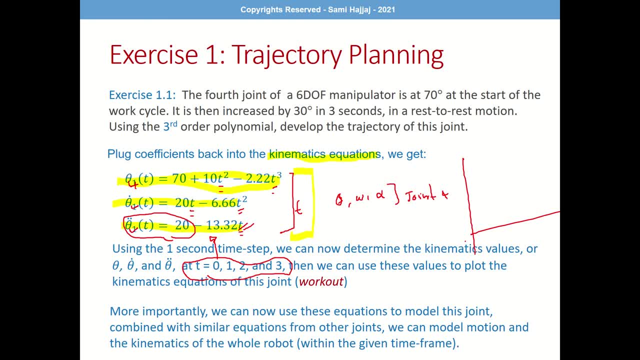 roughly the diagrams will look like: So the position will change from 70 to 100.. So, roughly speaking, this is going to look like: ignore that this is a 0, just say that this is 70 and this is 100. 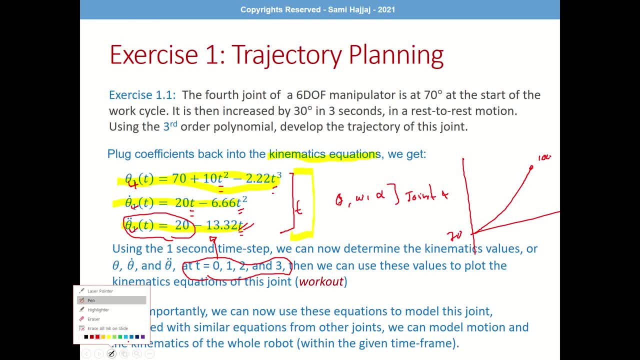 So this is the position diagram, And if I change the color a little bit, so now the angular, the velocity will change from 0 to 0, so that will look like this. So again, ignore the horizontal scale, whatever, but it will look like this. 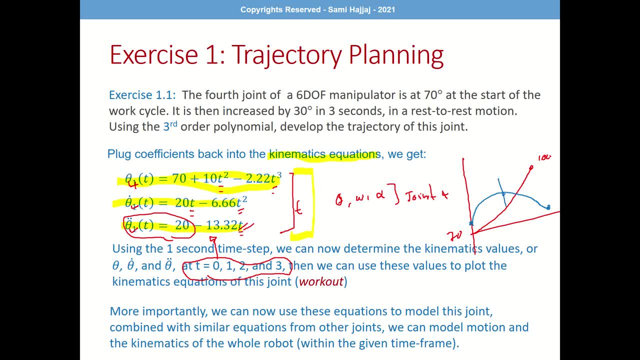 So you're going to end up from a 0 and end up with a 0, and then you know what? let me rewind a little bit, make this, yeah, let me just. I know for sure how the diagram will look like, so I'm going to plot it properly. 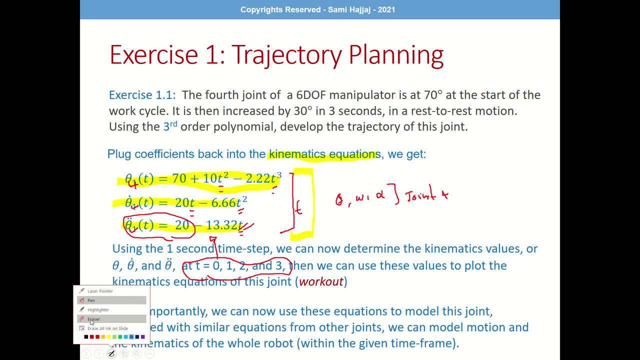 So, So, once again pen, and also the color of the pen is red. okay, right here. So let's say that this is now the time and this is now theta, omega and alpha. okay, So the value for theta is changing from 70 to 100. 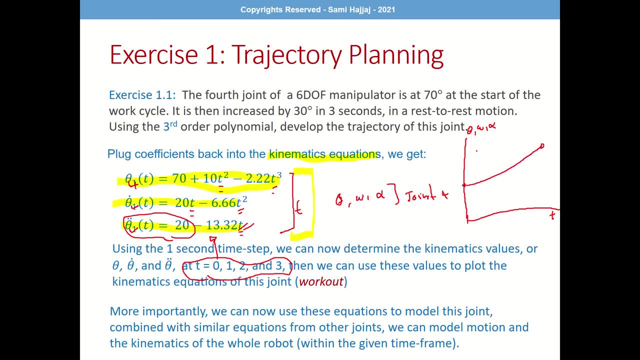 So let's just say that this is 70 and this is now 100,. okay, So this is now 70 and this is 100. And then omega will basically will be changing. Remember that omega, or the velocity, is rest to rest. 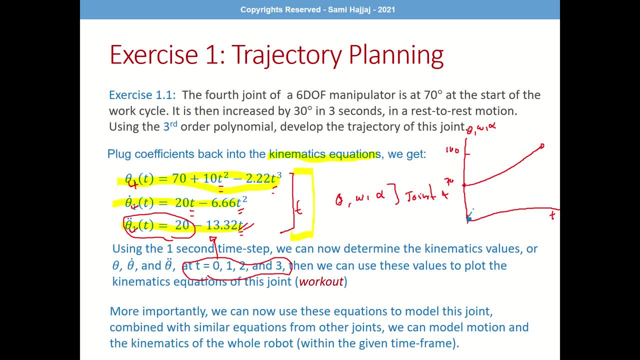 So you're going to end up with a 0 value right here. It's going to go to a maximum and then go to 0, 0 here again, right, But then take a look at what's going to happen to the acceleration. 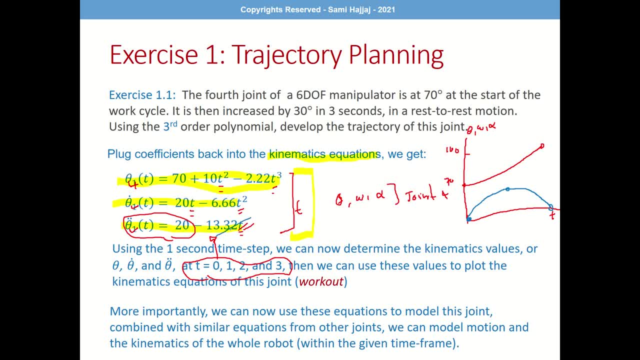 At t equal to 0,, which is right here- you're going to end up with the acceleration of equal to 20, right here or somewhere around here, And then at the end, it's going to end up with negative 20 at the end. 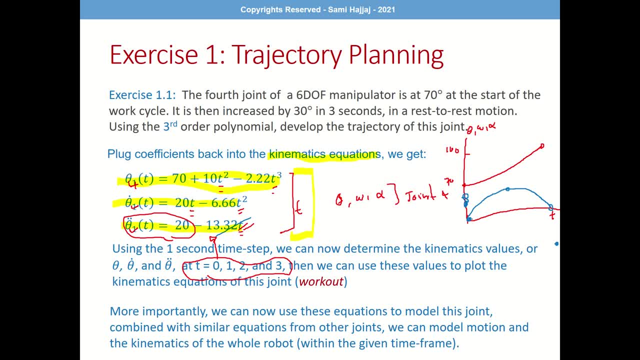 So, because it's accelerating here, as you can see that if you look at the velocity diagram and you can see that the velocity is increasing, is that right? So definitely we will have a positive acceleration here And then we're going to end up with 0 acceleration here. 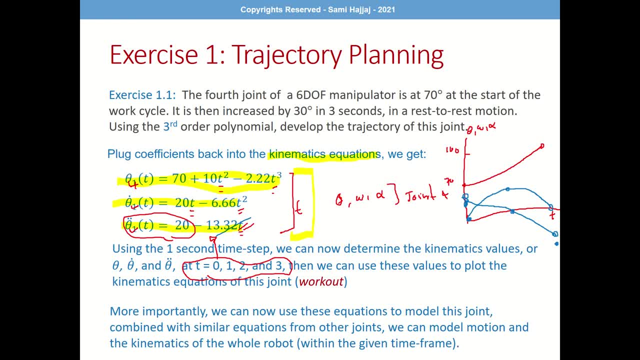 Then we're going to end up with negative acceleration because it's decelerating, as you can see from here. okay, Ignore this other point, All right. so what's the big deal? We can see that the cycle of this whole thing actually is now happens at this point. 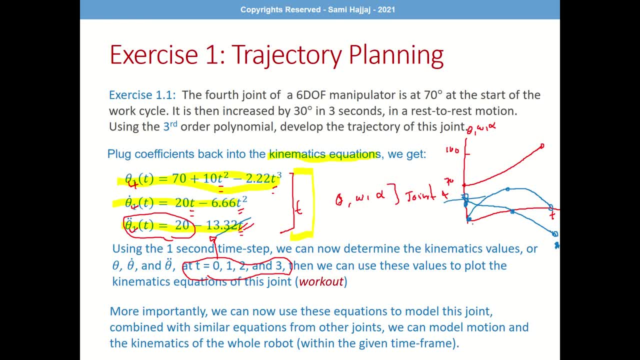 But what happens now is that when you start the cycle again- let's say, the robot motion is doing this in a cyclic behavior- we can end up with this behavior of the acceleration that looks like this: So now you have a jump or a sudden change in acceleration in 0 time. 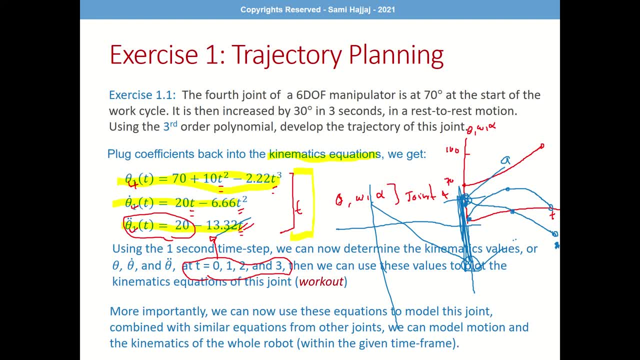 And you have to remember that this acceleration corresponds to a certain force and this acceleration corresponds to a certain force. So the change in acceleration will result in change in forces, in a very, very rapid change in forces That could result in a catastrophic failure to the actuator. 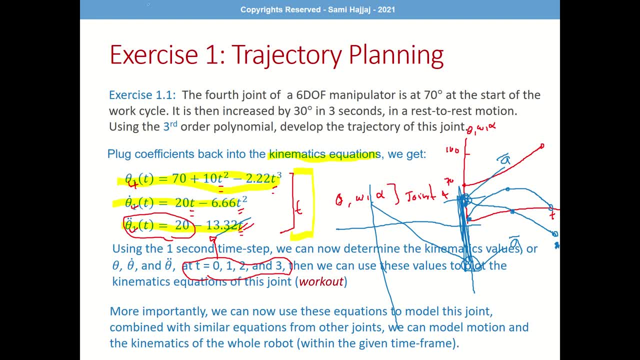 So that is why you know we're going to end up with 0.. Okay, So that's why sometimes it's not a good idea to do third-order polynomial, because the third-order polynomial does not consider what happens to the acceleration. So that is why, as an exercise, I want you to repeat the same exercise. 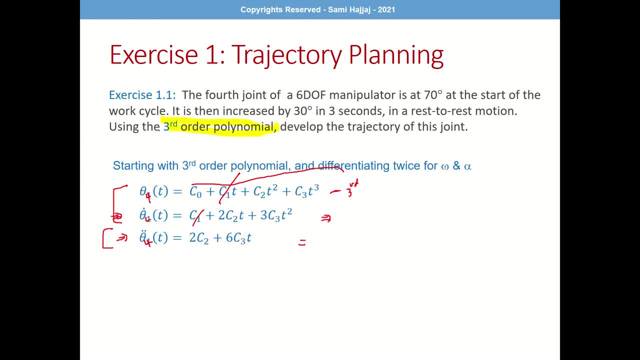 the same question right here. but rather than using third-order, use fifth-order and repeat the process yourself If you do want to do the manual work, which I suggest you do, but if you really want to do the labor work, simply use a program. 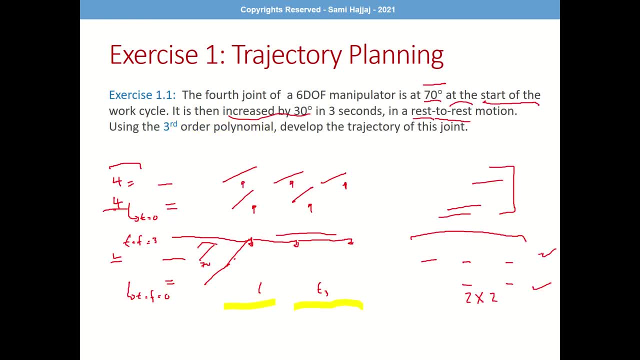 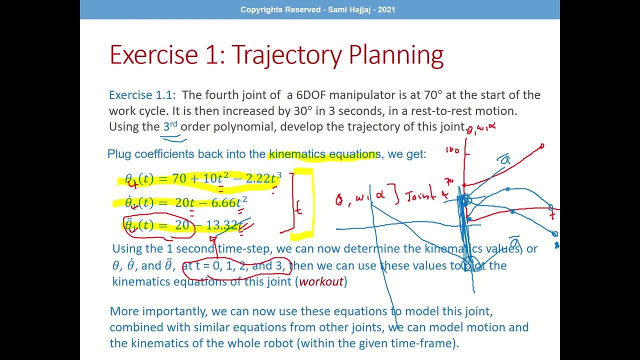 Write it in MATLAB or use it in your calculator or whatever, But then essentially see then the difference in the plots and you will see the difference or the impact of the third-order and the fourth-order. Finally, this is the last couple of slides now. 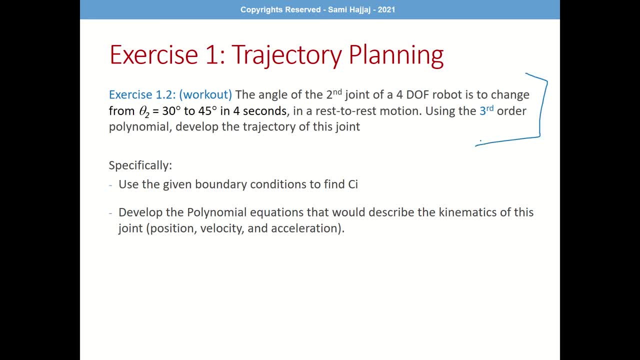 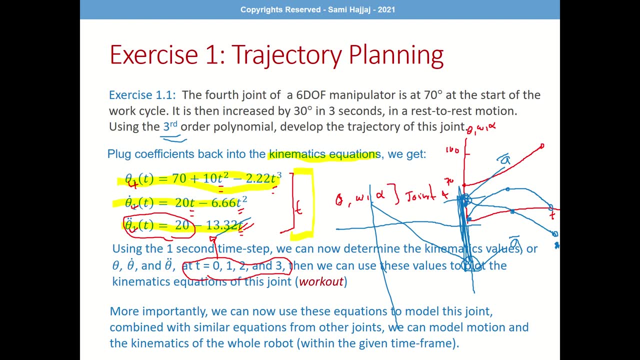 This is a different exercise, different workout. I suggest you do it twice, once for third-order and then fifth-order, And it's really it. It's just a different example, That's all. It's a different example. I suggest, with that solution this time. 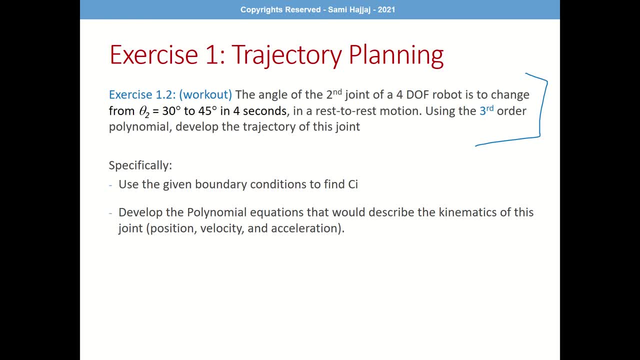 So I suggest that you do it directly using twice, Solve it Using third-order and then fifth-order, and then compare the difference in between them. Of course, when the object is resting, the acceleration must be also. The object is not moving, so it must have an acceleration of zero. 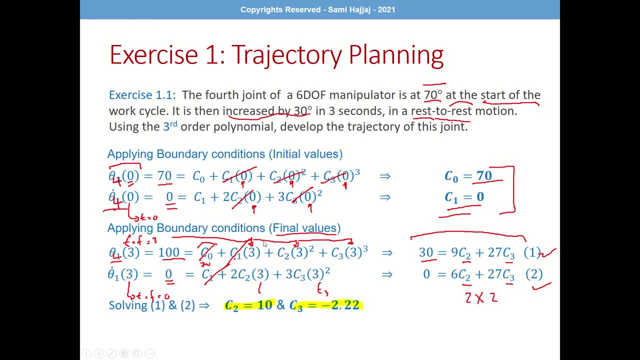 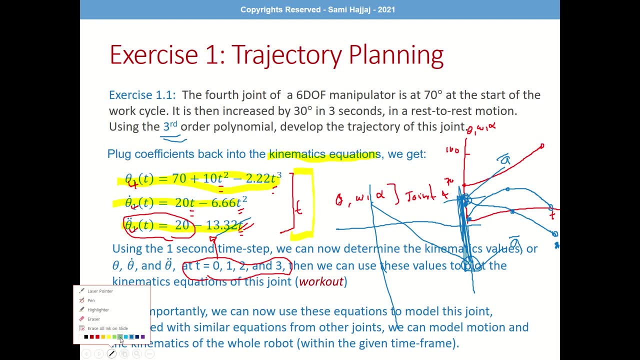 This could be something that actually made you think a little bit. You see What is it? Yeah, right here we said that the acceleration is The motion of the object is rest-to-rest. Is that right? We said that this is rest-to-rest means the object in the end is not even moving. 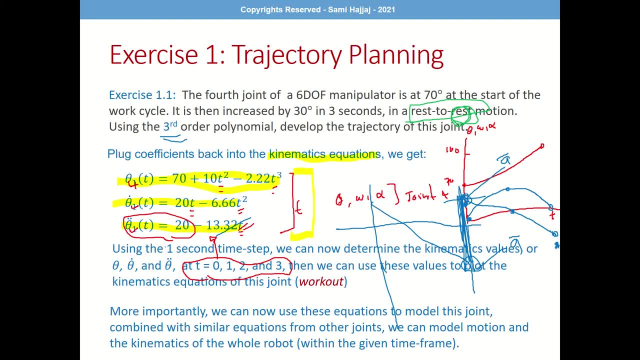 Or the robot joined. It's not moving, It's actually constant, Yet the acceleration in the end or the beginning are not constant, are not zero. You know what I mean. So that again gives us a little bit of problem. 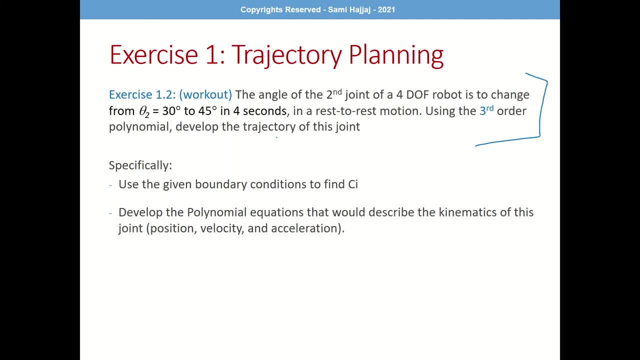 So that is why you should get, You should use the fifth-order polynomial, And I can tell you the fifth-order polynomial, the diagrams will be slightly different. You will end up with a situation like this. So this is the position 70 to 100,, as usual. 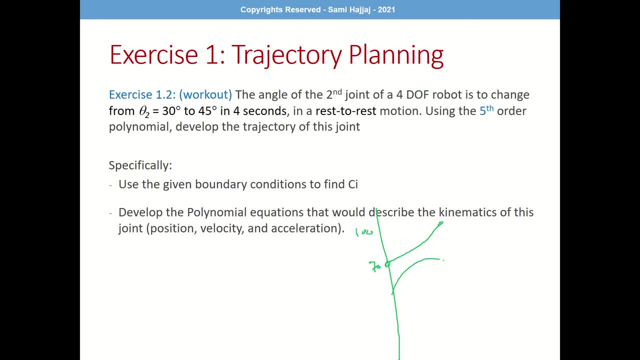 70 to 100.. The position or the velocity again will change as before: Right, But then the acceleration again. you should end up with a situation like this And the situation is also like that. So again you will have the velocity not going to be a very high step or sudden changes. 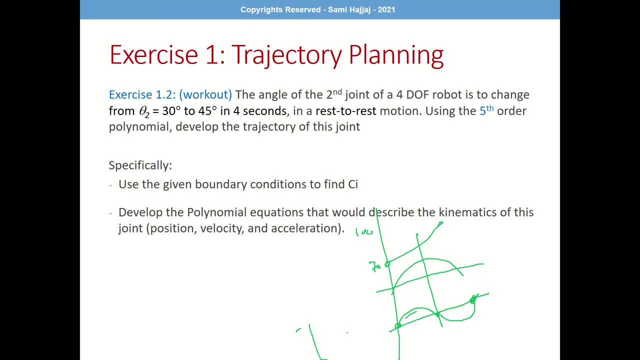 but then it will be cyclic. So even if, let's say, we repeat this motion in cycles, then the cycle will not be interrupted, so it should be no problem. So this is the impact of the fifth-order versus third-order. That's it. 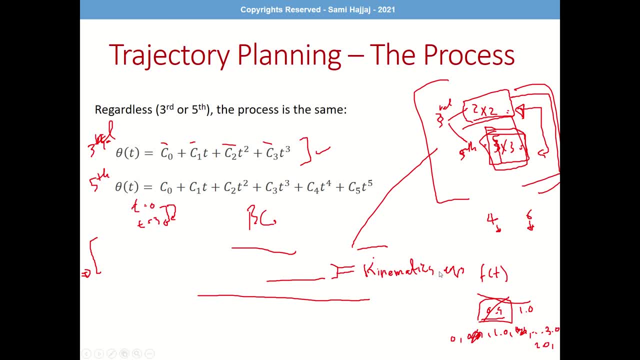 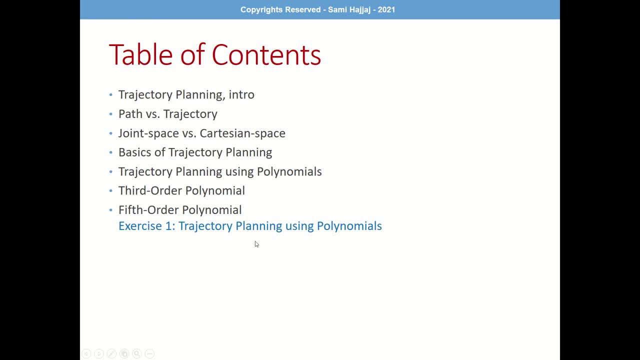 We have done. As I told you before, this session is relatively smaller compared to the others. We have essentially completed now the analysis on trajectory planning. One other thing: Like I said, this is only for one joint. We are just working with one individual joint. 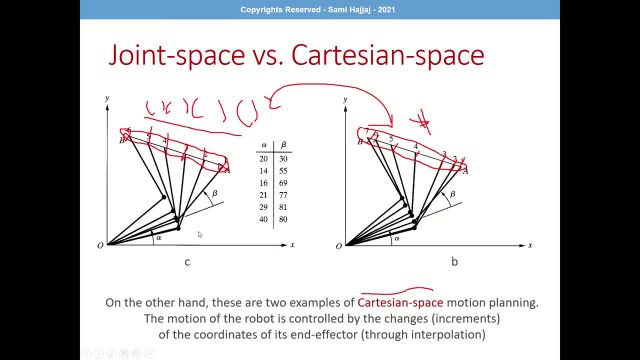 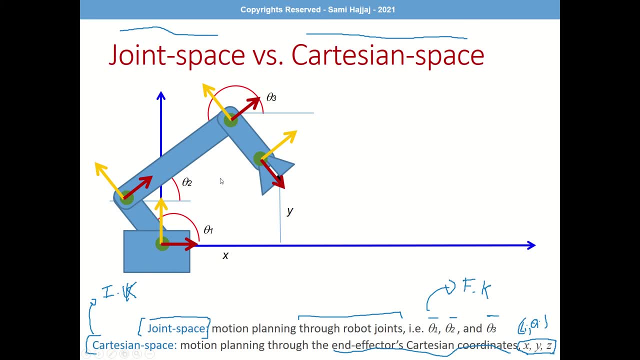 But in a real robot we will. After we finish the analysis on one joint, we will have to move on to the other joint. So basically we have to repeat the process, whether it's third-order or fifth-order for joint one joint, two joint, three, and so on. 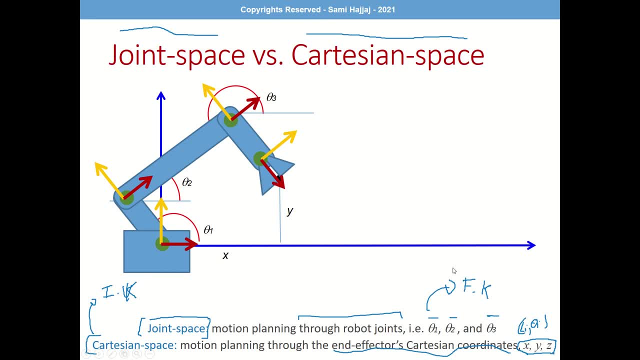 on until we develop a set of equations for each joint, and then we will then feed the controller all of these equations for each individual joint. but of course there is no point of repetition here. so if you know how to do this for one individual joint, then you can do the same thing for each. 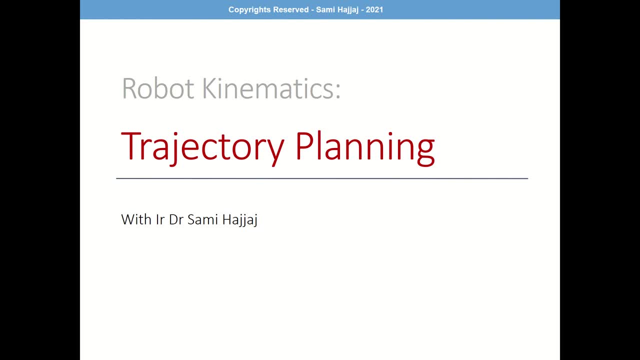 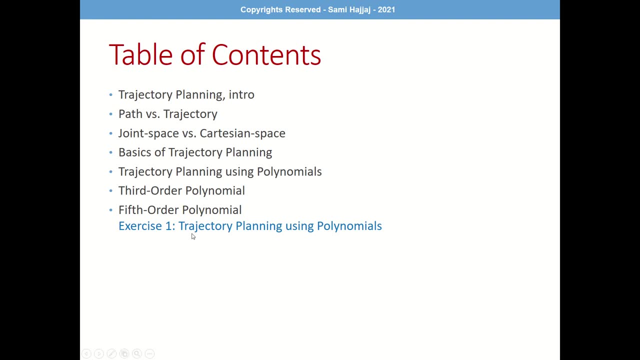 joint. so that is why we will stop right here and we will not do a robot-based trajectory analysis. we will simply stop at a single joint analysis. so, essentially, this is it. we have learned some, we have talked about some terminologies and then we we did some analysis familiarity with, if you. 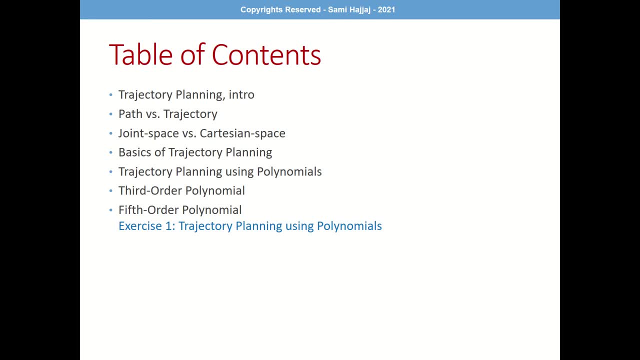 are already familiar with the theory of machine concept and cam chapters and that will helpful. if not, i will. you can then familiarize yourself with the polynomials in description in the link that i shared in the description, as well as through the example that i went through. 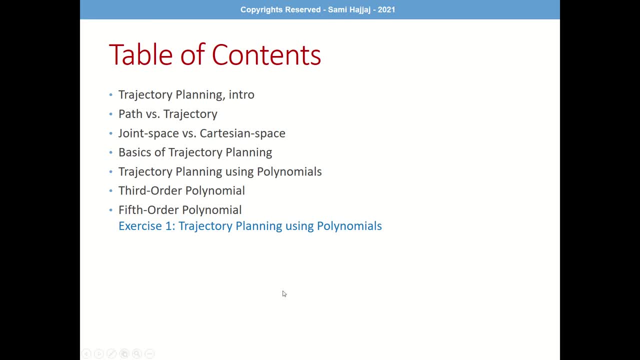 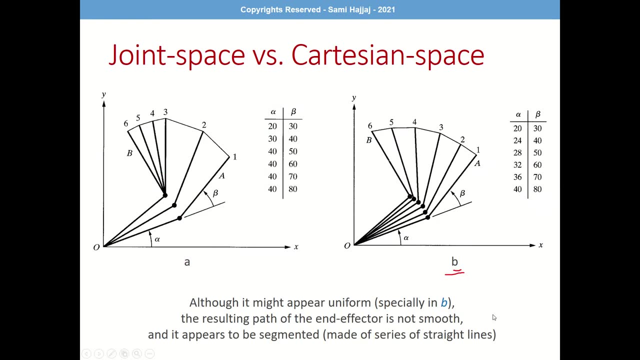 you and hopefully that will be useful for you. Now, what's the point of all of this? What was the purpose of developing all of these equations? I think I'm going to jump to the end for the answer to this one. So, once again, the purpose of developing those equations. 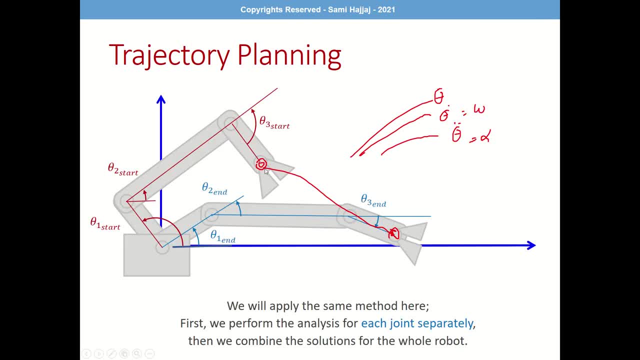 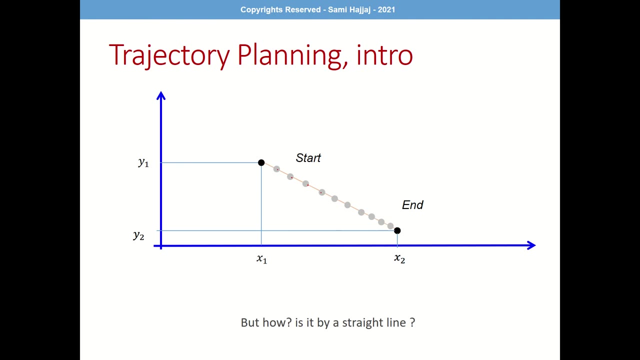 is that we will develop a formula or a function that defines the motion of the robot from one point to the other, while considering its velocity and acceleration of changes, So that then gives us the best. Remember, we were confused when we were moving from one point to another. 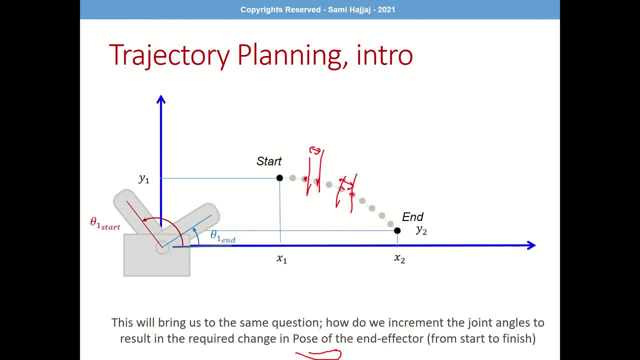 Should we use a straight line? Should we use a curve? Should we do a complicated curve? Or how do we go about it? And then the trajectory analysis simply answers this by providing us with a curve, directly curve, without having to know the individual points in between. 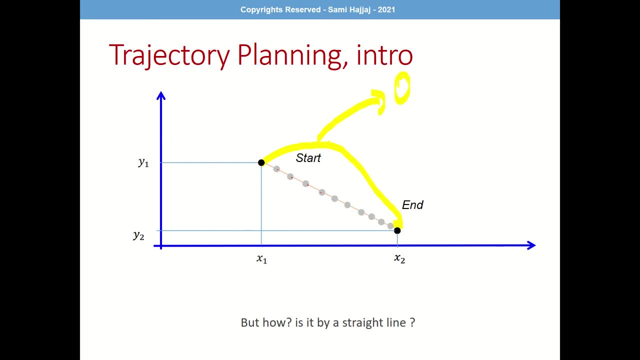 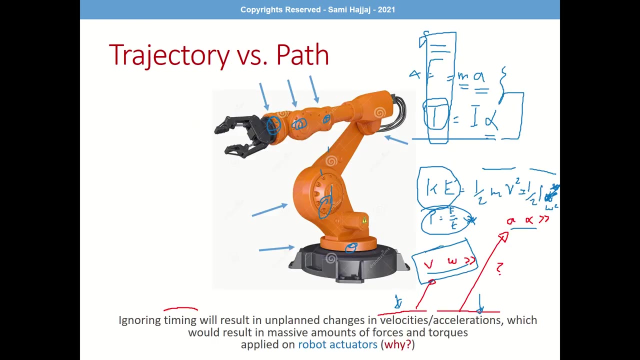 And not only that this curve provides us with a motion of the joint in terms of time, but it also gives us the same equation, or It also does the same thing, while considering velocity and accelerations as well. So that means that the motion will be timed. 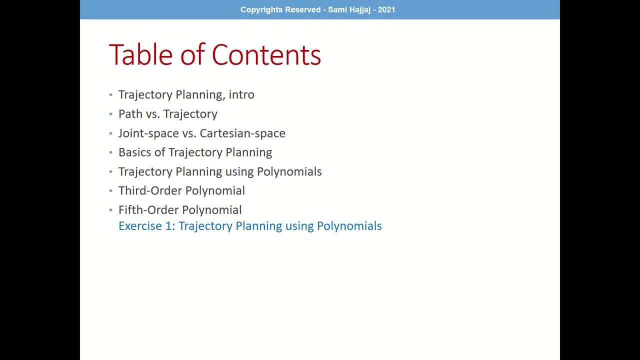 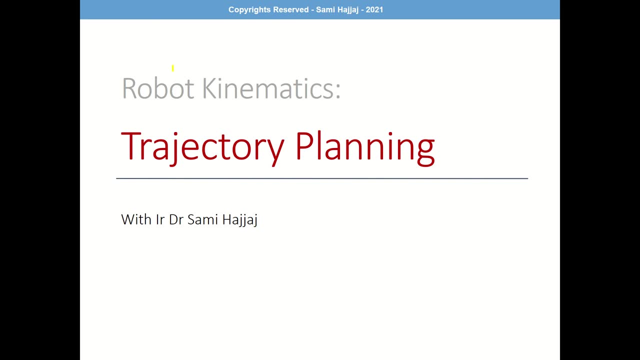 and therefore it will be within the safety requirements of the robot itself. Okay, so I hope that with this, we are now completed our kinematics in general. And if you remember, the very purpose of robot kinematics was actually to do this- Is that you have a robot and you would like to program it. 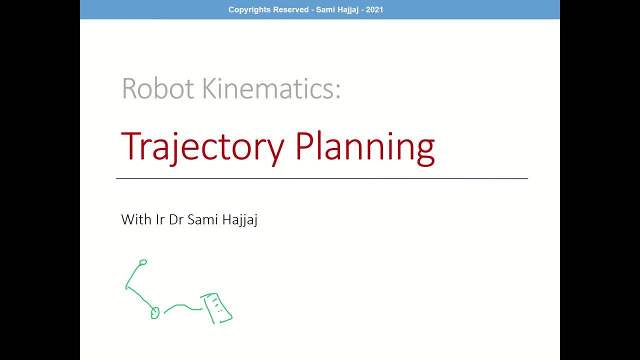 You would like. This robot is Connected to a controller and this controller is controlled or is you know- can be given instructions through a program, And in this program you will need to tell the controller what to do. So this controller would require some algorithms or some functions. 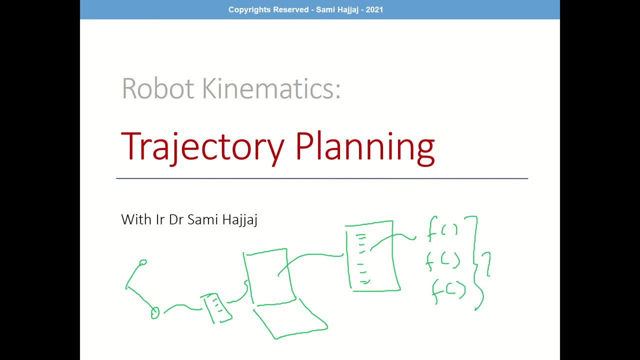 And those functions, how do we get them, was through kinematics, So this is now. hopefully now you will see the whole point of doing kinematics, Be it forward kinematics, inverse kinematics, as well as predictorial analysis. The procedure, essentially, is the same. 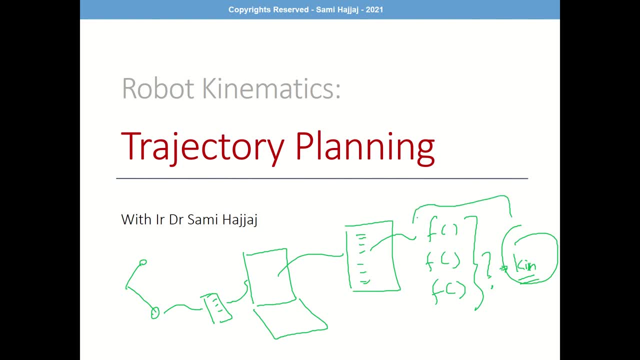 First, by doing the kinematics operation, we will develop the formulas. Once we develop the formulas, we can then write them in our program. Then in our program they can be then used to control the controller, which then results in the motion of the robot, to essentially to perform the motion that we want from the beginning. 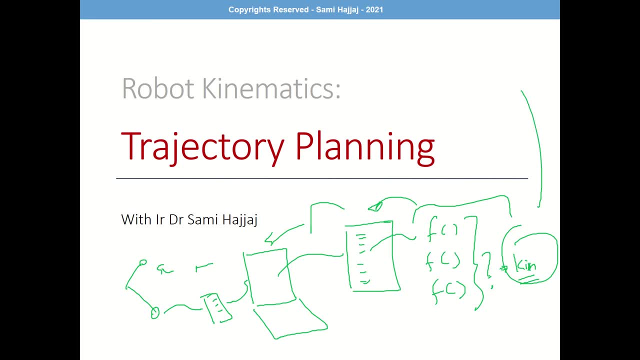 So of course, our kinematics will be based on requirements. So of course our kinematics will be based on requirements. So, of course, our kinematics will be based on requirements. Like certain changes, you want the robot to travel along a certain path. 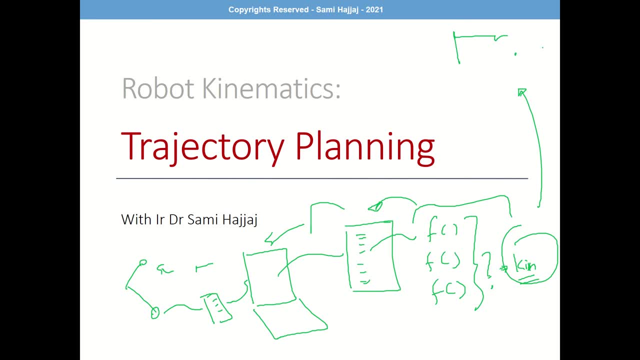 or you want the robot to move from a specific point to another. So these are the things you define. So first, after you define the motion itself, you then go to kinematics. Okay, this last part was ugly, So let me fix that one. 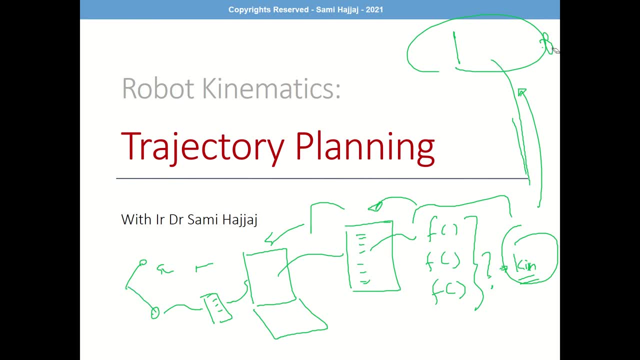 So essentially the complete sequence. hopefully now you can get the whole picture. So yeah, so we start from here. This is where you begin. You have an industrial robot that you would like the robot to do a certain motion. So you have the robot and it's right here. 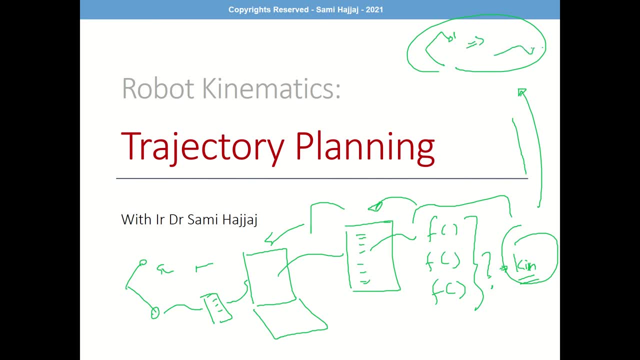 and you want it to move from this configuration to this configuration, for example, and you want the robot to travel from this configuration to the other, maybe back and forth, Let's say like in a sequence of motions. So you already define, you know the boundary condition. 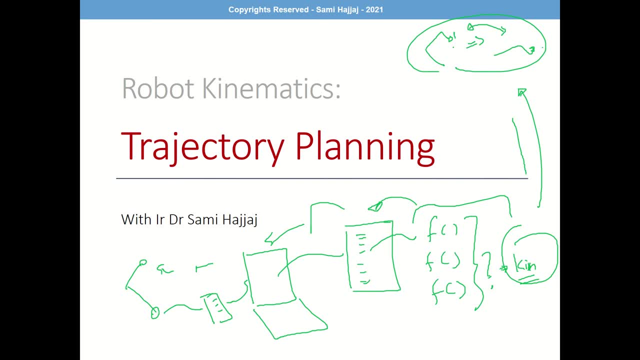 you define the position and orientation, all the pauses from the beginning, and the beginning and the start, And then you take this information and you feed it into your kinematics analysis. That will then, in turn, will provide you with the formulas that you will need in order. 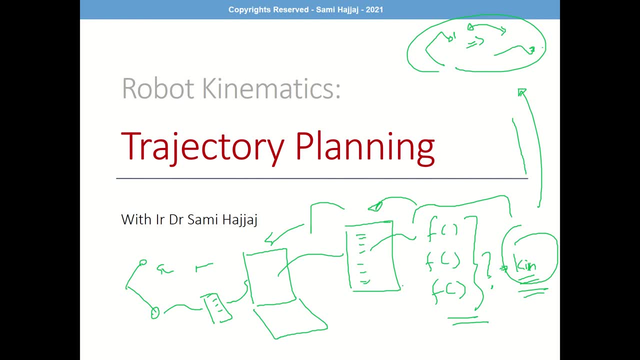 to those formulas that will govern the motion of the individual joints of the robot. These formulas in turn can be then fed into the program, And once they are in the program and then given the right values of the parameters, which once again given from here, then you can then use it to control the robot. 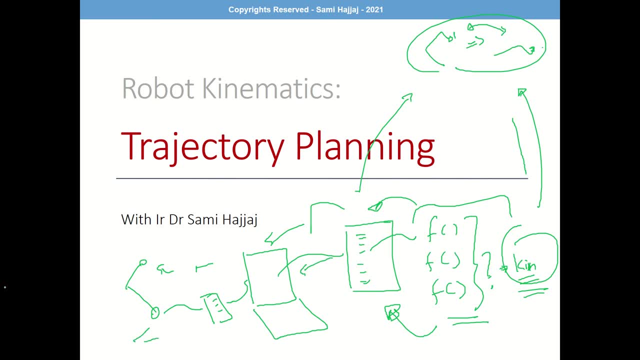 Then the robot can then perform the motion that you wanted it in the first place. So kinematics- in general speaking, kinematics are the key element that is missing for between what you want the robot to do and then the robot actually doing it. 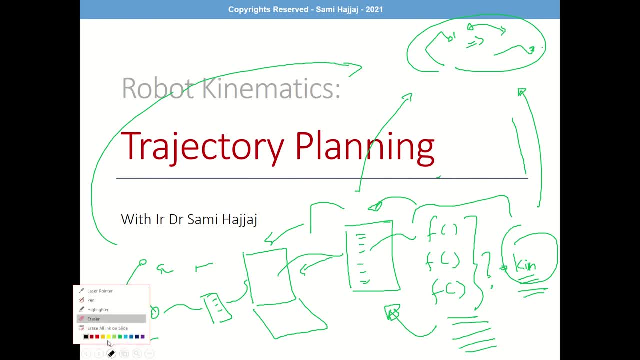 So hopefully by now you get the whole picture into what robot kinematics is and its purpose and why do we use it. It's extensive- it's nearly five weeks- but then we needed to go through this whole process to understand how it works. 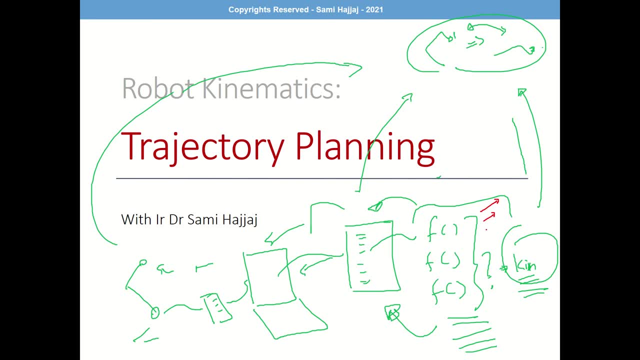 Again the robot frame matrix Transformations, forward kinematics, inverse kinematics and then trajectory analysis. They were all part of one unit called kinematics. Of course, in this particular course we also missed some elements out, like the DH approach. 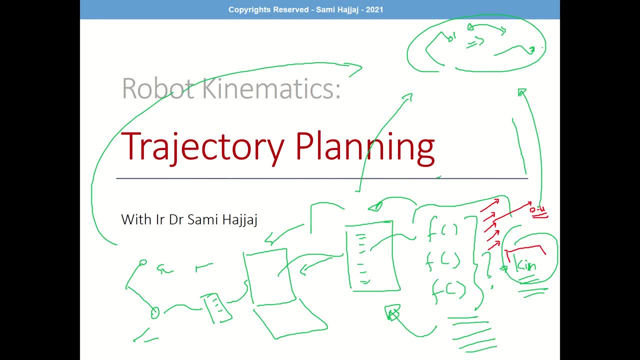 We did not really do it. So as of now, if you're in a course, you are limited to a specific number of robots. But if you are interested, then wait for my video on the DH, which I will do later on. 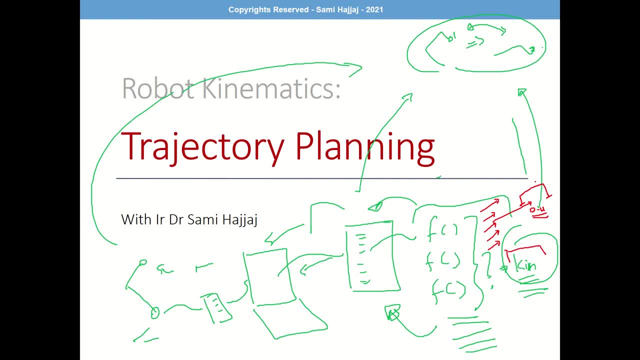 but it's not part of the syllabus But it's for your general purposes only. But if you learn the DH approach then you can do any customized industrial robot And the reason why we did not include it in the course is because the chances of you working. 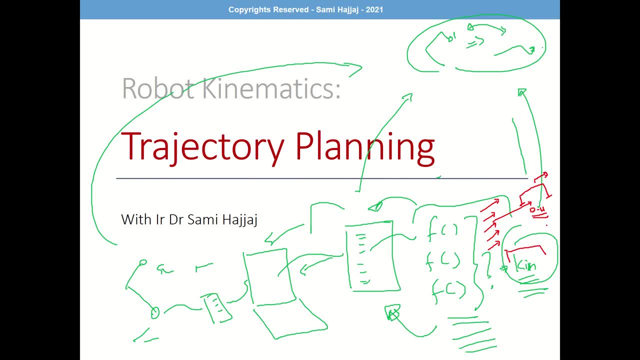 with a customized industrial robot are very slim. Most of the time, your company will buy one of the industrial robots or one of the planar robots that we talked about, So that is why the chances of you doing a customary or customized analysis are very slim. 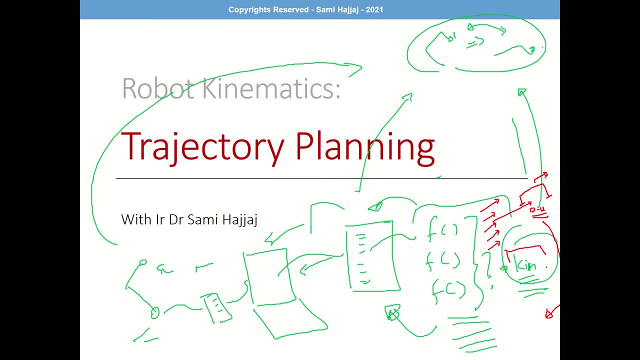 unless you are designing the robot yourself. The chances of you working with or designing the robot yourself right after graduation are very slim, So that's why I wanted you to focus only- or in the beginning at least- on standard robots like Cartesian, Spherical and Cylindrical, and then, of course, the planar robots. 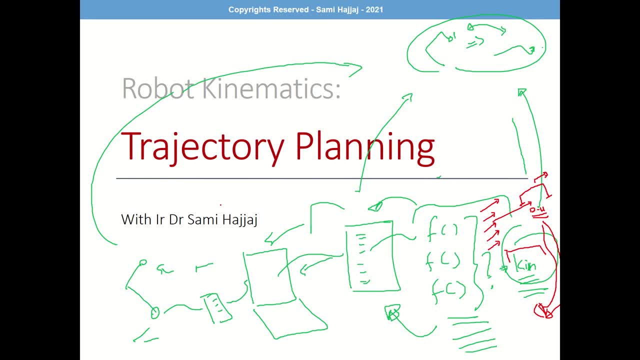 Okay, so with this we are done with kinematics. Starting next week, I think, we're going to have the test and then followed by the break, And then after that, we're going to start to focus on robot control. So I'll see you in the later sessions, in the next video. So thank you and take care.